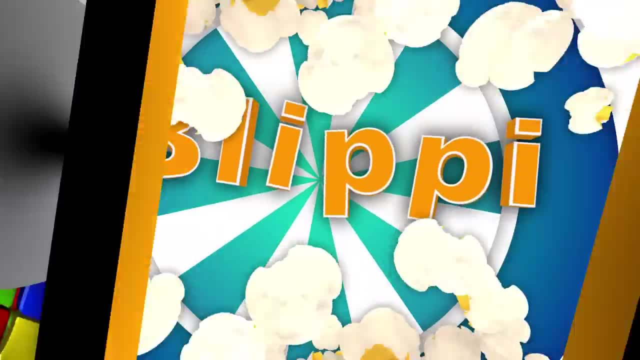 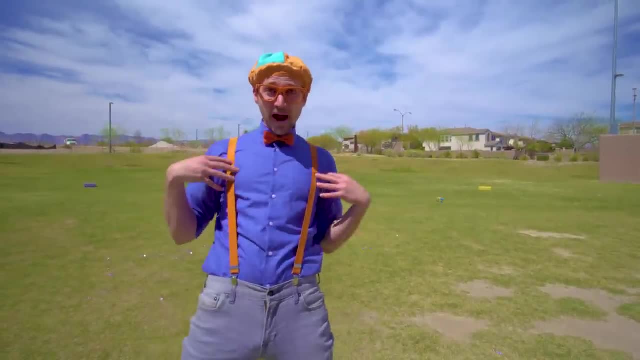 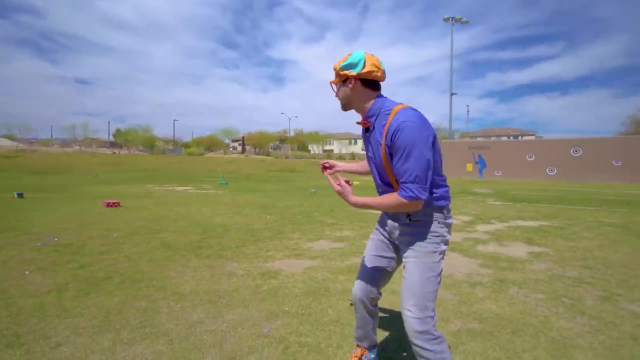 So much to learn about. It'll make you want to shout: Blippi, Whoa. Hey, My name's Blippi and look at what's behind me. Whoa, There's a lot of colorful boxes back there And it looks like there's ten boxes. 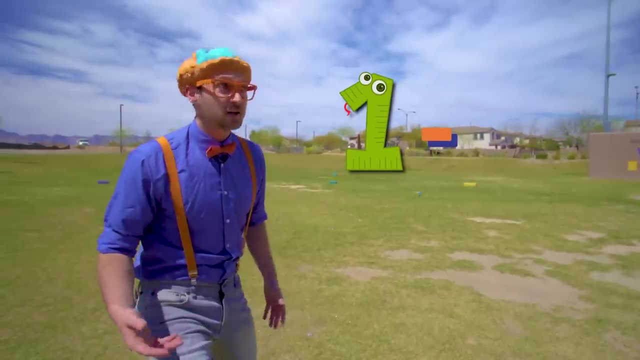 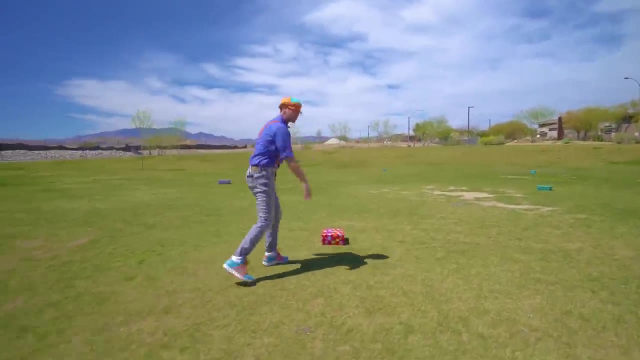 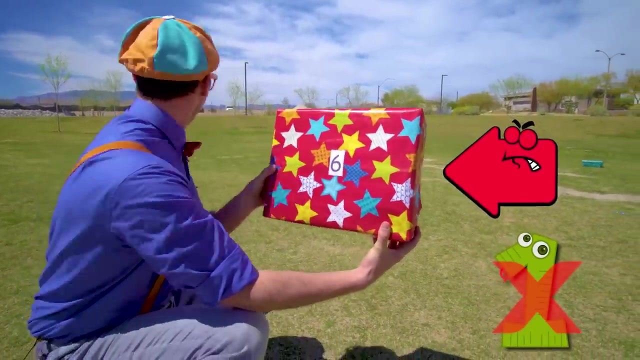 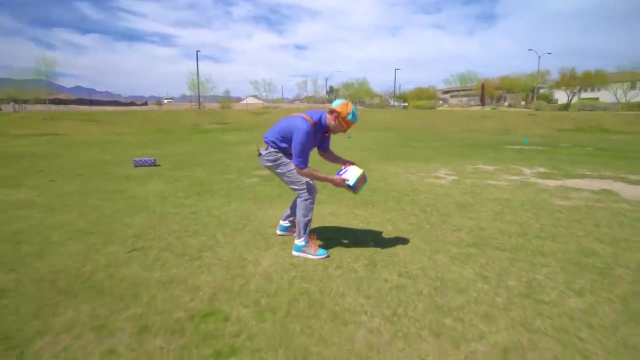 Whoa, Let's go learn our numbers one through ten. Come on, All right, Look at this red box. Wait a second, That's not number one. Let's go check another box. Another wrong box. That's the number nine. 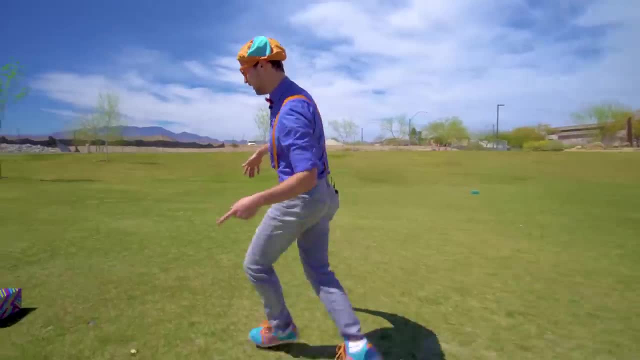 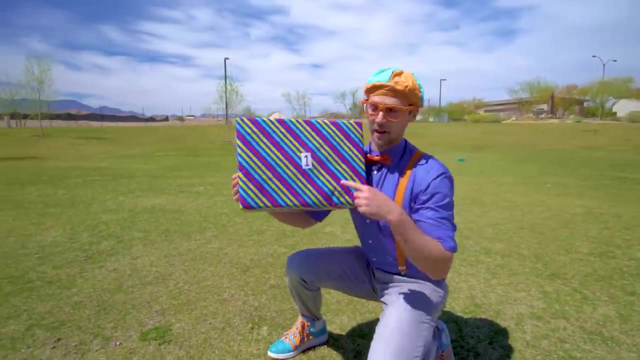 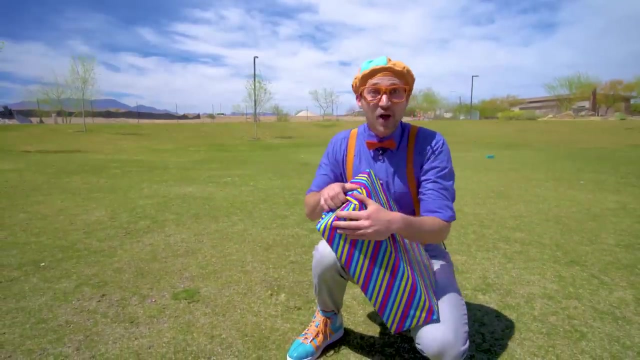 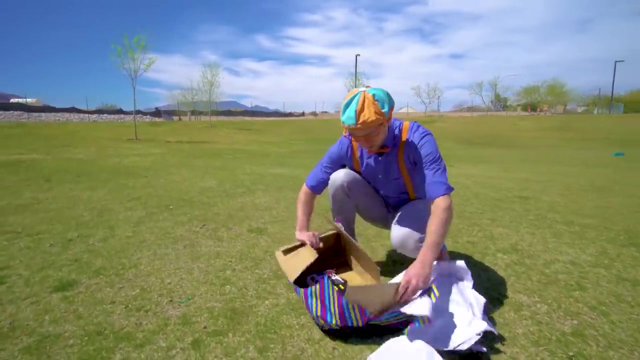 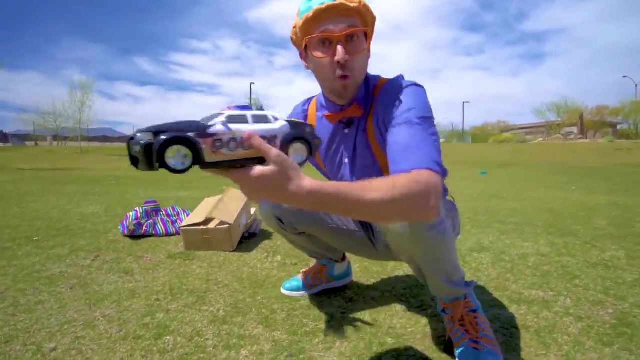 Oh, Here's a box. Ooh, Yeah, Look, We found it, The number one. Ooh, I wonder what's inside. Let's open it up. Look at what it is. Oh, There's one police car. 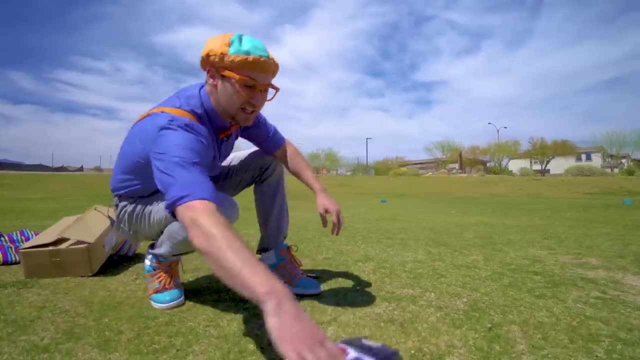 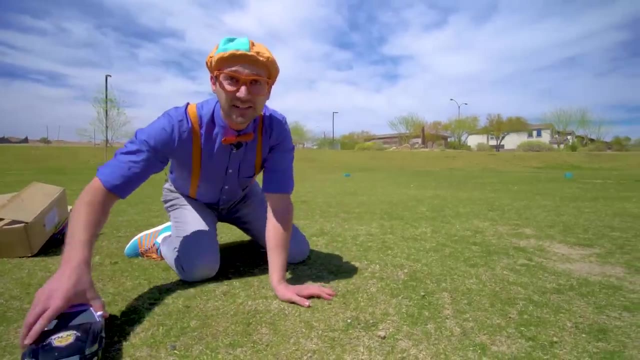 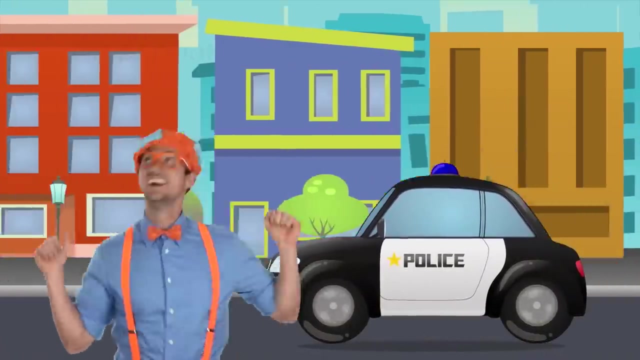 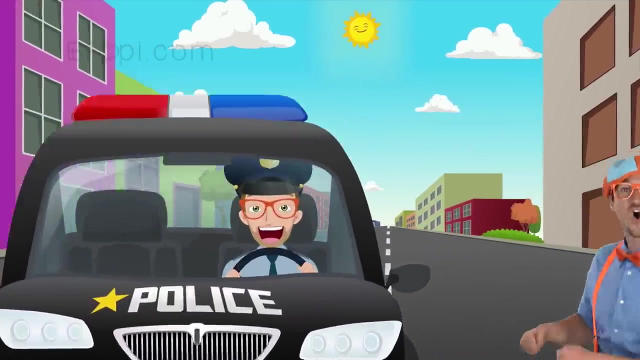 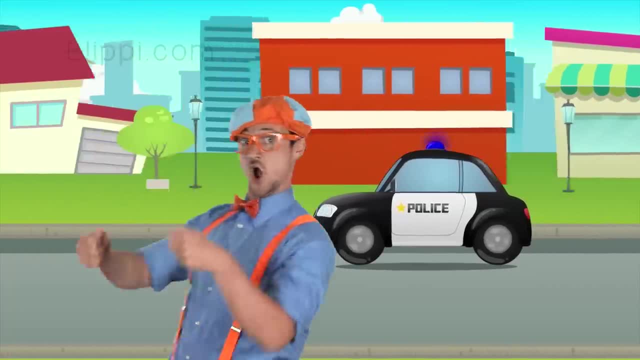 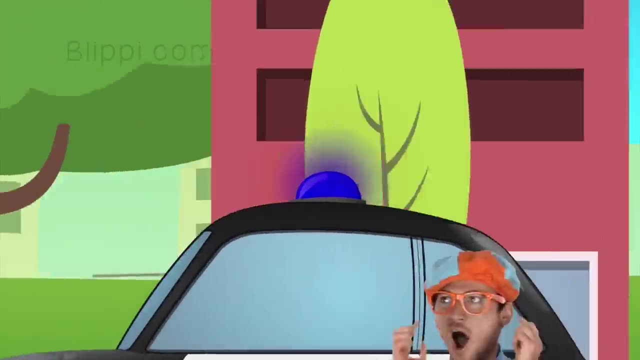 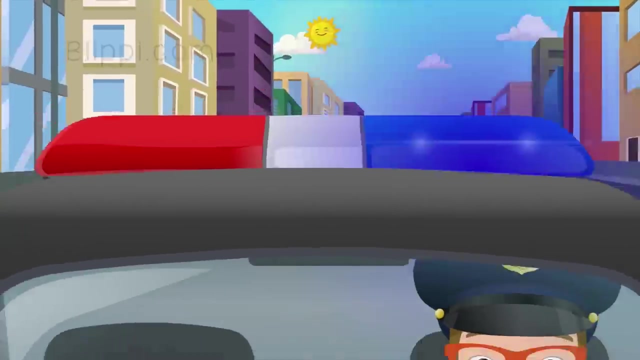 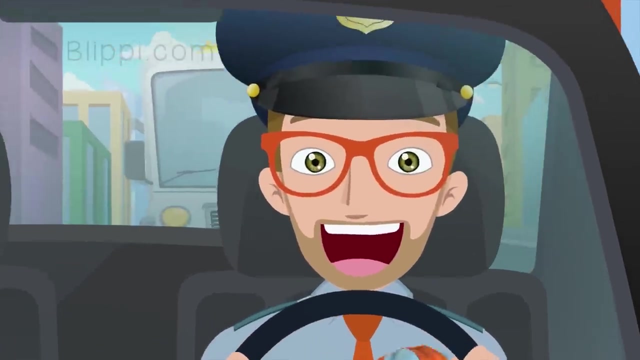 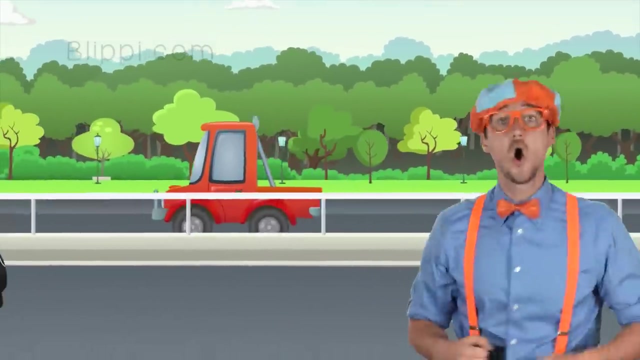 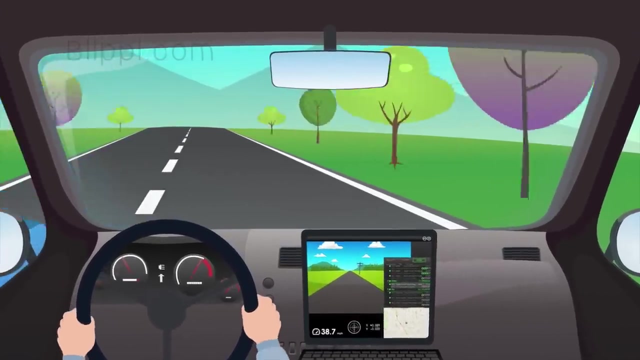 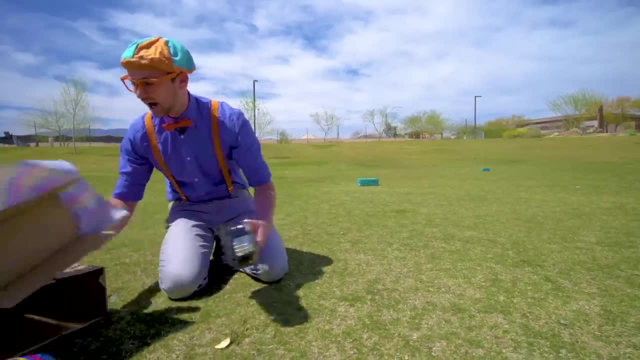 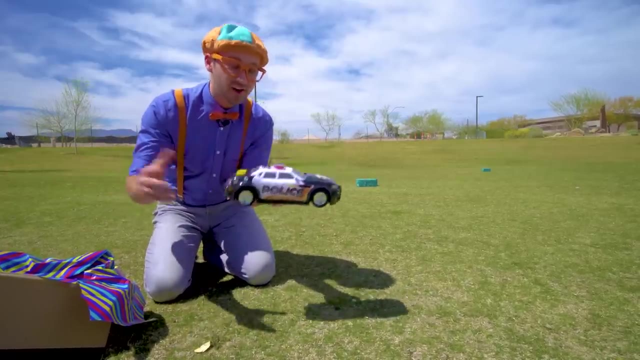 Wee, Wee, Wee, Wee, Wee. Oh geez, I love police cars. Well, one police car, Let's go find number two. Come on, Hup, Hup, Hup, Hup, Hup, Hup, Hup. 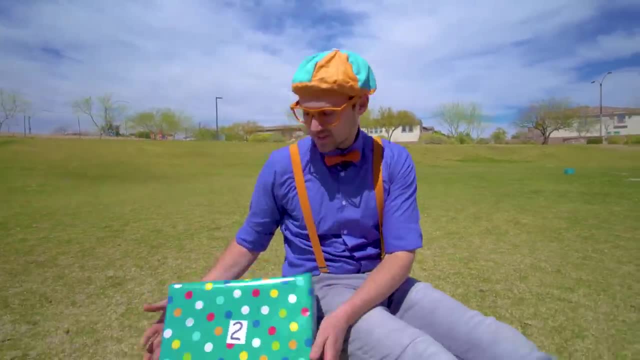 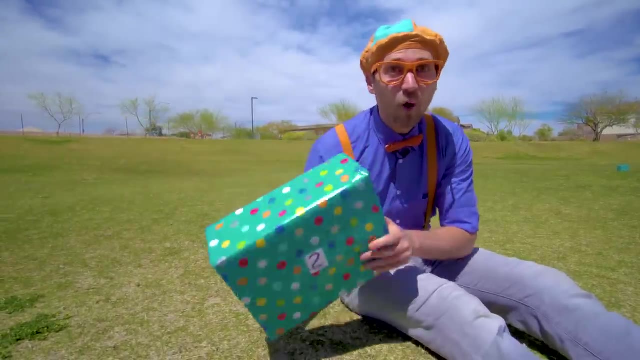 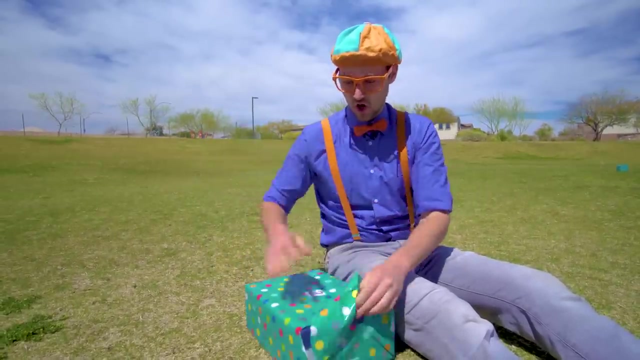 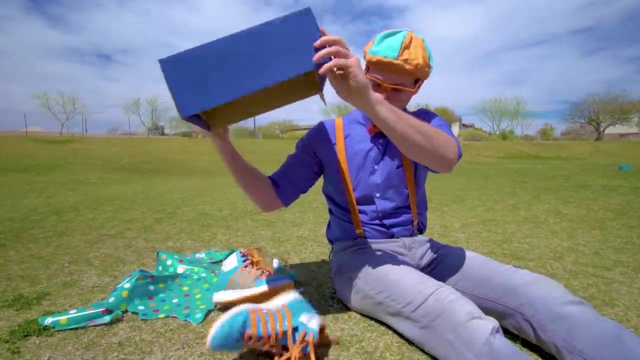 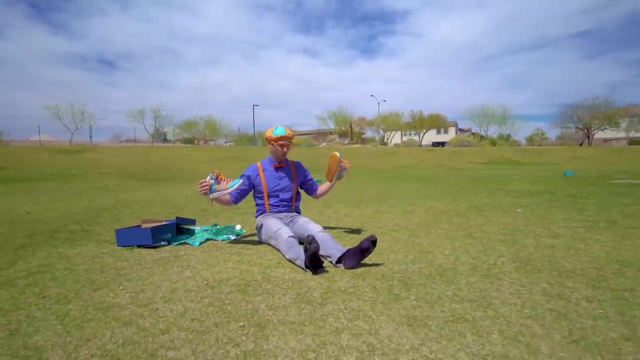 Okay, here is another box. See, This is the number two. Whoa, I wonder what's inside. We gotta open it up to find out. Two shoes. Wait a second. Look, My shoes were in the box, Okay. 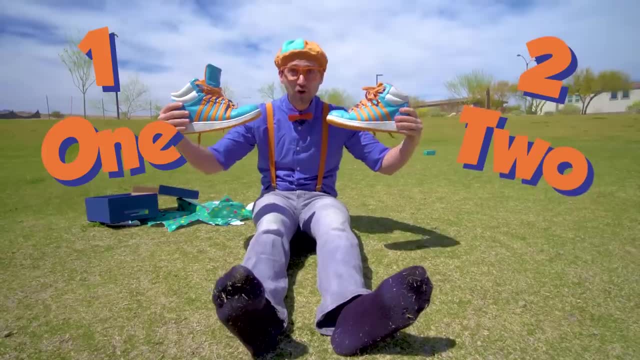 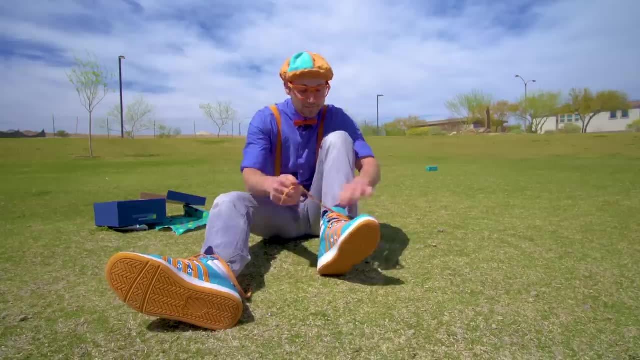 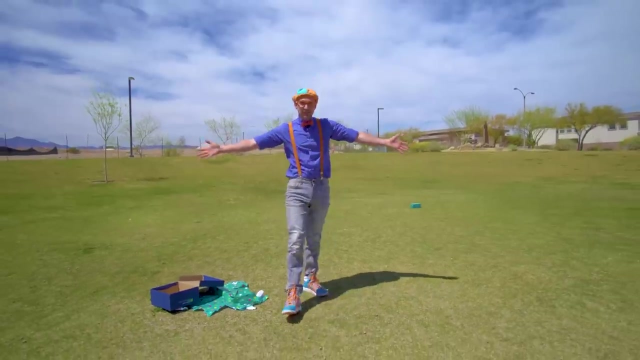 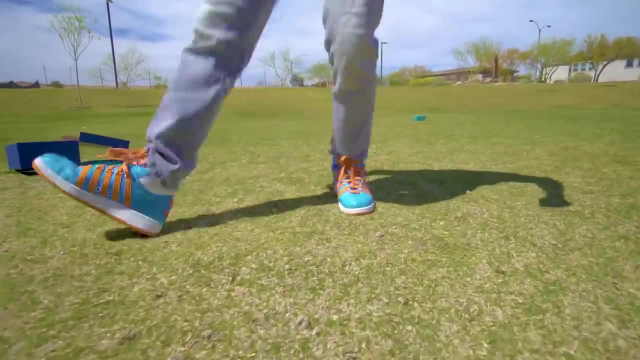 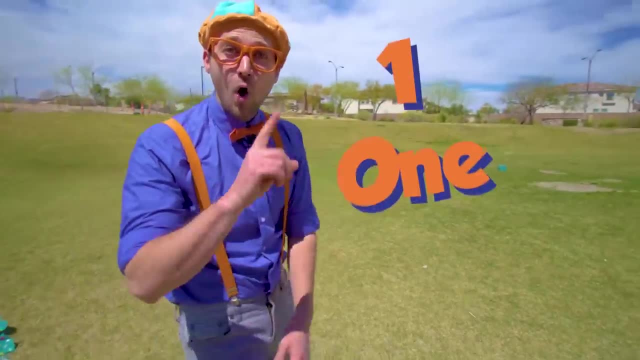 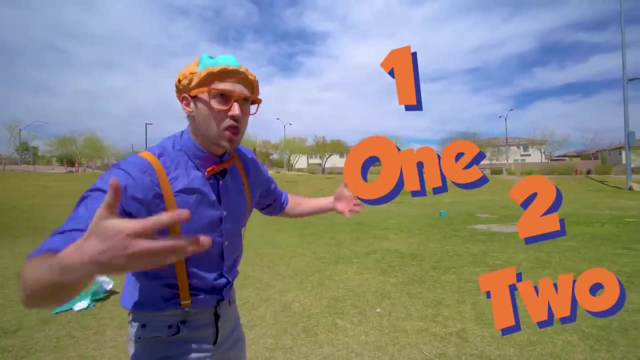 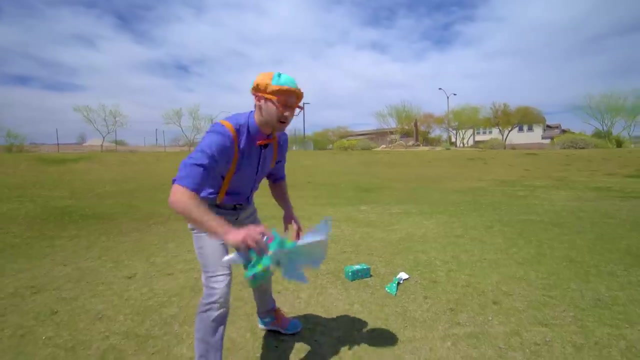 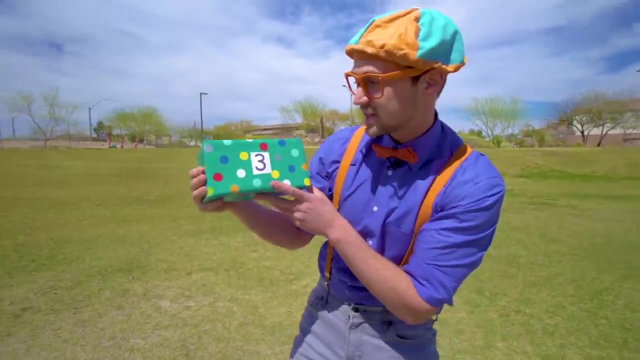 One Two, Ha, Yeah, One Two. Alright, Now let's find the next number, One Two. I know, Look, The paper was telling us to go here. Another box, Whoa. Oh, this box has the number three on it. 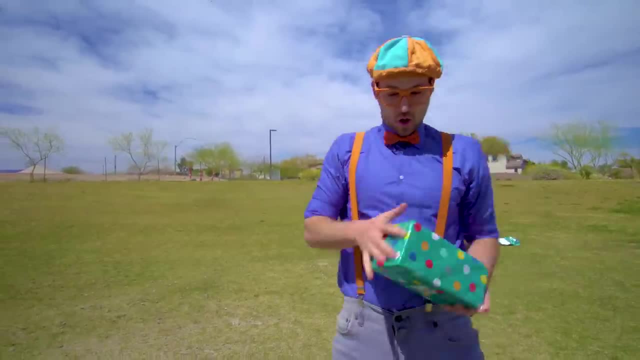 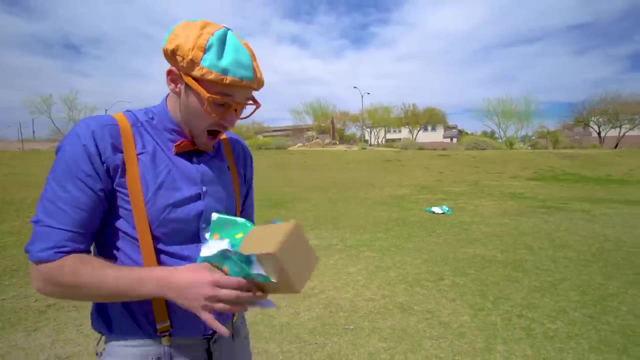 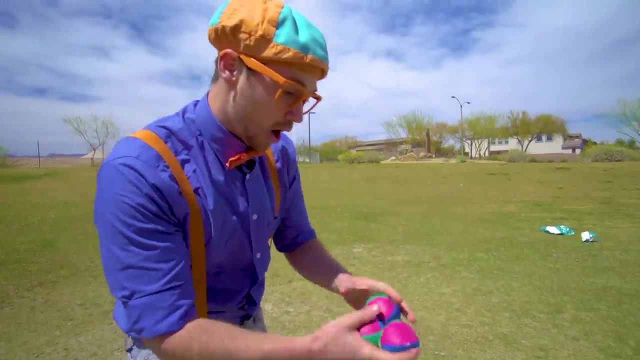 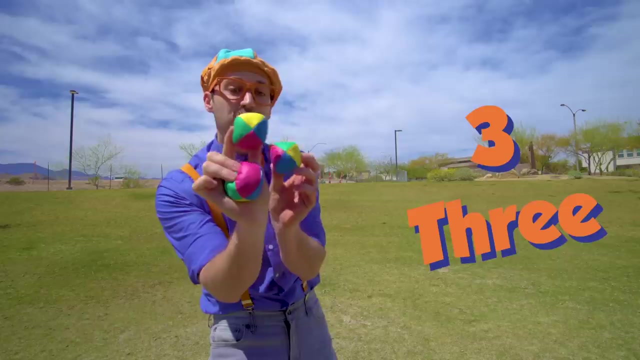 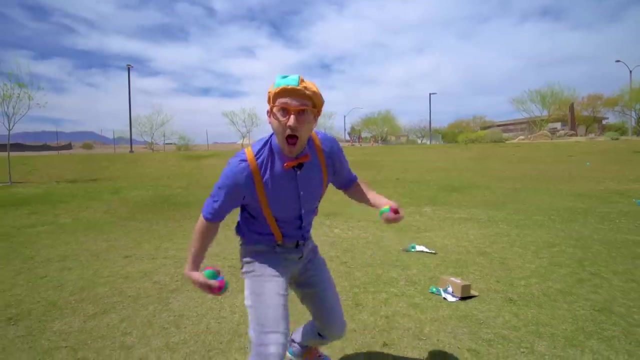 One, two, three. Let's open it up. I'm so excited. Okay, here we go. Look three balls: One, two, three. Huh, I wonder what I can do with three balls. I can juggle. 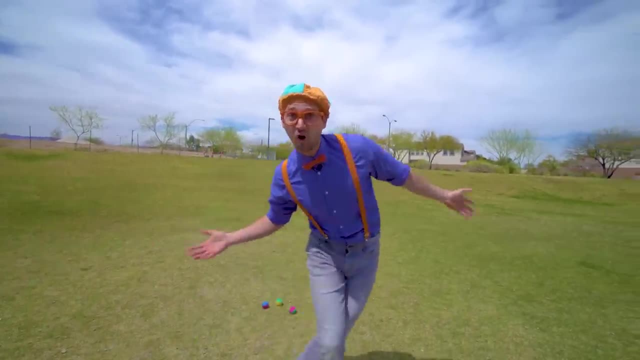 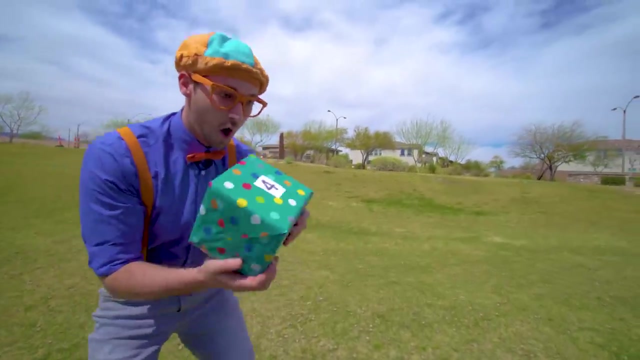 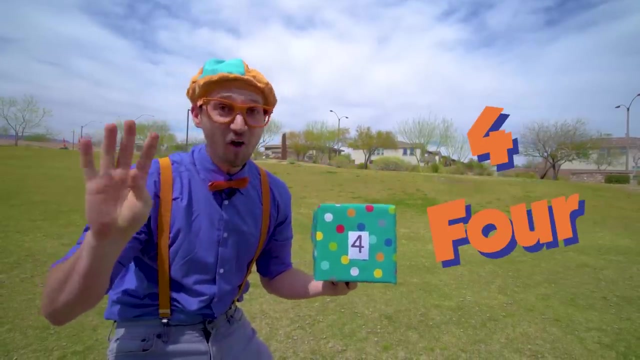 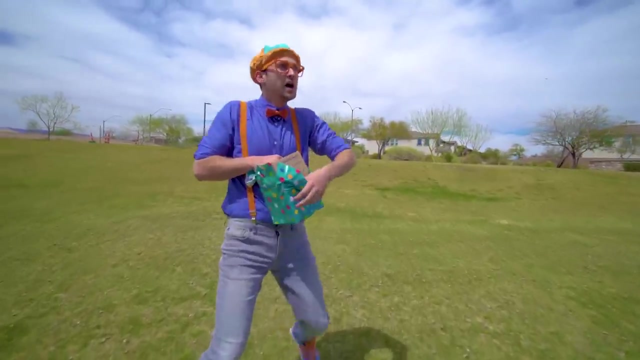 I love juggling. All right, let's go find number four. Oh, look another box. Oh, and this has the number four on it. One, two, three, four. Let's open it up. Oh, this is so tiring. 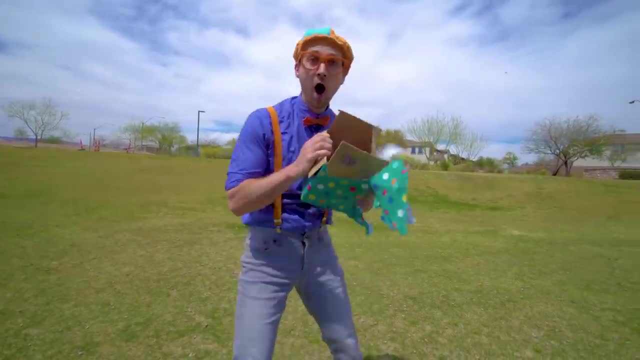 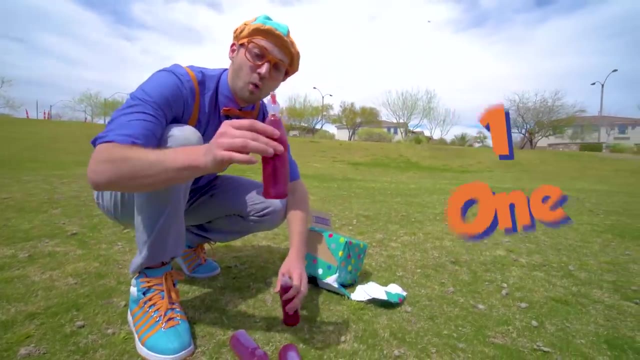 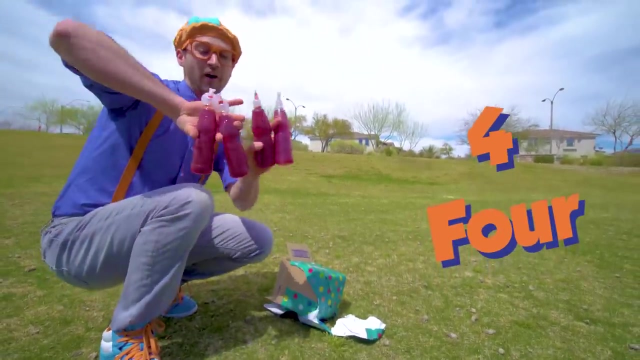 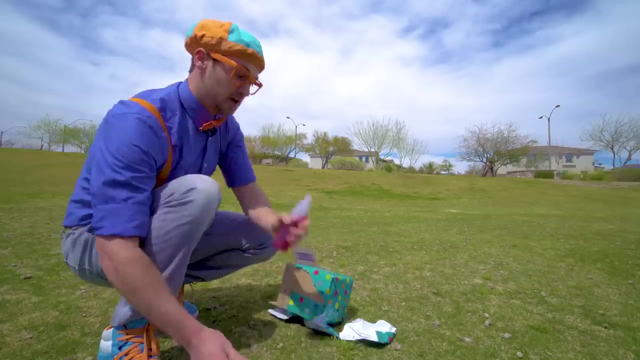 I am so thirsty. Look Yeah, four juice boxes: One, two, three, four. One, two, three, four, Four. Whoa, All right, Yum, Here we go. Yeah, Bye-bye, juice. 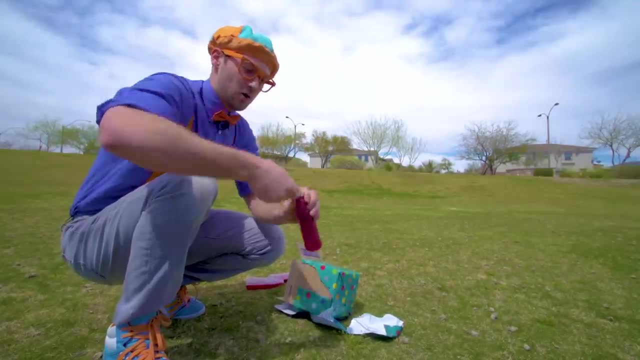 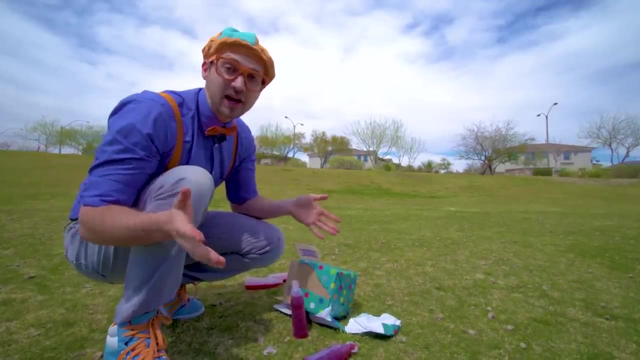 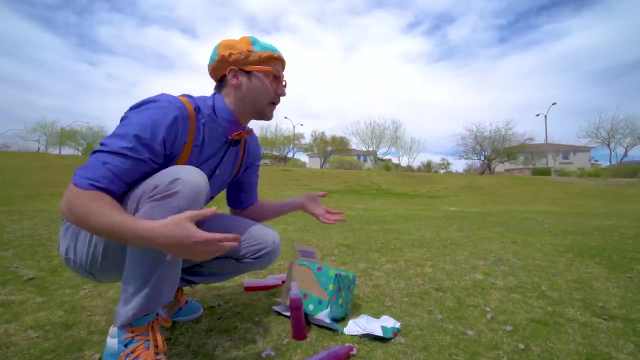 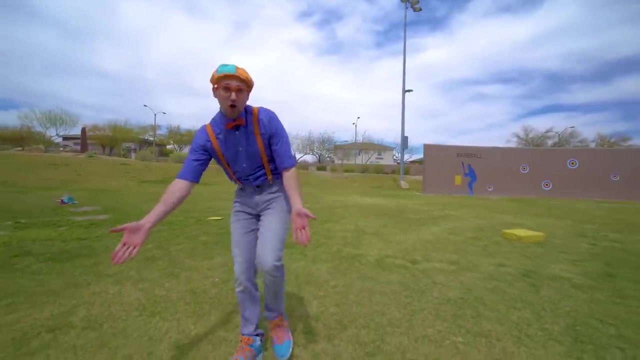 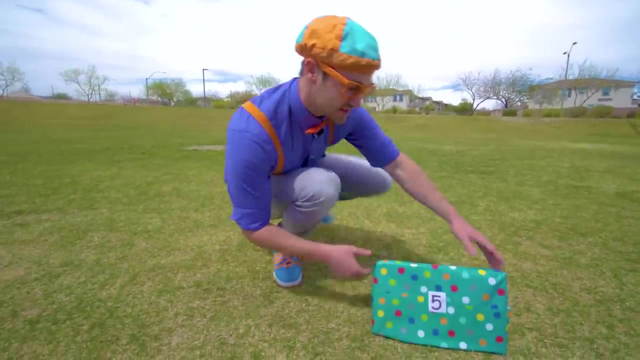 Whoa, Okay, last one. Oh Okay, Ugh, hydrated and we learned numbers one, two, three and four. let's go find the next number. Look Here- it is Another box- And look at what this says. This has the number five on it. One: 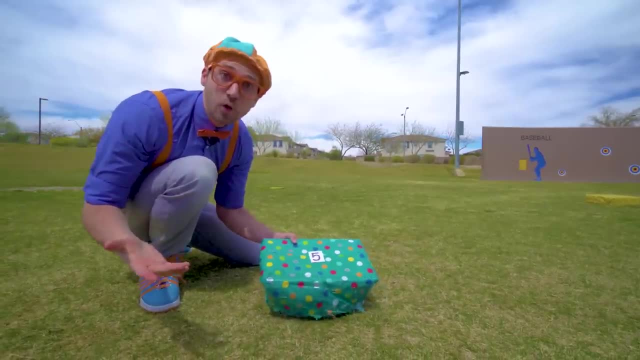 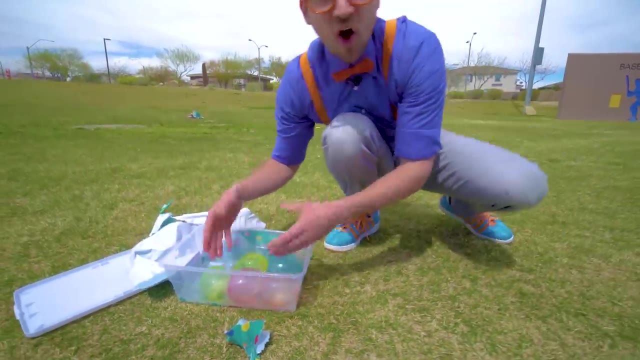 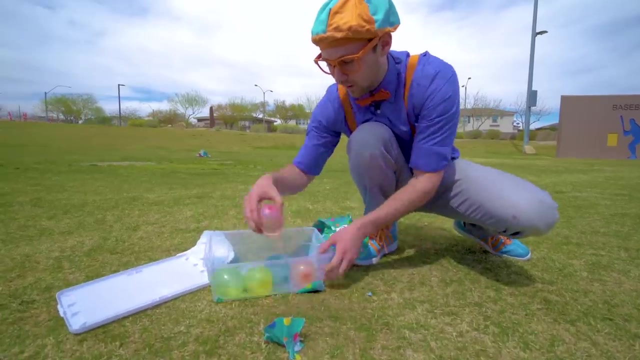 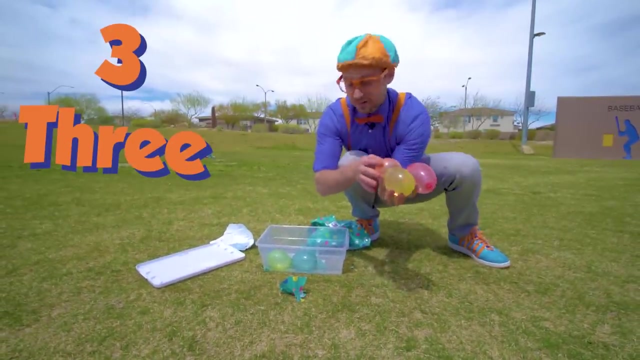 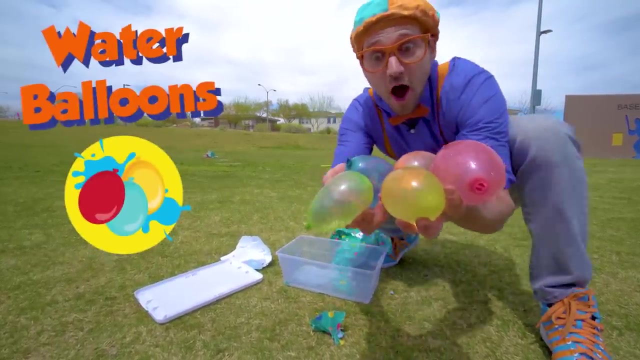 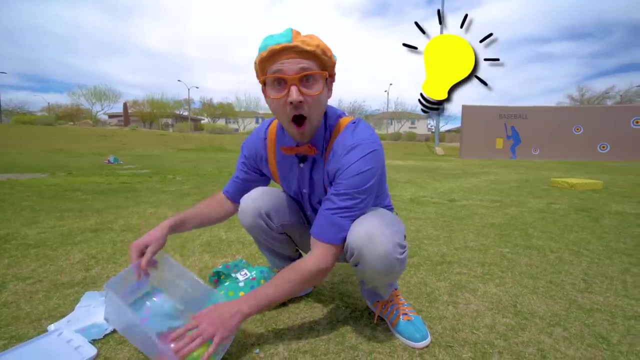 two, three, four, five. I wonder what's inside. Oh look, Water balloons. Five water balloons. Dump out. Okay, we have one, two, three, three, four and five water balloons. What can you do with water balloons? I have an idea. Hey, Dee, Dee, Dee Dee. 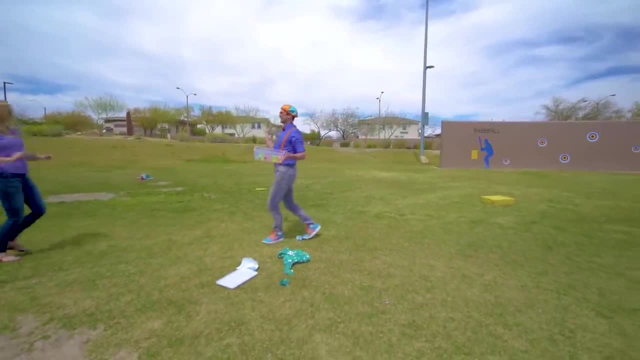 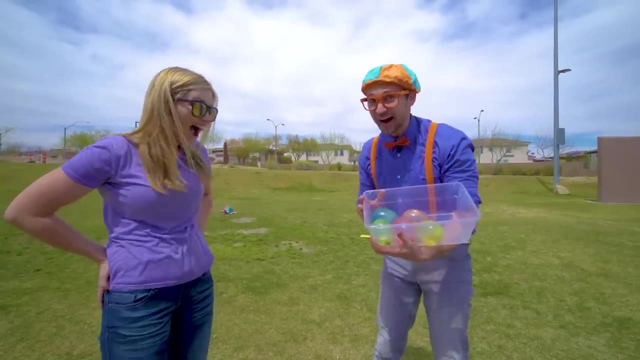 come here. Hey, how are you Blippi? Oh good, Hey, I had a question. Do you want to have a water balloon fight? Yeah, Blippi, that sounds so fun. How many water balloons do I get, You get? 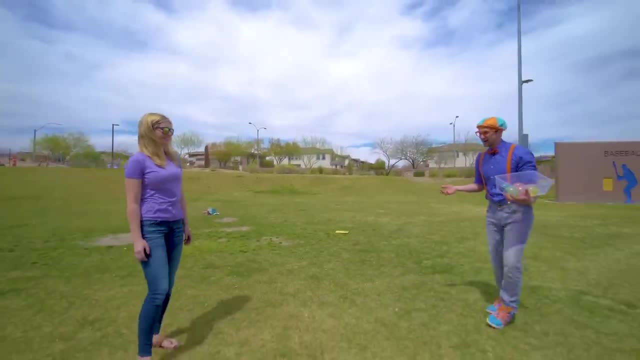 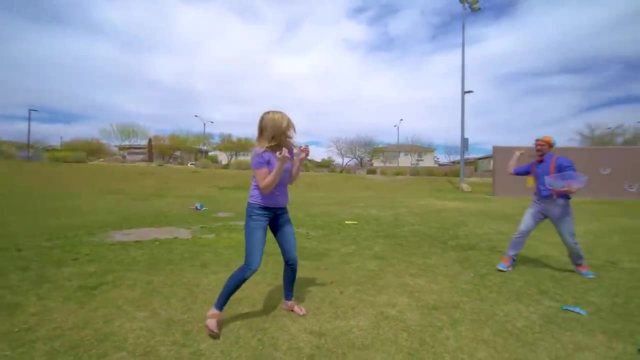 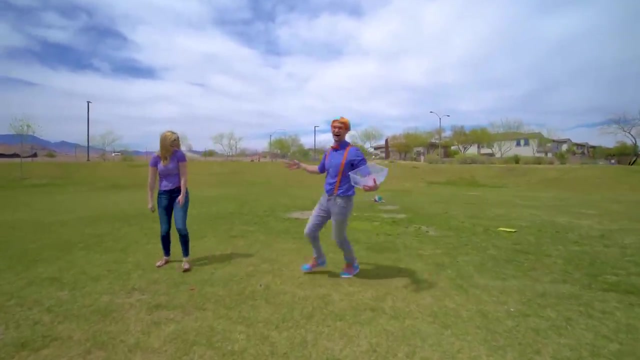 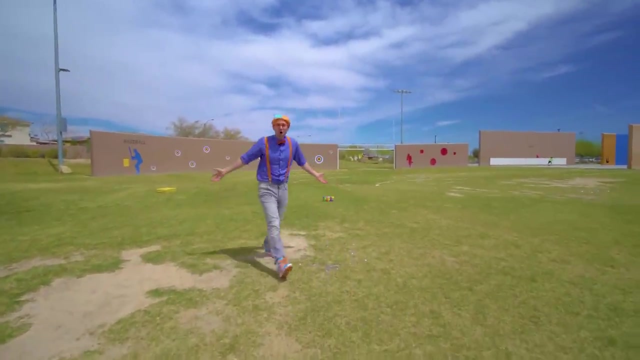 zero. All right, Are you ready, Blippi? That was such a fun water balloon fight. That was so much fun, All right now- that we learned numbers one, two, three, four, five, six, seven, eight, nine, 10,, 11,, 12,, 13,, 14,, 15,, 16,, 17,, 18,. 20,, 21,, 22,, 23,, 24,, 25,, 26,, 27,, 28,, 29,, 30,, 31,, 32,, 33,, 34,, 35,, 36,, 37,, 38,, 38,, 39,, 40,, 42,, 43,, 44,, 45,, 46,, 39,, 40,, 42,, 45,, 46,, 47,, 49,, 40,, 49,, 50,, 51,, 52,, 53,, 44,, 45,, 46,, 47,, 49,, 50. 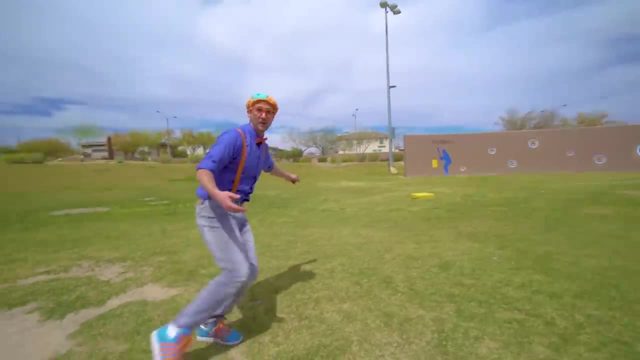 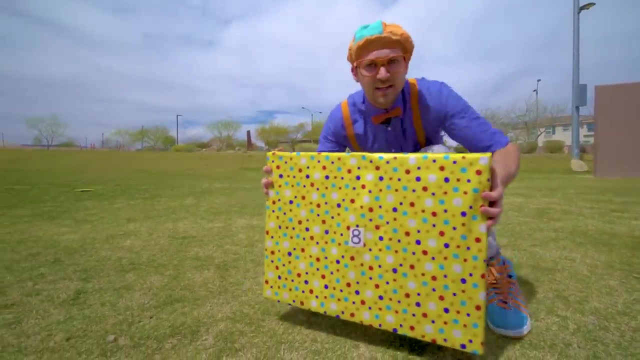 Now I'm going to go find the next number. No, let's go find the next number. Look a big box back there. Oh, look at this big yellow box. Wait a second, That's not the next number. Let's get to this one later. 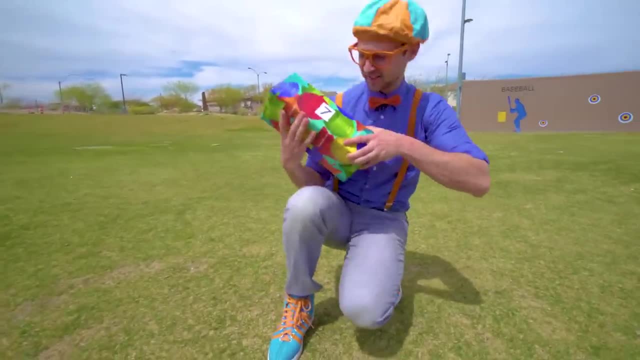 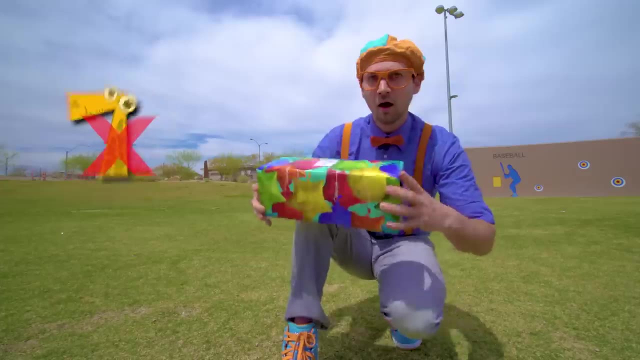 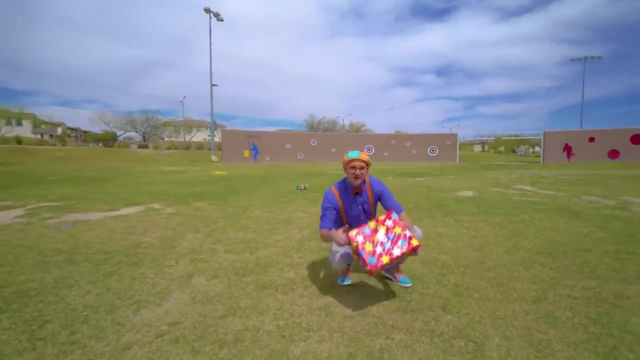 There's another box. Yeah, we found a box, But wait a second. Do you see that That's not the next number Must be another one. Here's one. Yeah, We found a box And look, That is the number six. 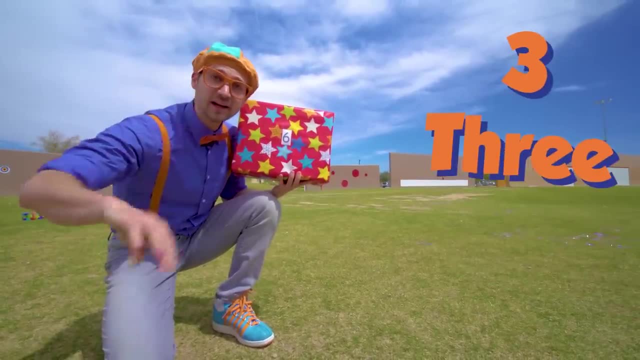 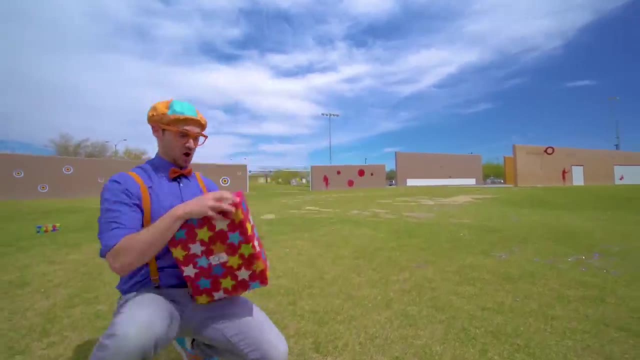 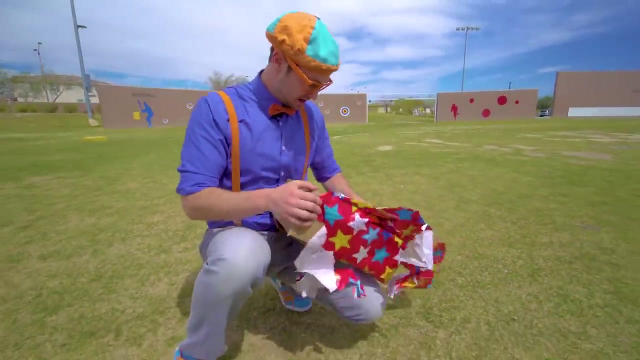 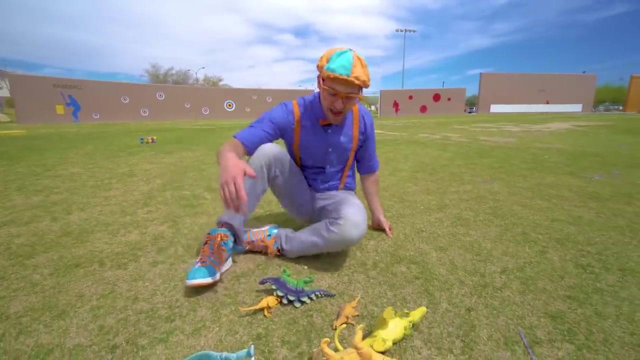 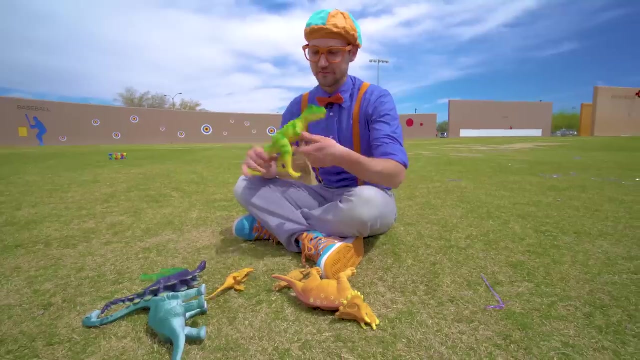 One, two, three, four, five, six. Alright, let's open it up and see what's inside. Yeah, Yeah, Whoa, Look, Yeah, Dinosaurs, I love dinosaurs. Okay, let's see what ones we have. 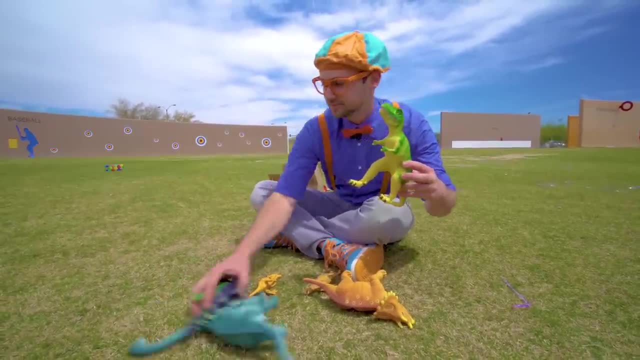 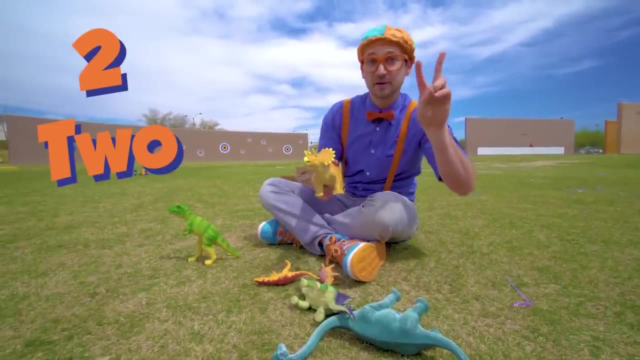 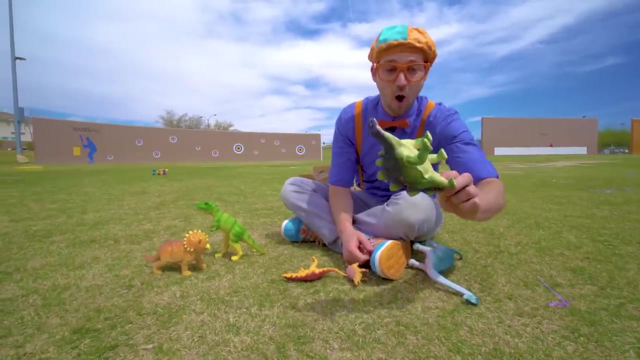 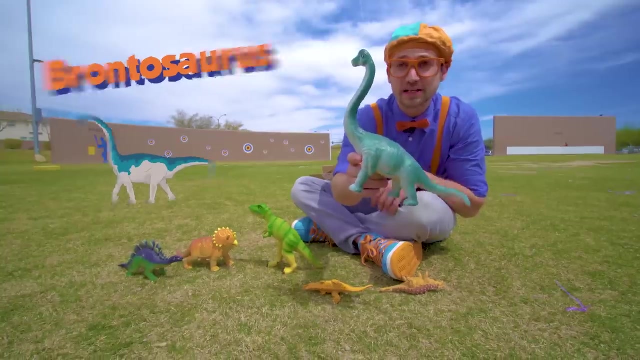 A T-Rex, That's number one. One Ooh A Triceratops, That's number two. Ooh A Stegosaurus, Whoa Number three. Ooh Brachiosaurus, Or a Brontosaurus. 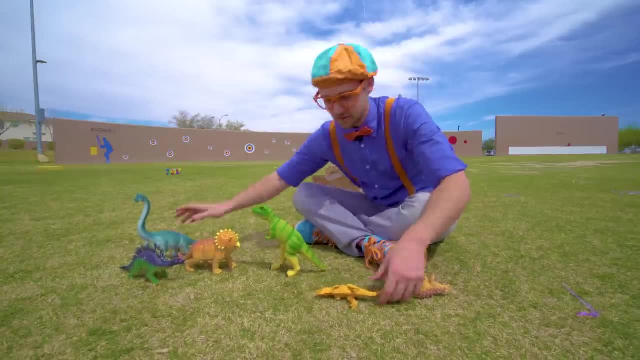 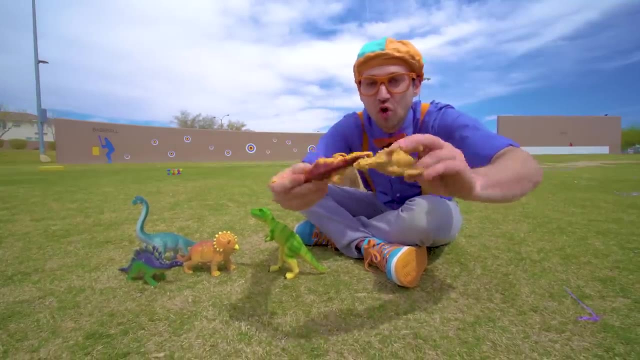 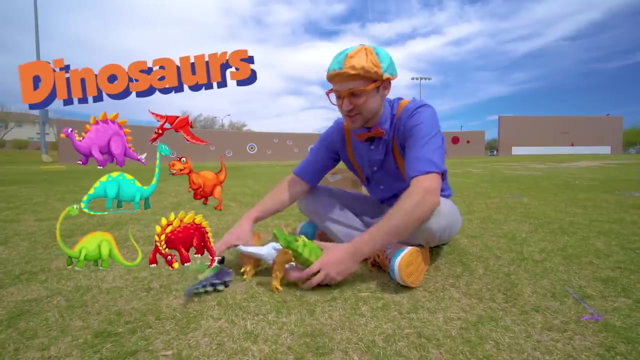 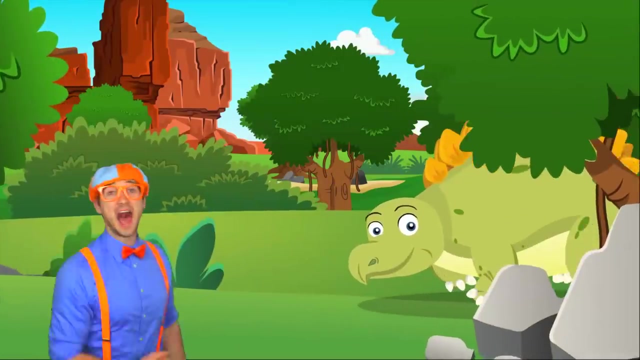 That's number four, Oh, And two little ones. So we have one, two, three, four, five, six dinosaurs. Whoa, This is the perfect time for the Blippi Dinosaur Song. Dinosaur, Roar, Dinosaur. 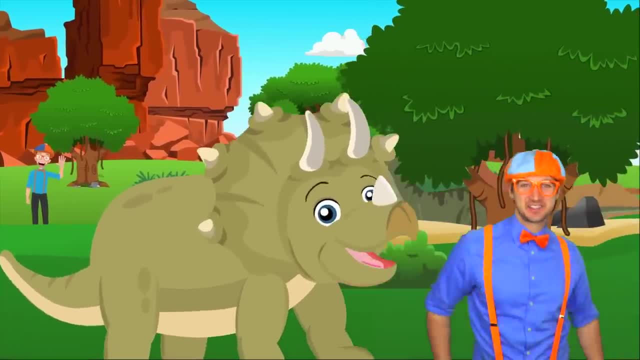 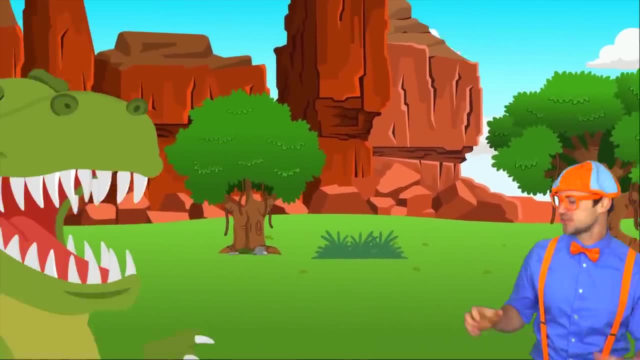 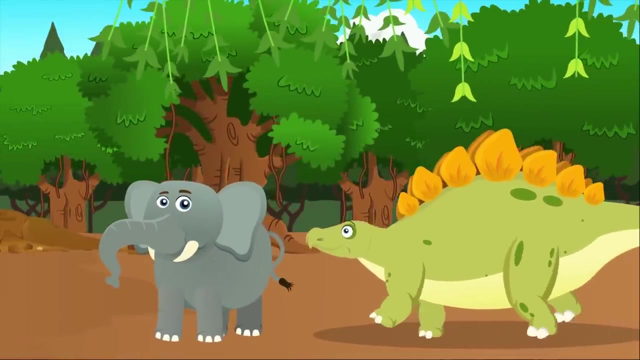 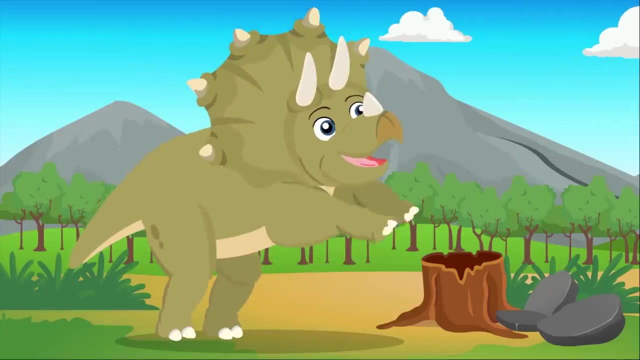 Oh, I love dinosaurs. Roar, Dinosaur Roar, Prehistoric dinosaurs, Roar Roar, Stegosaurus, Dinosauphores, Dinosaur film, Ba spunk, Dinosaur stuff, Ha, Even the giant ones get turned inside out. 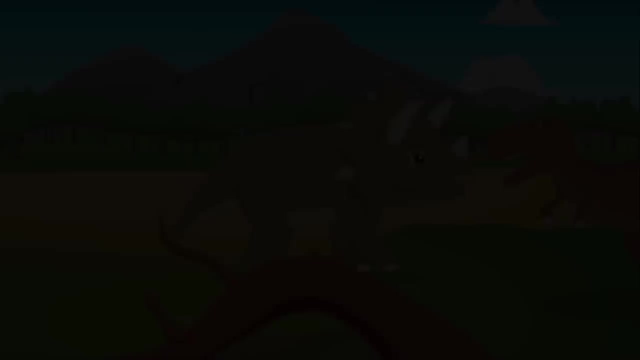 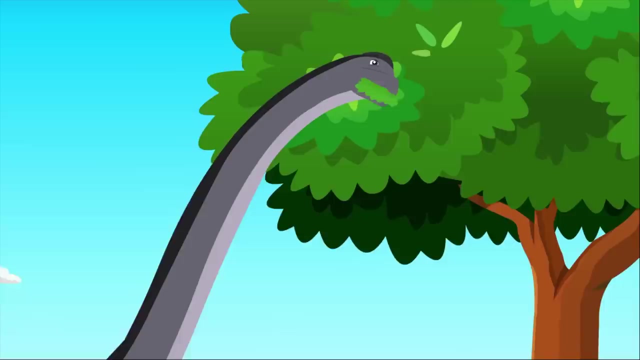 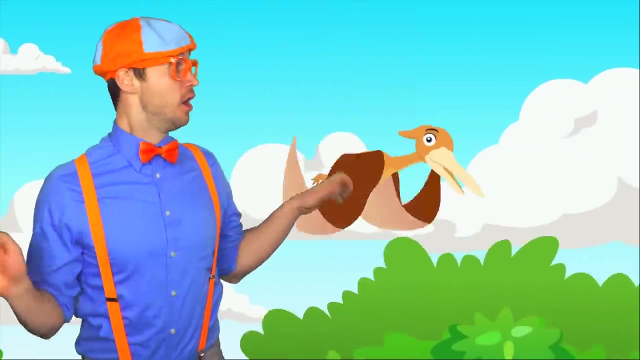 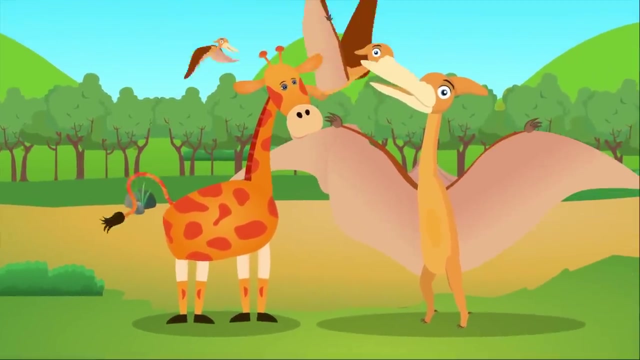 testimi metabolic Justin Race theme song. The Brachiosaurus had a really long back and at the end was a itty bitty head. Pterodactyls would soar through the sky their wings And if they stood up straight on the ground they would be as tall as a giraffe. 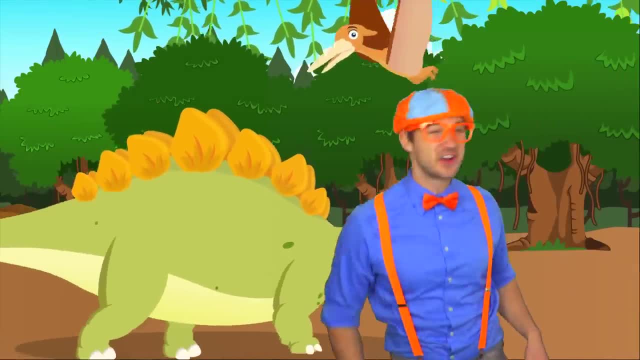 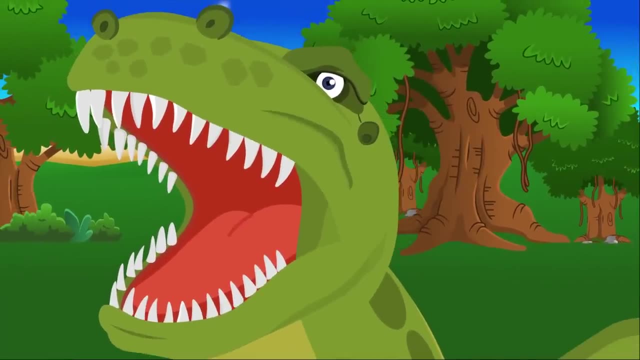 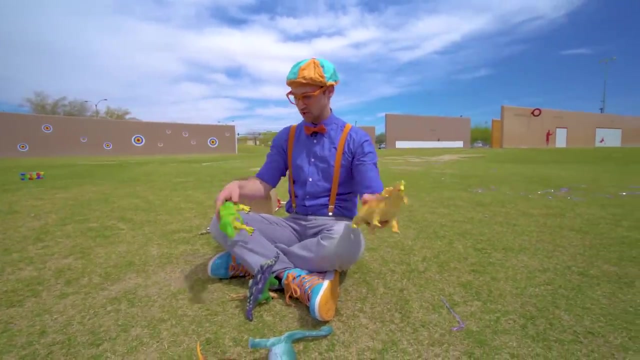 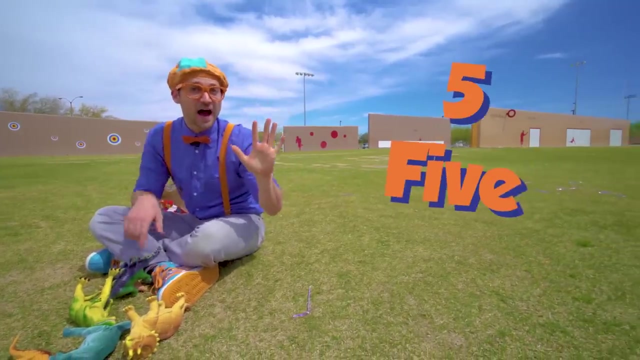 Dinosaur Roar. Dinosaur Roar. Oh, I love dinosaurs Roar. Oh jeez, I love dinosaurs. All right, We've learned numbers one, two, three, four, five and six. 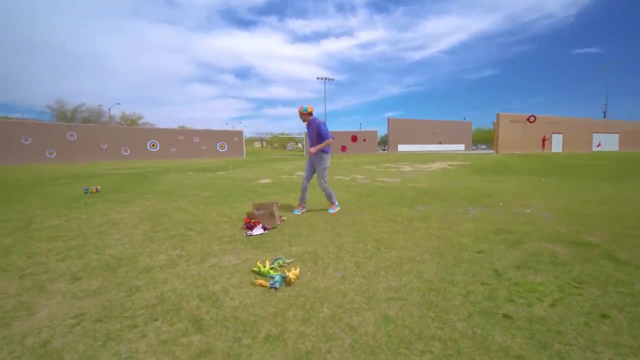 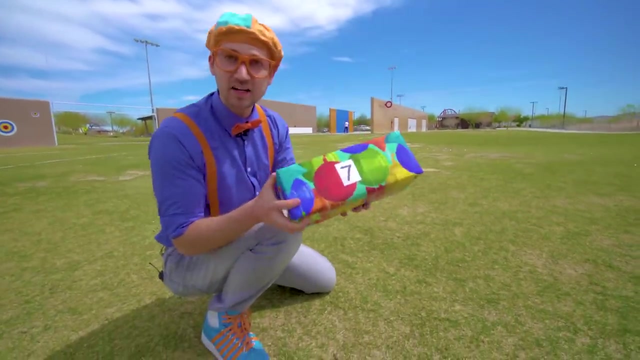 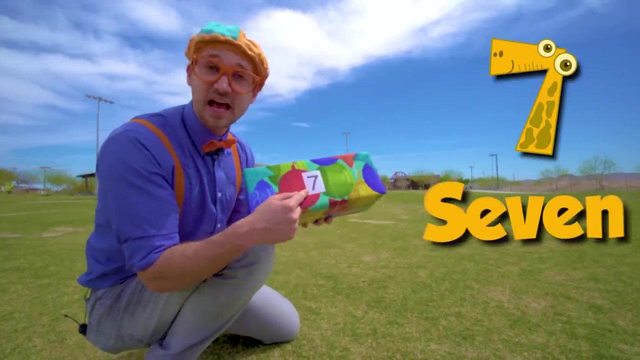 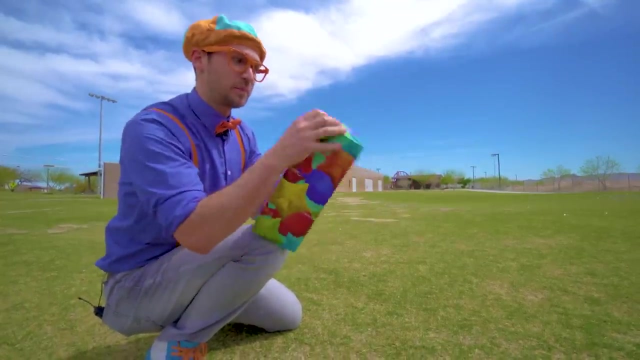 Let's go find the next number. Yeah, I remember this one, It was the box that came after the dinosaur. Let's look down here the next one, because we already saw the number Number seven. What's inside, I don't know. 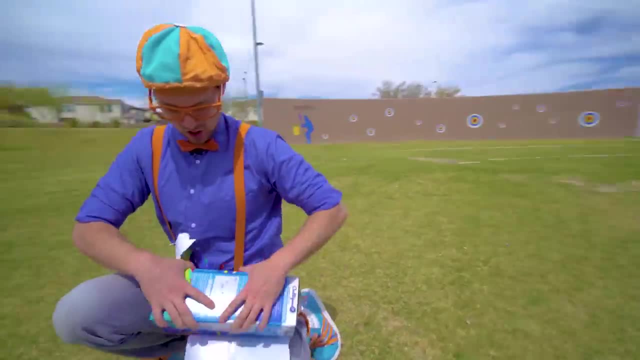 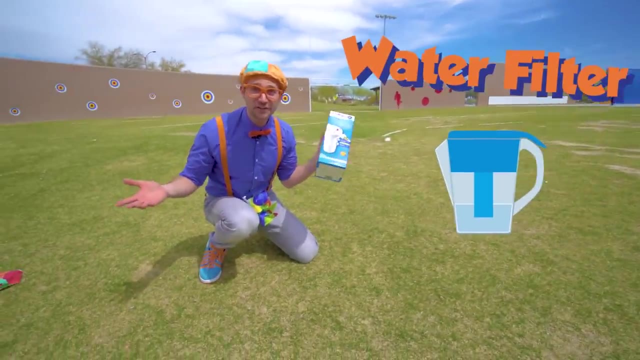 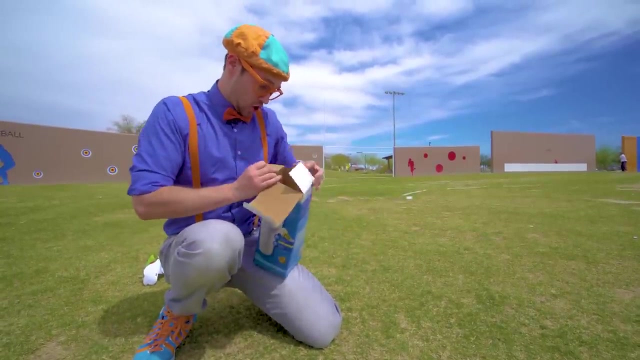 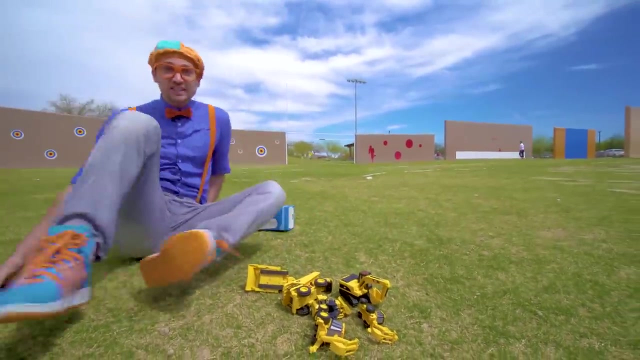 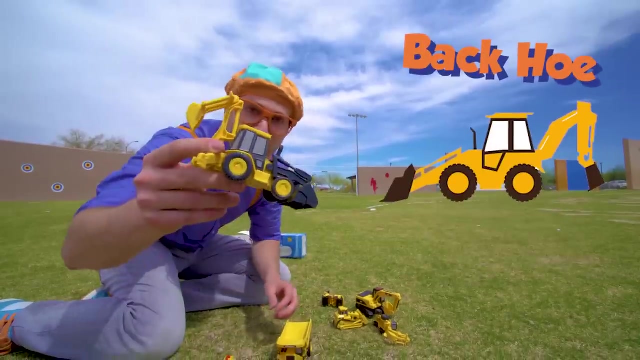 Let's open it up. Whoa, Look, It's a water filter. Huh, That's not that interesting. Maybe something's in here. Dinosaur construction toys- that's way more cool, check them out. a bulldozer, a dump truck, a backhoe. 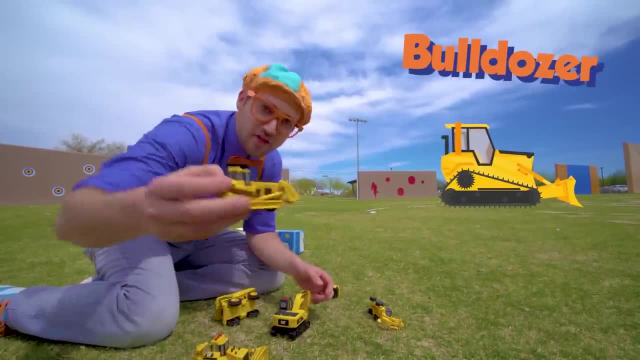 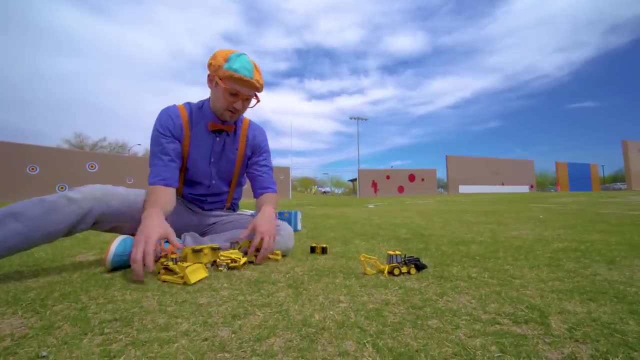 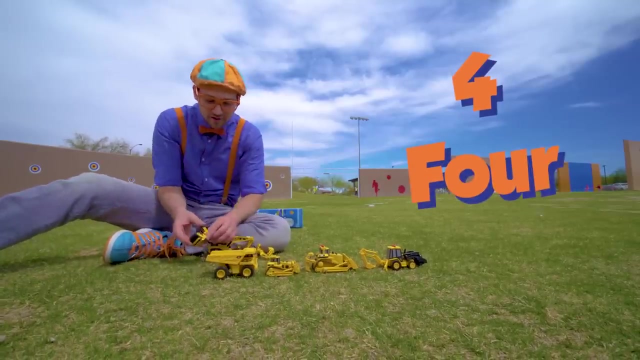 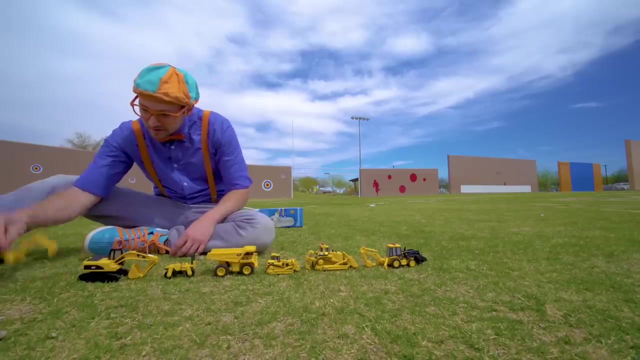 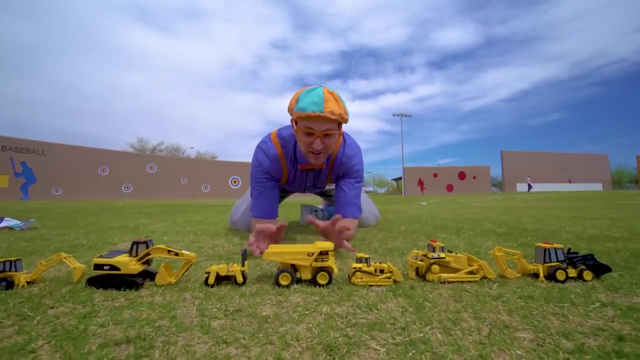 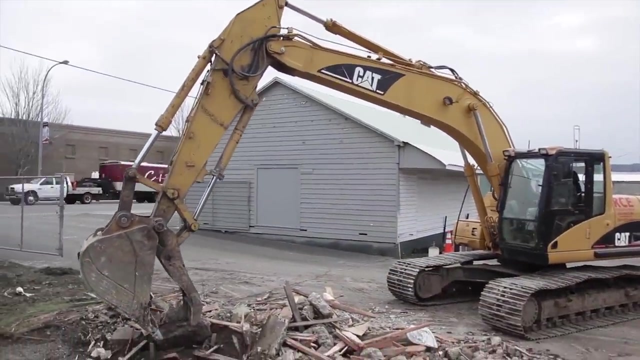 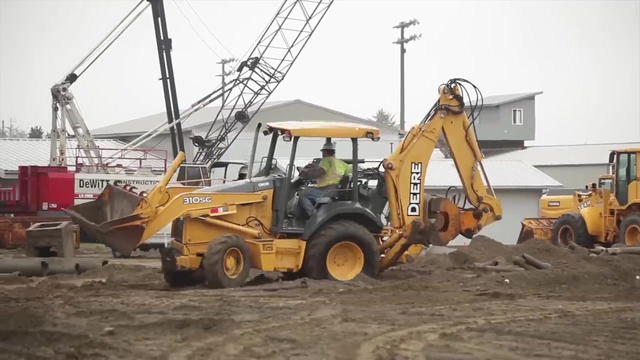 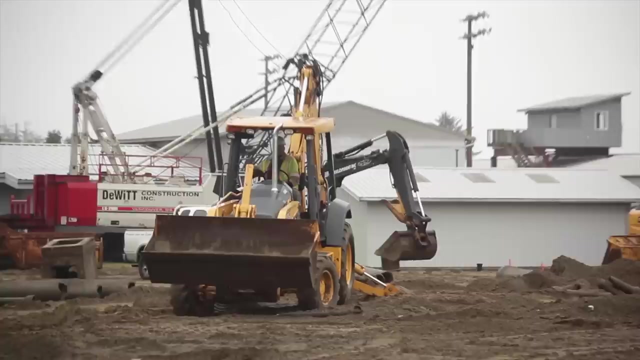 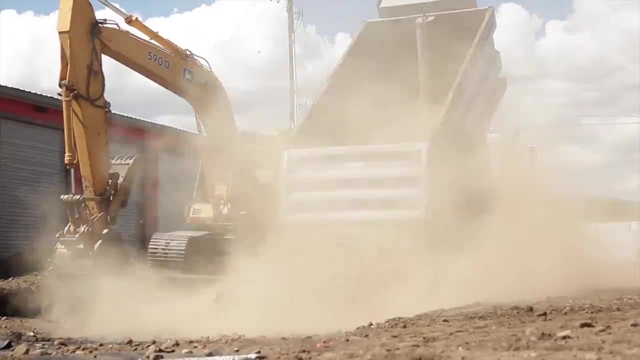 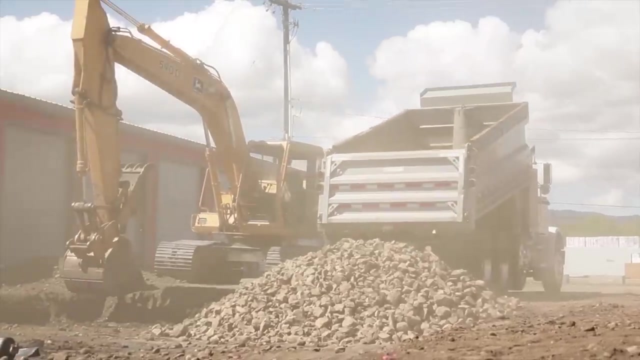 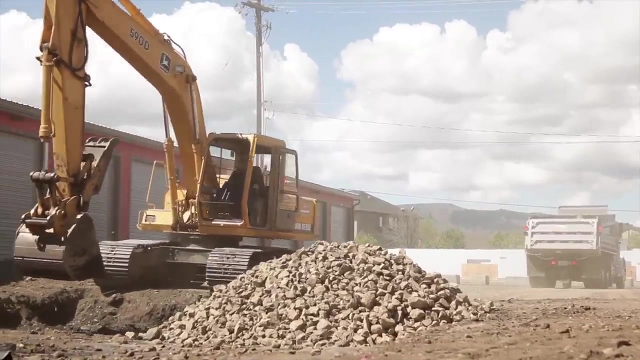 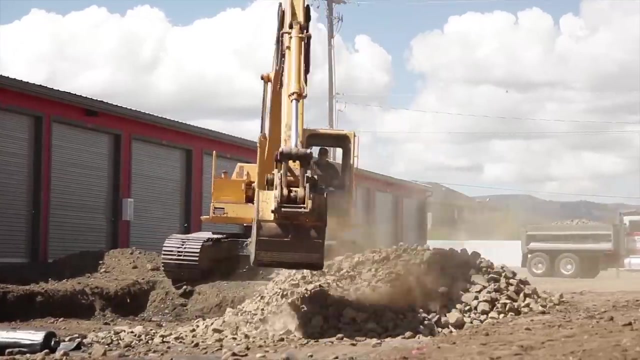 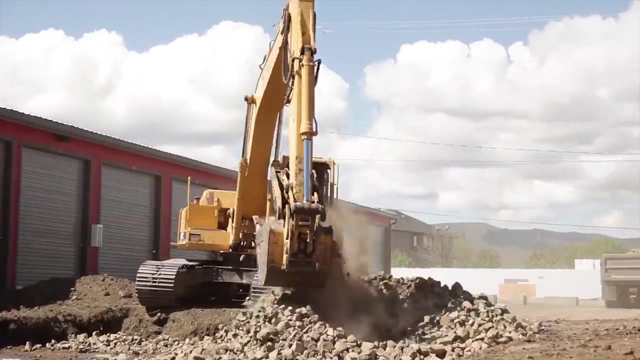 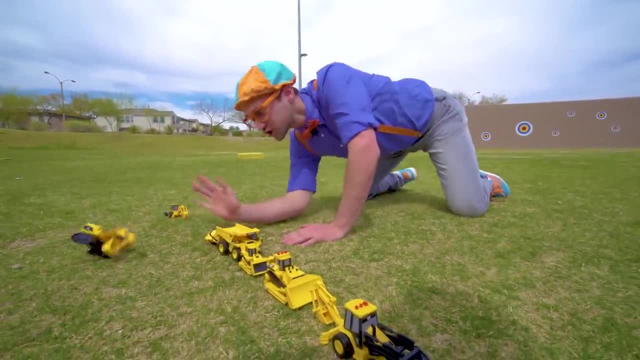 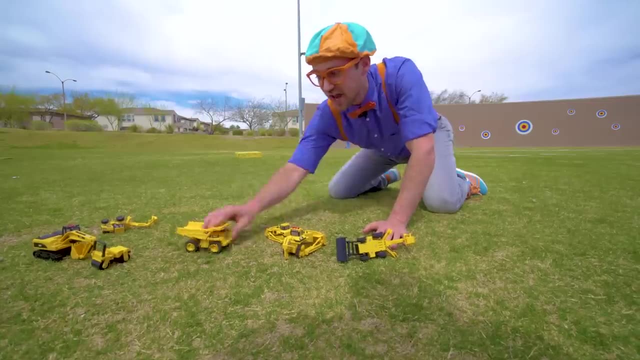 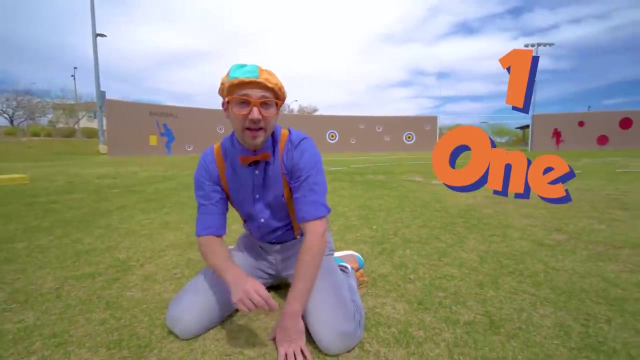 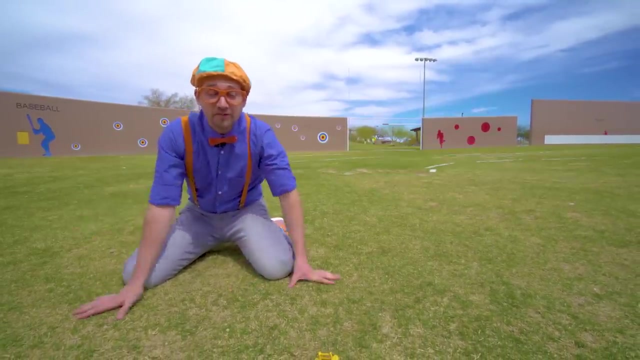 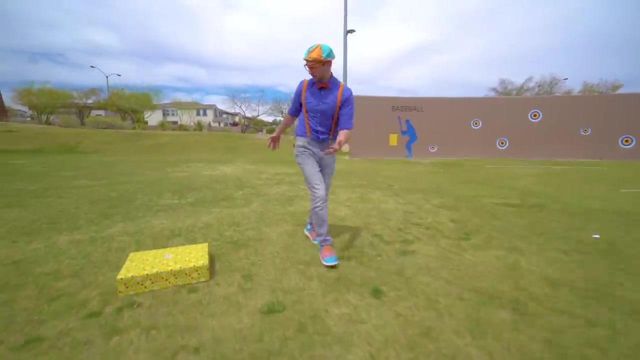 they're so cool how they can push things out of its way and also dig giant holes and dump stuff out of the back. ha ha ha. alright, so we have learned numbers one, two, three, four, five, six and seven. lets go find the next number. Oh yeah, We saw this number earlier, Remember, Yeah, the big yellow box. 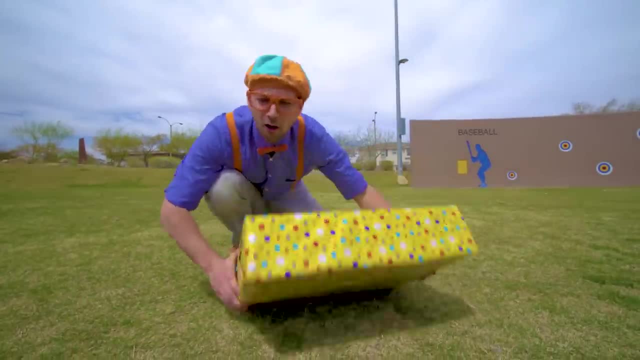 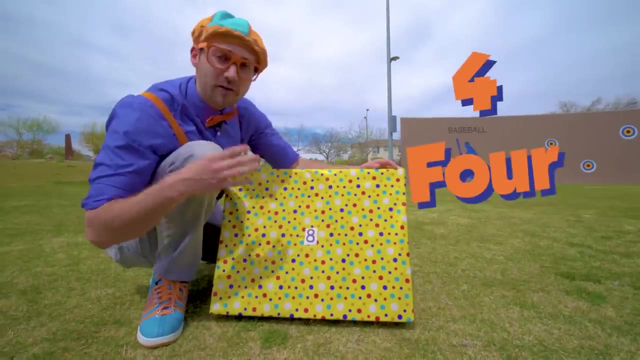 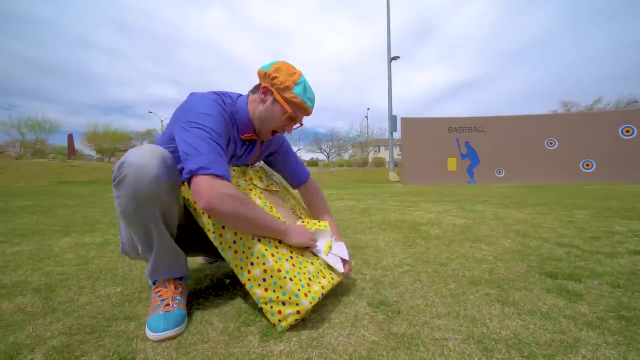 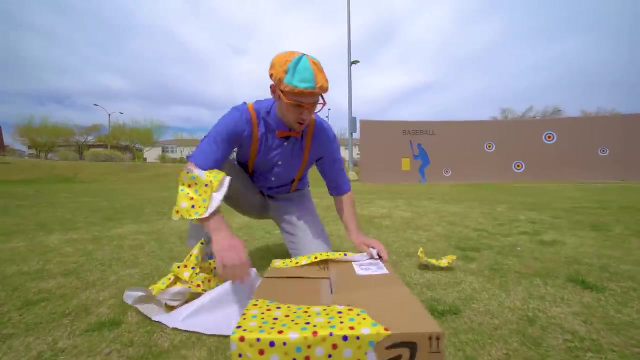 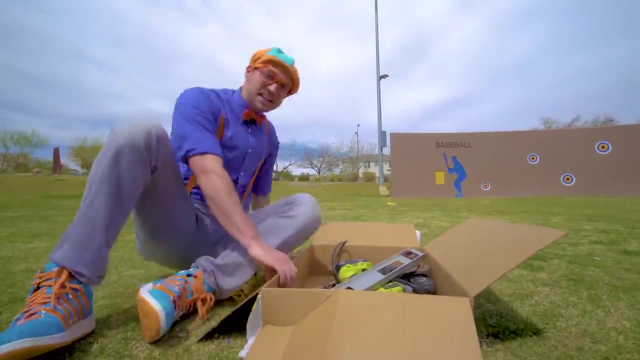 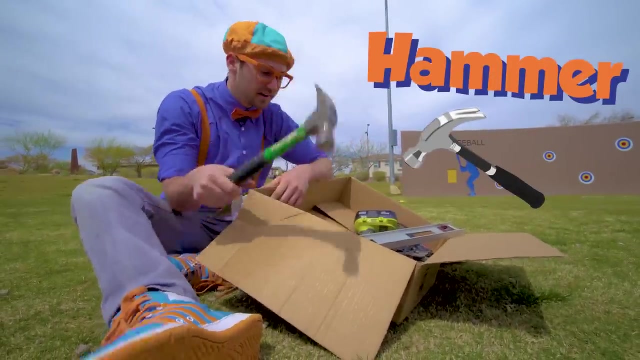 Whoa, This one's really heavy. Okay, It says eight: One, two, three, four, five, six, seven, eight. There must be eight things inside. I wonder what's inside? Whoa, Whoa, Look, This is awesome. There's tools. Okay, We have a hammer, We have a level. 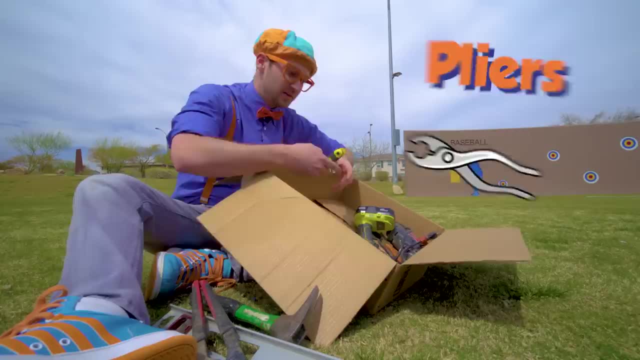 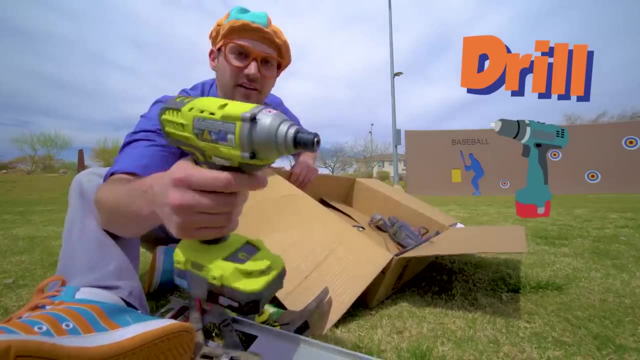 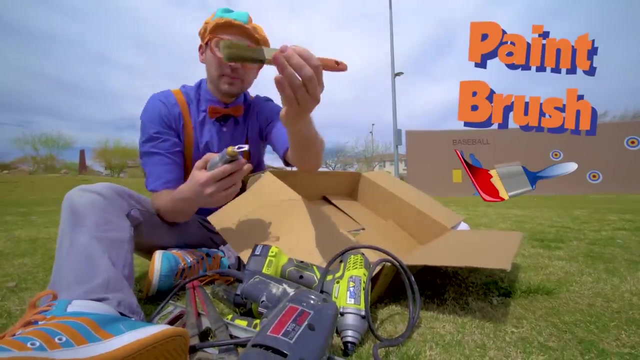 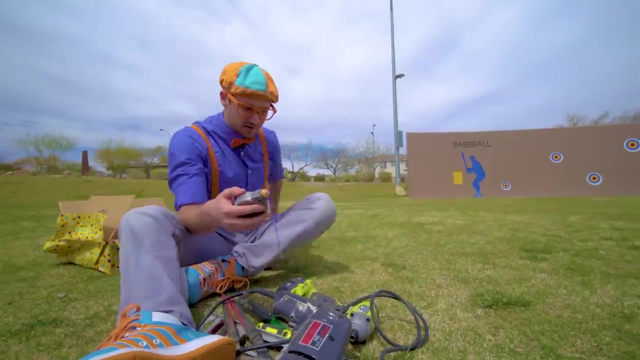 Ooh, A pair of pliers. Ooh, Some Allen wrenches. Ooh, A drill. Ooh, That one was wireless. This has a cord, a paintbrush and a chalk line. Whoa, All right, Let's count them. Okay, Let's see, here We have one tool. 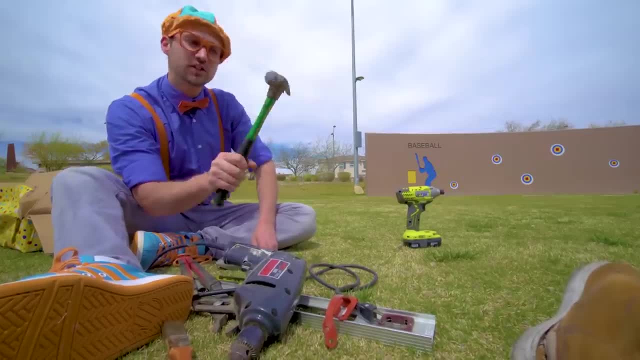 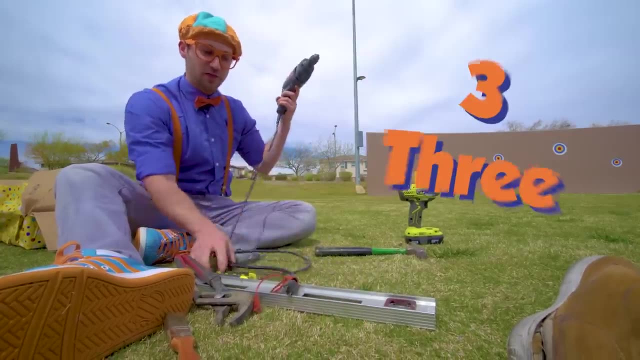 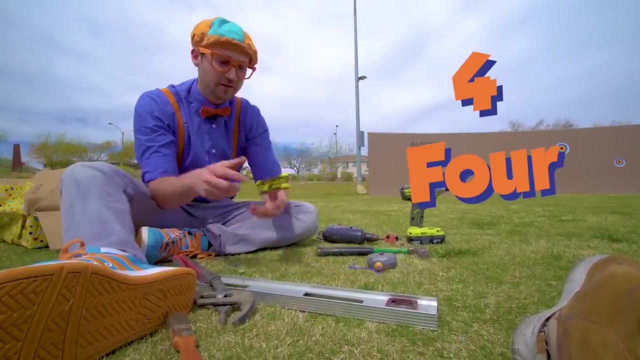 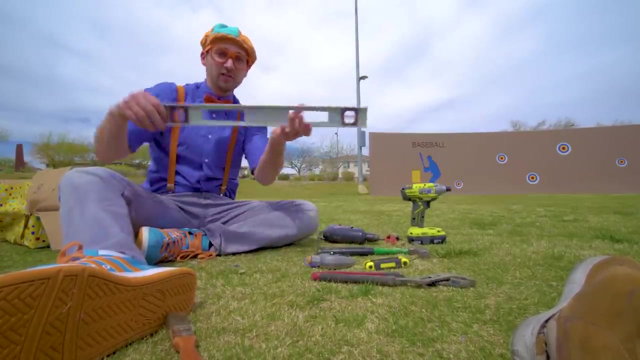 We have a second tool, which is a hammer. So we have a hammer, a drill, another drill, which is number three: One, two, three, chalk line, four, ooh Allen wrenches, five pliers, six, a level. 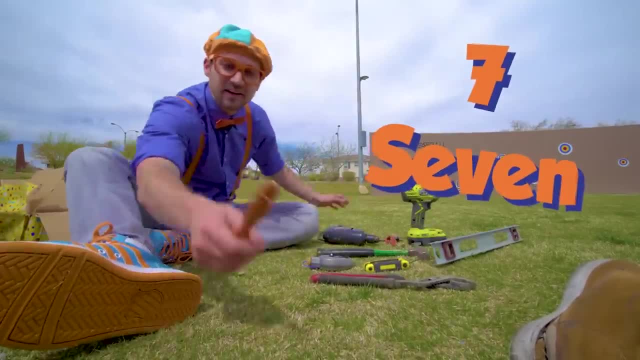 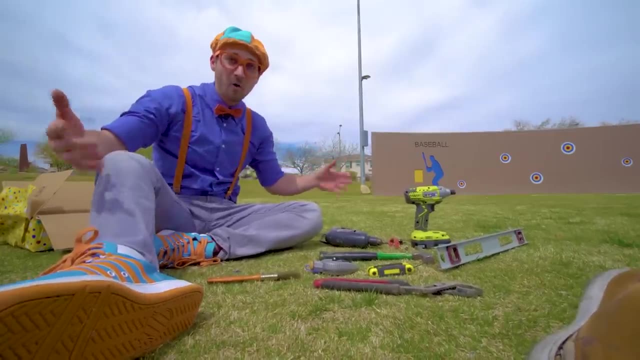 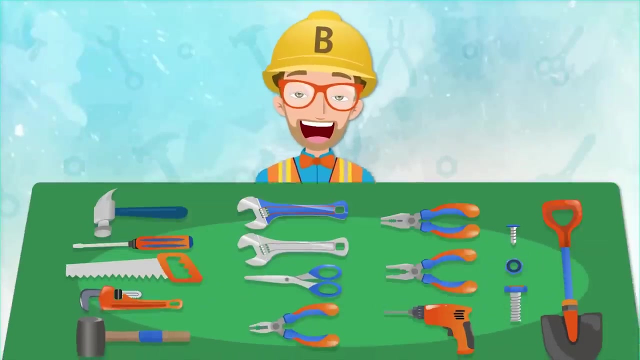 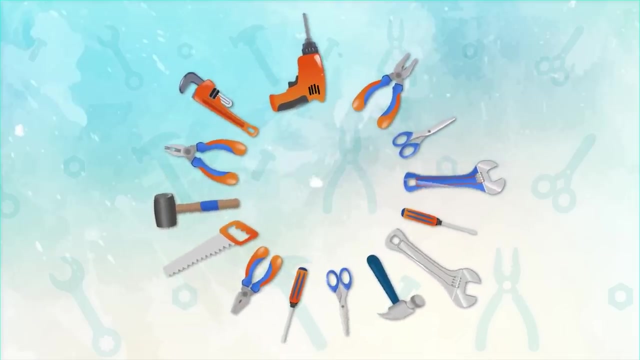 Whoa Seven and a paintbrush. Woo hoo, Eight, Whoa. This is the perfect time for the Blippi Tools song. When you're working with tools- working with tools- you hear all kinds of things. When you're working with tools- working with tools- you hear all kinds of things. 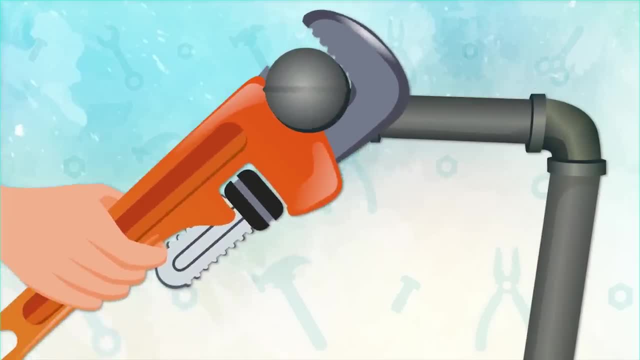 The wrench tightens, pipes go in. clang clang, A hammer hits the net, a hammer hits the big какая. You hit the otheroply too. Maybe pull down the bucket? No, you wouldn't. I get better this time. I don't want to have to fly. 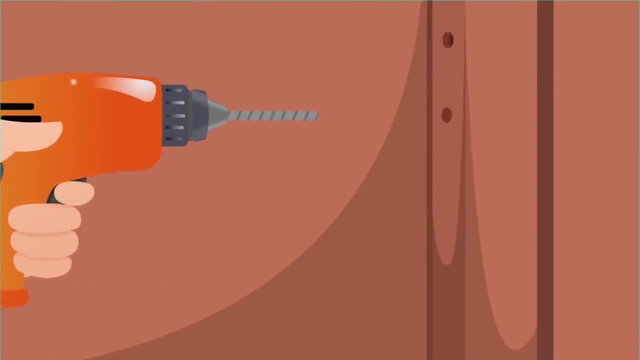 Benor likesnehmen. Are you ready to play The Life of Years 1?? I'm ready. I can't believe I've survived the first triple pot, but I'm going to have to play the second triple eating challenge. nail going bang, bang, bang. A drill is making holes going zzzz When you're working with. 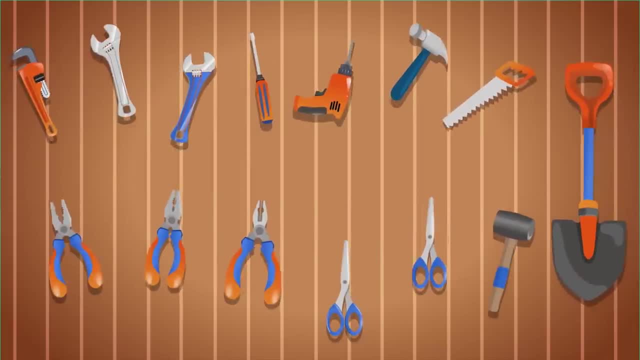 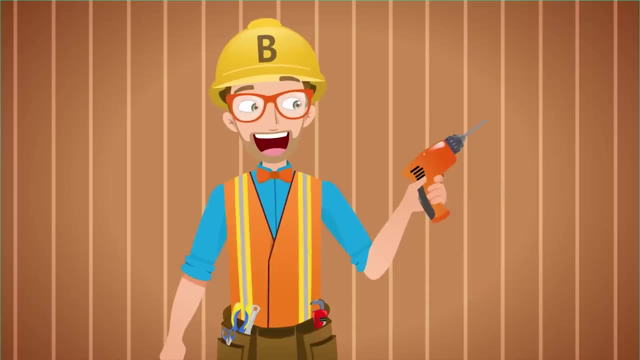 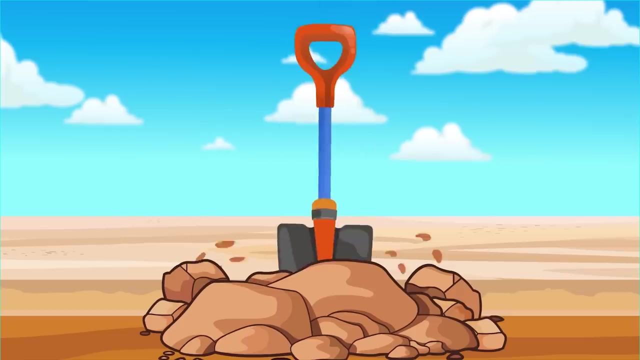 tools. you hear all kinds of things When you're working with tools. working with tools: you hear all kinds of things When you're working with tools. working with tools: you hear all kinds of things. You hear thuds and squeaks, cracks and rings When you're working with. 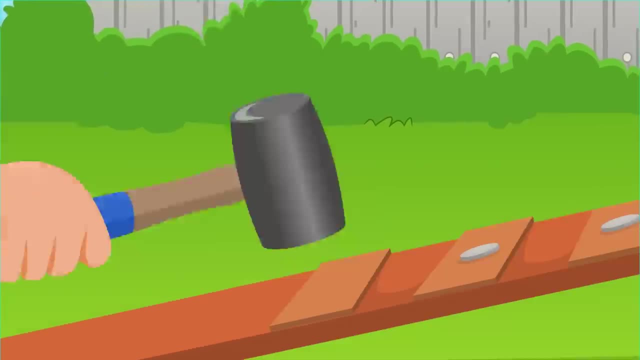 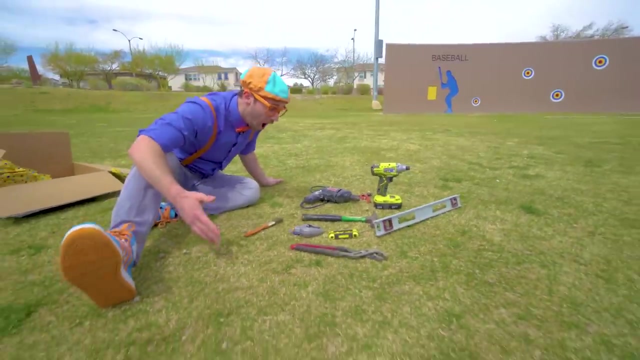 tools, you hear all kinds of things. You hear bangs and booms, clangs and zzzz. When you're working with tools, you hear all kinds of things. Whoa, I love tools. Oh, that fell One, two. 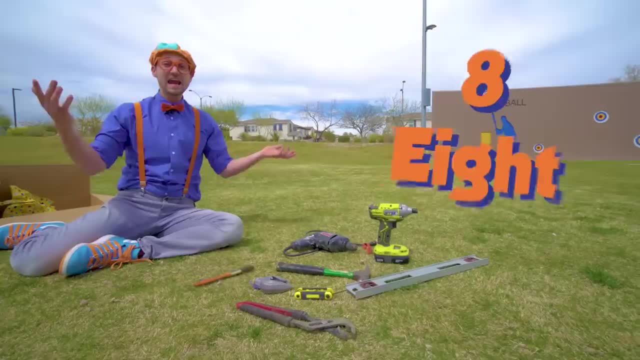 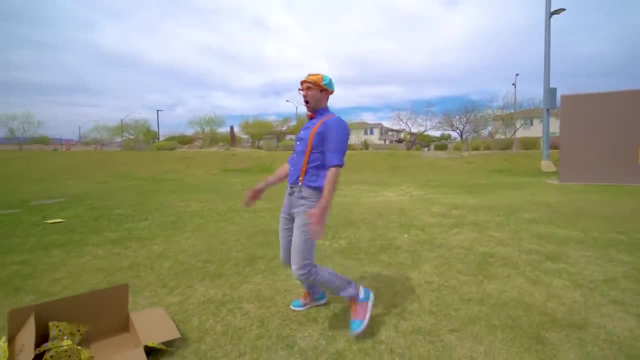 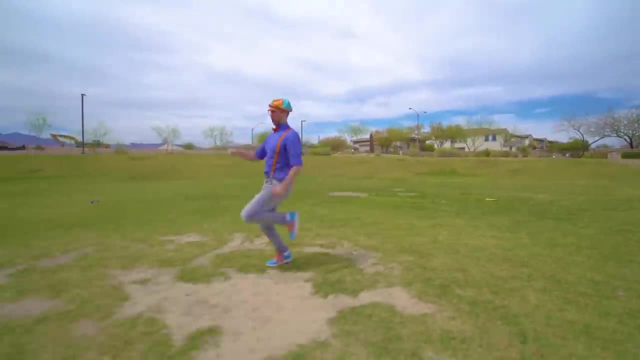 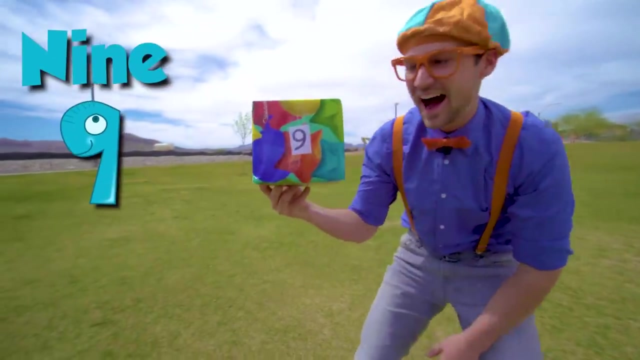 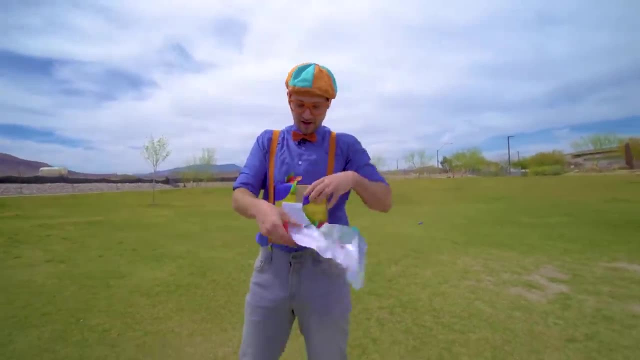 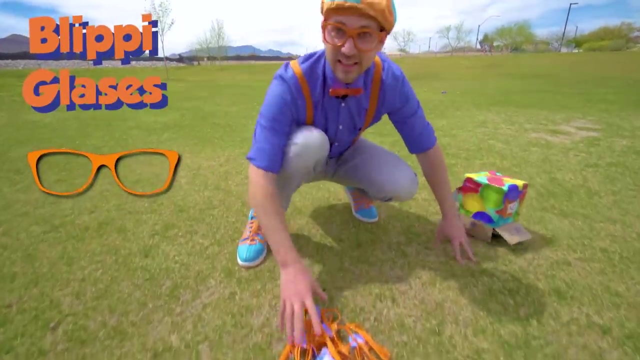 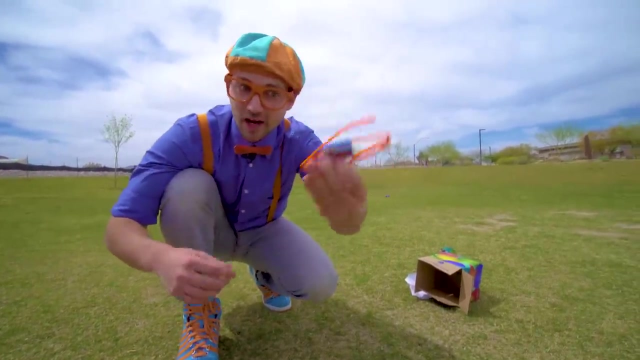 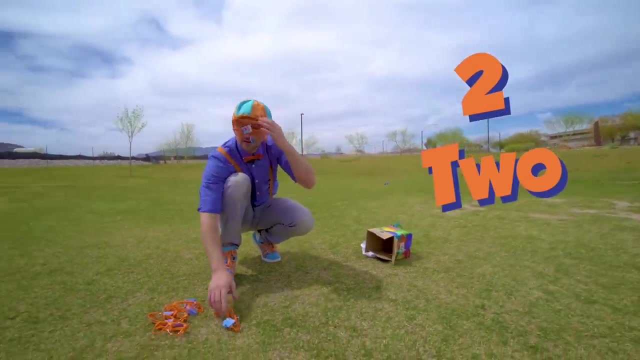 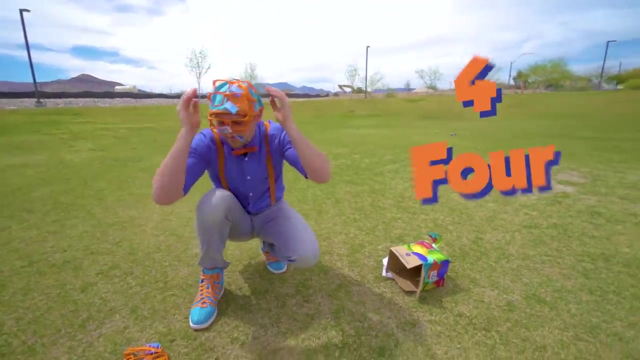 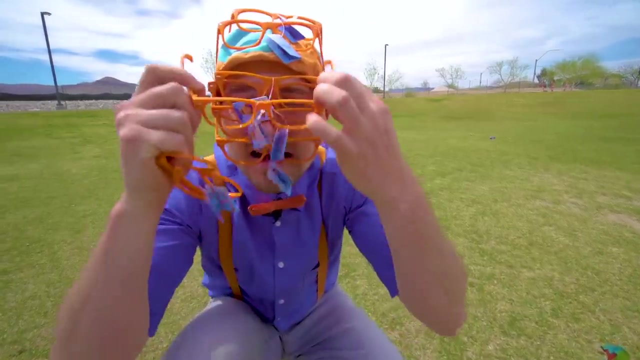 inside. I think there's nine things of these. Whatever it is, Whoa, Whoa Flippy glasses. Alright, there's nine of them. You know what we have to do. We have to try them on. So one, two, three, four, five, six, seven. 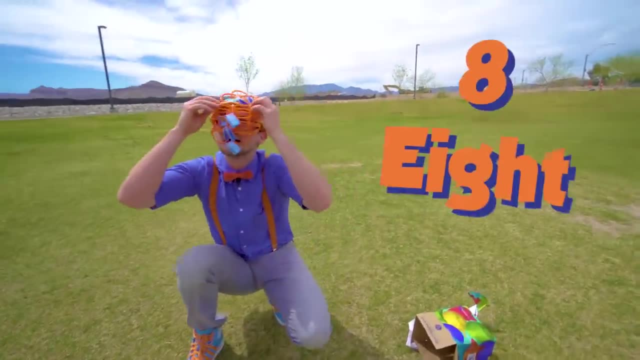 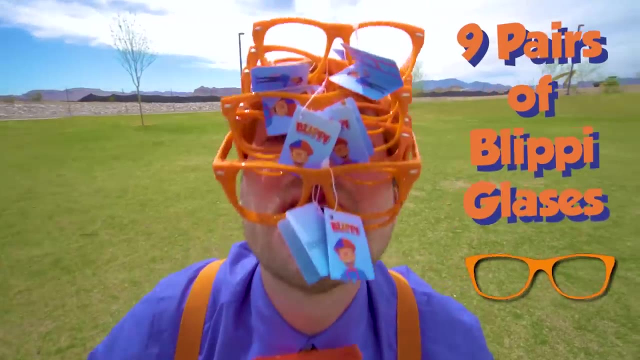 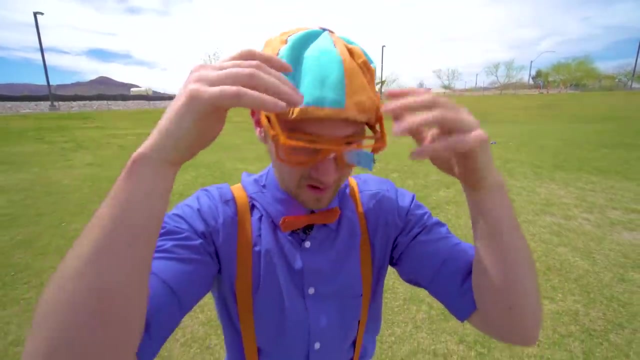 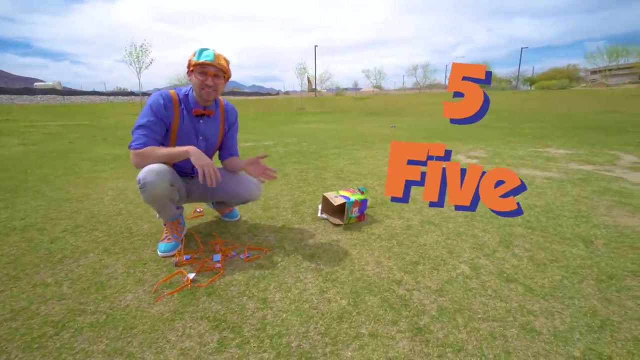 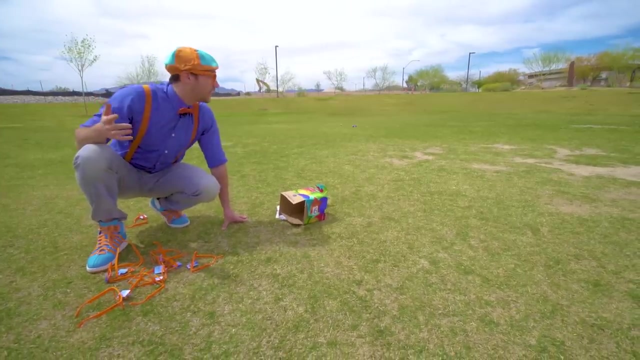 eight. I can't see, I can't see. Eight, Okay, Nine, Nine pairs of blimpy glasses: One, two, three, four, five, six, seven, eight, nine, All right, Now we need to find the next number. I see the last package. Let's go. 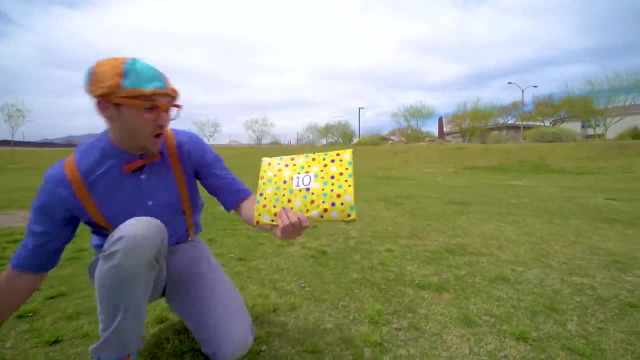 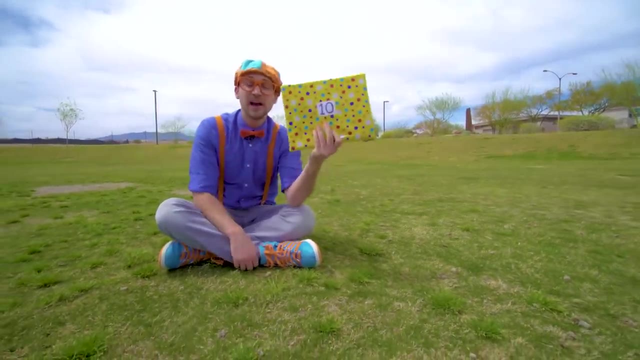 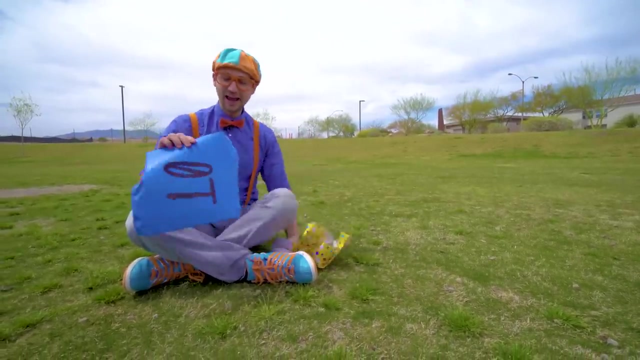 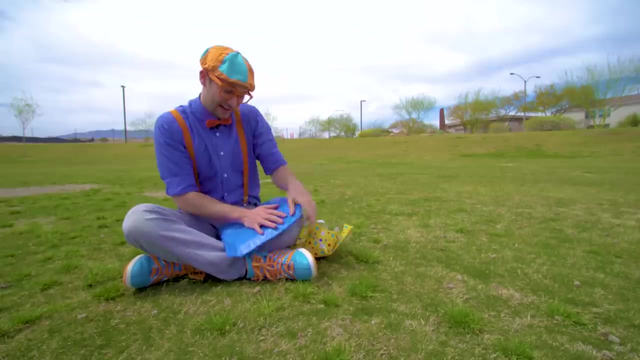 Yeah, The last package. Whoa, I am so excited to see what's inside. And it has the number 10 on it. All right, Let's open it up. Oh hey, A package with the number 10 on it. Huh, I wonder what's inside. I'm so excited. 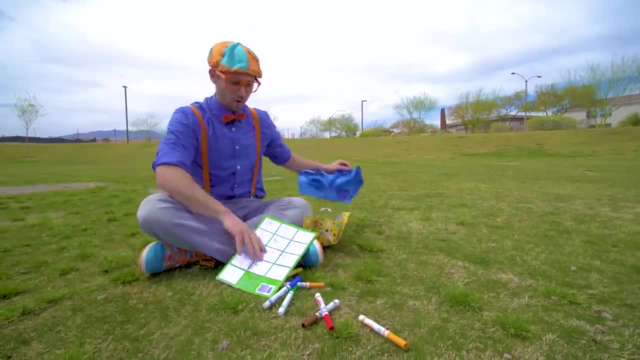 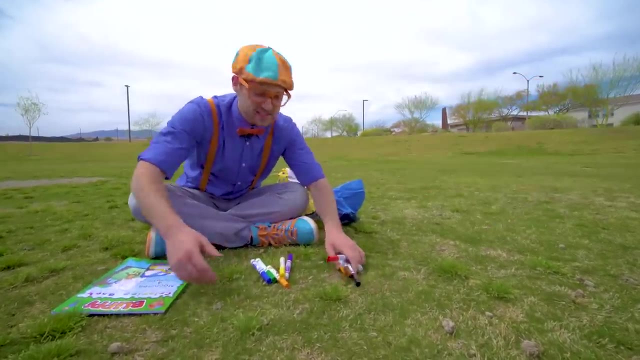 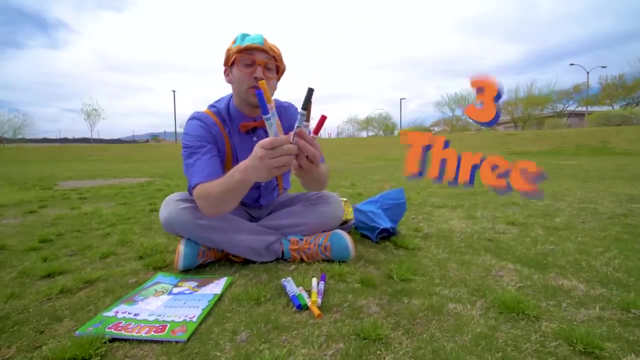 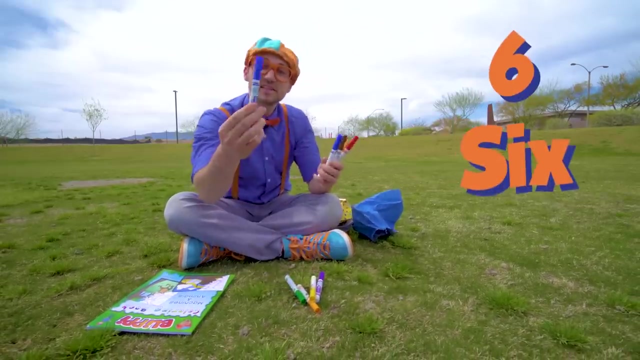 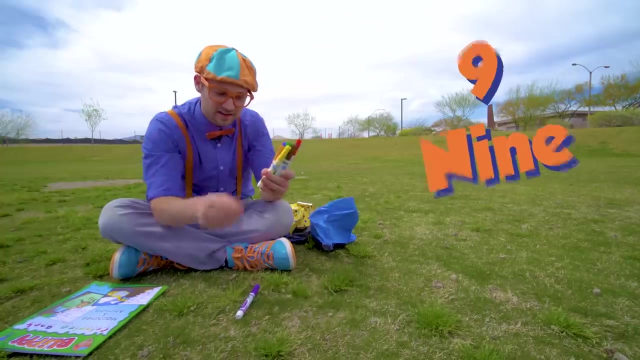 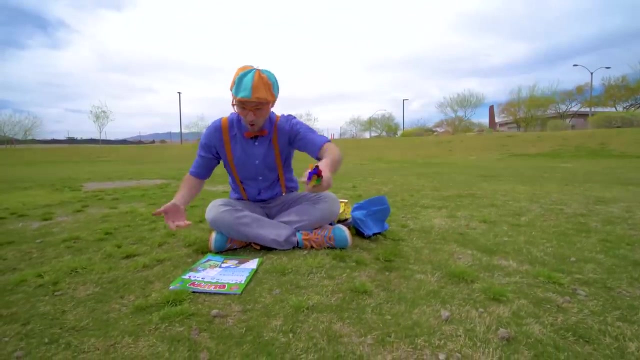 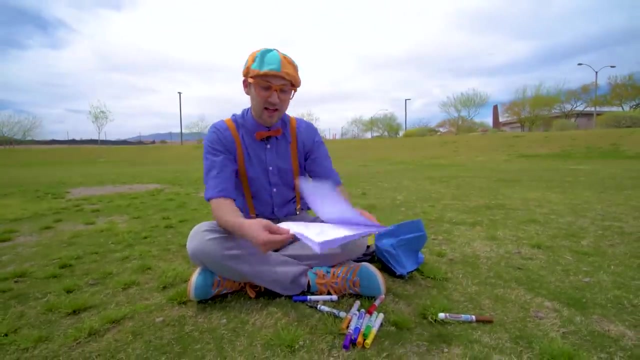 Open up the blue package. Whoa, Look at that. A bunch of markers. Oh hey, And there's 10 markers. Okay, One, two, three, four, five, six, seven, eight, nine, 10.. Whoa, 10 colorful markers. So color. Wait a second, I didn't even see this. It's a blimpy coloring book. I think we should color a page. Let's color the 10th page, Okay. 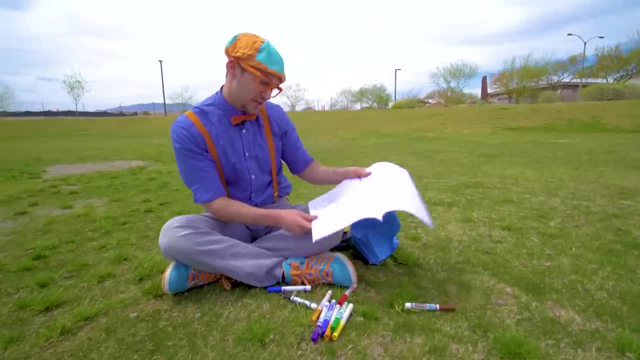 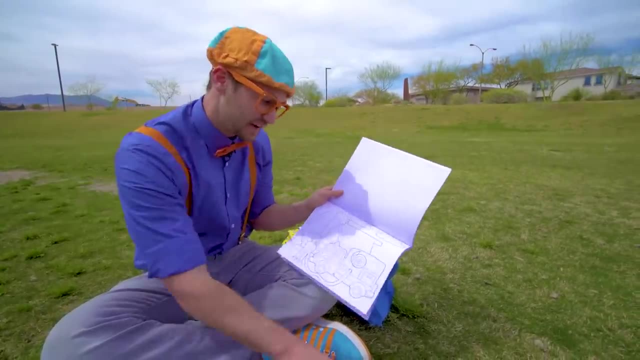 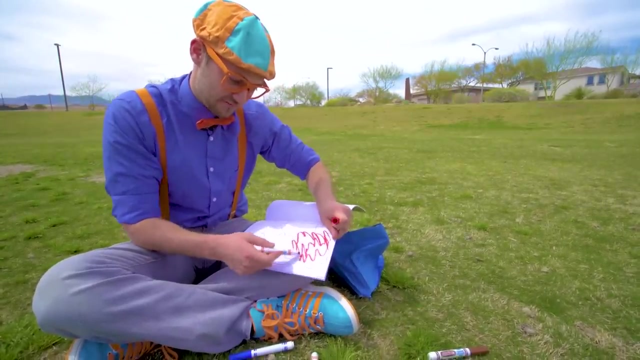 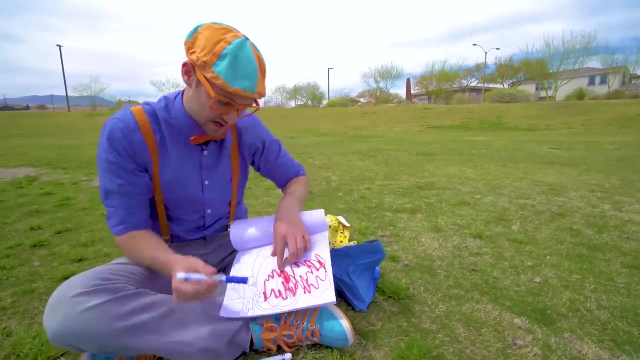 All right, Looks like the 10th page is blimpy Me spraying water on a house with a fire truck. to save it, All right, Let's make the fire truck red. Okay, Nice red fire truck. There we go. Oh okay, Nice red fire truck. And then, ooh, my shirt can be the color blue. 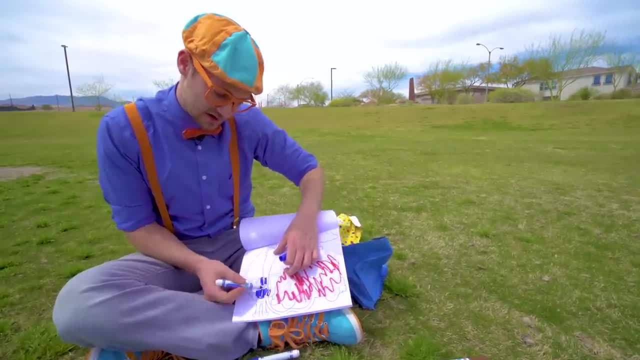 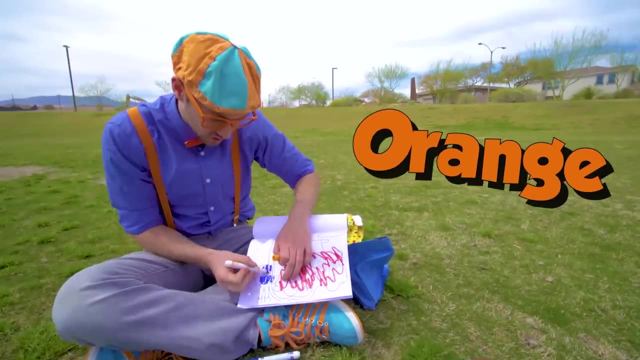 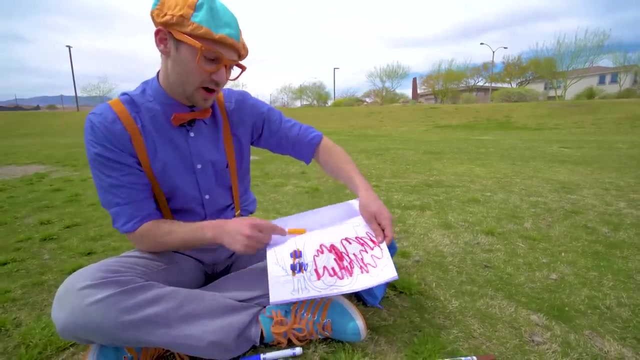 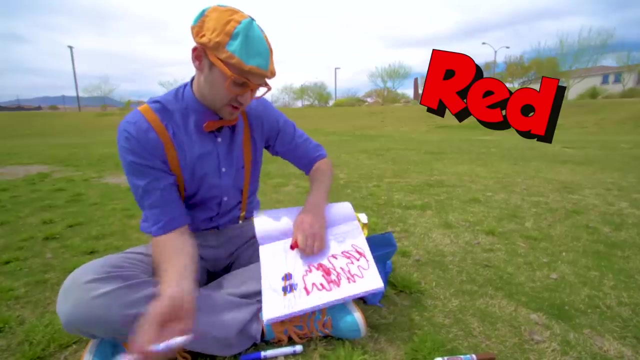 Okay, and my hat can be blue. Yeah, and my suspenders and hat is also orange. Perfect, look, it's me spraying water on this house that is caught on fire. Okay, fire is the color red, so let's color the fire. 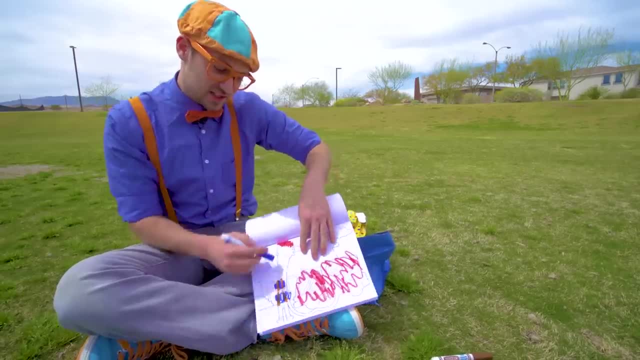 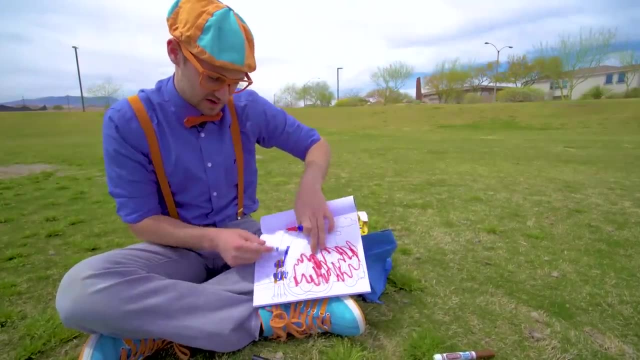 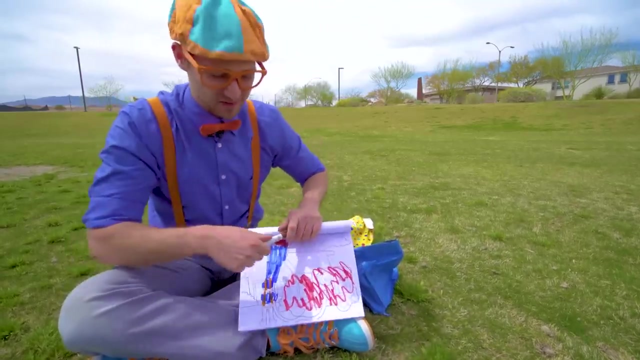 Whoa and we need to save it with the water spraying, So let's color it with blue, All right? oh yeah, we saved the house. woo, hoo, hoo hoo. Let's color the house real quick with the color whoa. 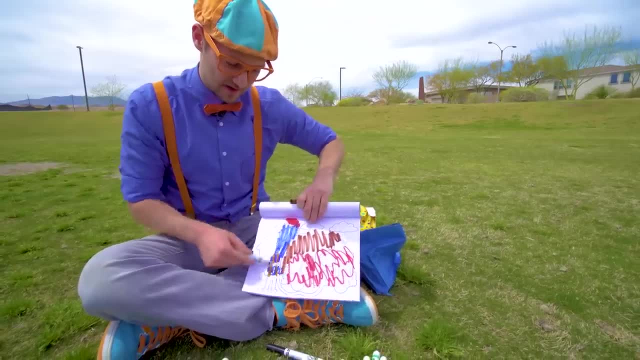 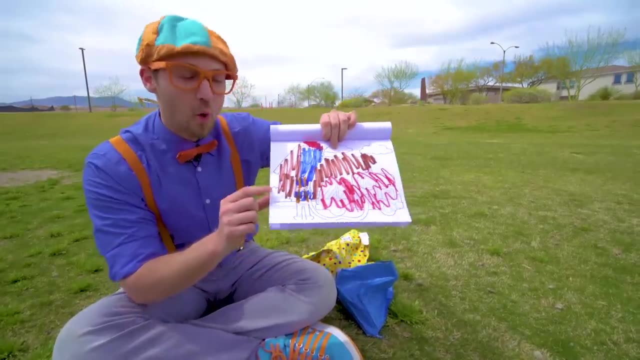 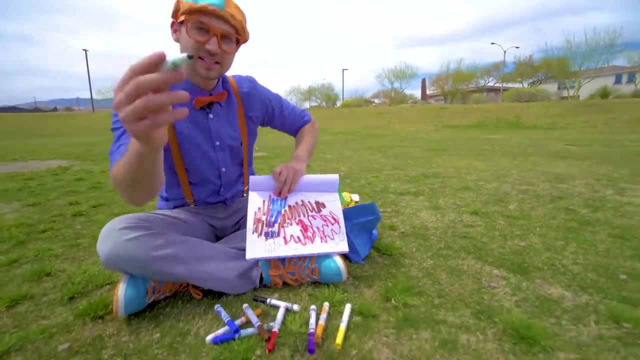 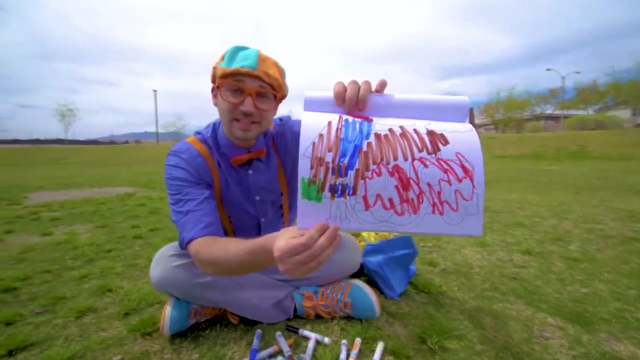 Brown, it's a brown house. How about that? whoa, look at that. that's so beautiful, Ooh. one last thing to color: Nice lush plant right there. Okay, that's the color green, Perfect, wow, what a masterpiece. 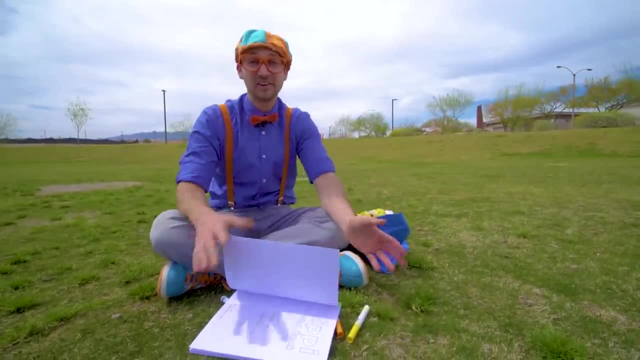 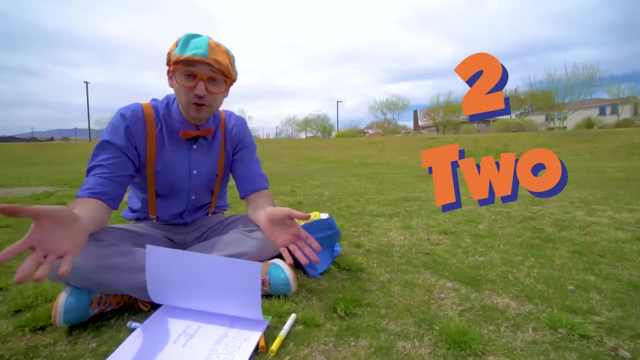 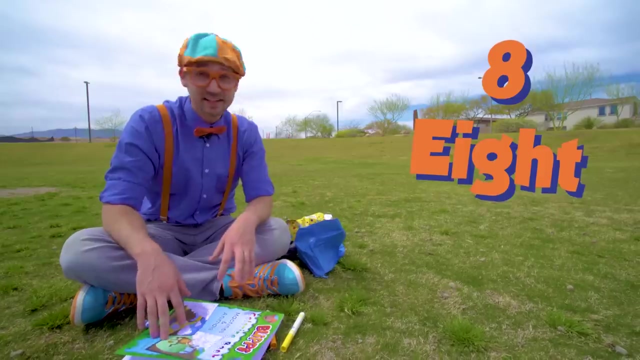 All right. well, this was so much fun learning numbers one through 10 with you. Let's recite them: one, two, three, four, five, six, seven, eight, nine, 10, whoa, will you recite them again with me? 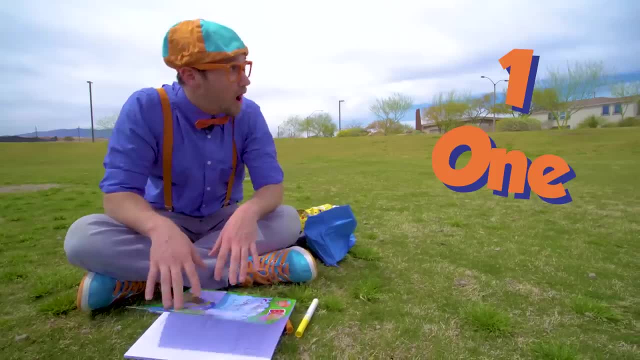 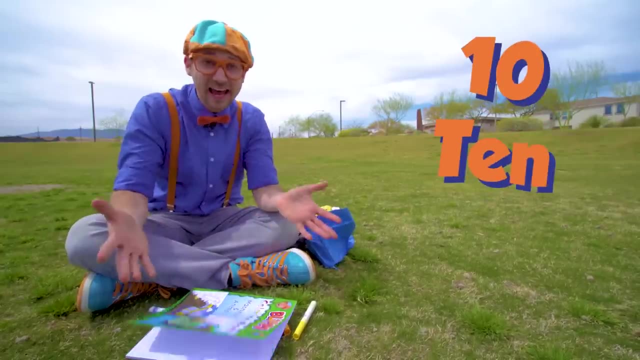 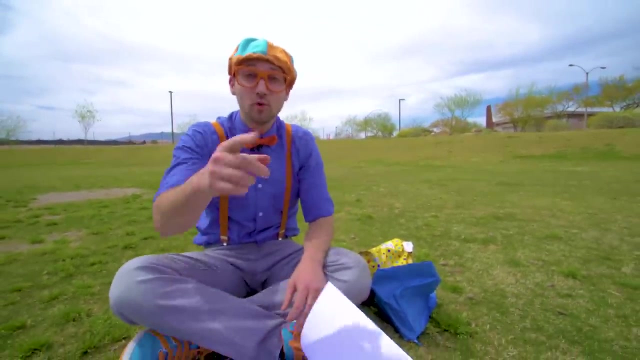 Okay, this time let's do it a little faster: One, two, three, four, five, six, seven, eight, nine, 10.. Yeah, all right. well, this is the end of this video, but if you want to see more of my videos, go to my website. 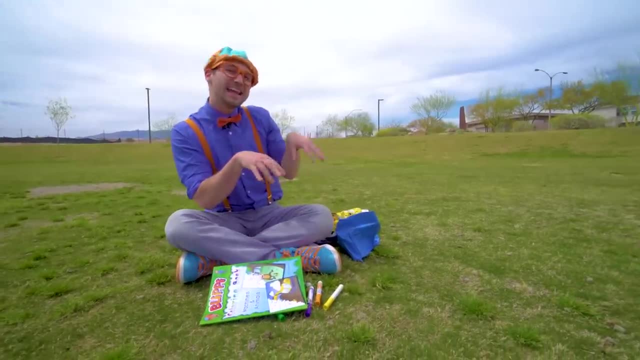 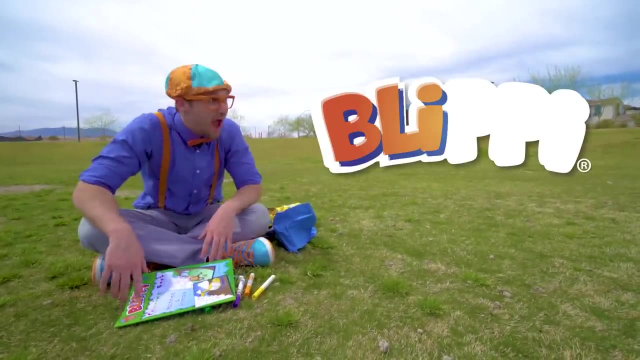 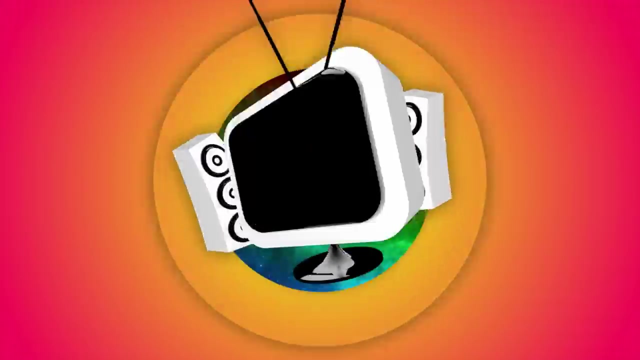 and you'll see more of my videos. All you have to do is search for my name. Will you spell my name with me? Ready, B-L-I-P-P-I, Blippi, yeah, see you again, bye-bye. So much to learn about. it'll make you want to shout: Blippi. 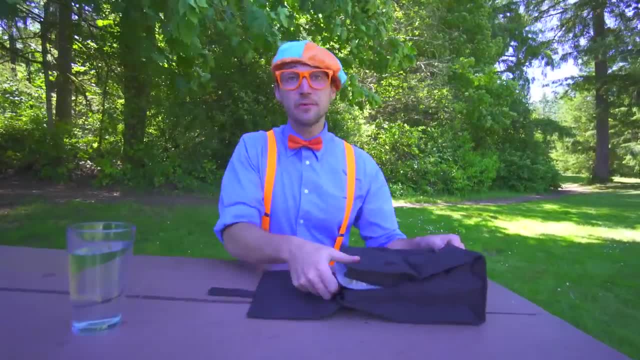 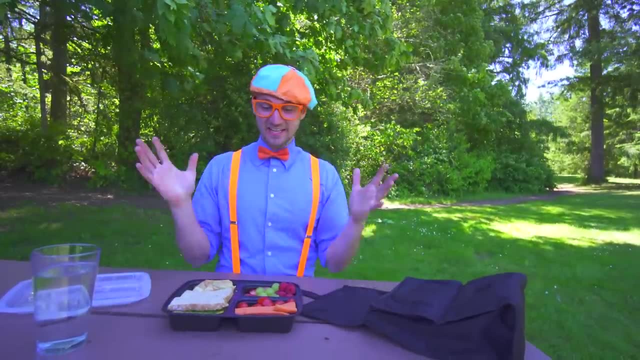 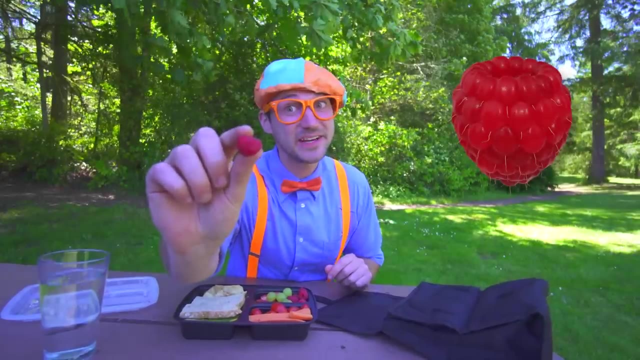 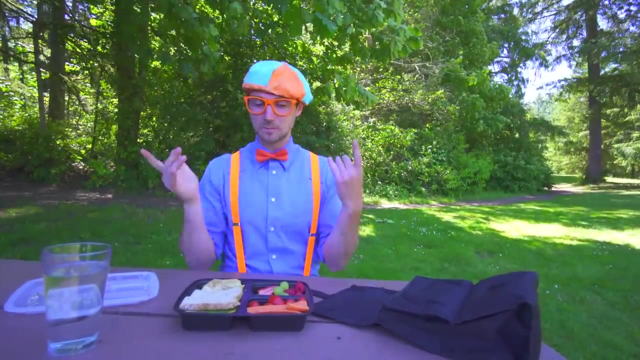 Hmm, hey woo, look at where we are. We are at a beautiful park And look at what we have: Yum, a tasty lunch, Like this grape, hmm, hmm. this raspberry, hmm, hmm, hmm, a red strawberry, hmm, and we have some vegetables. 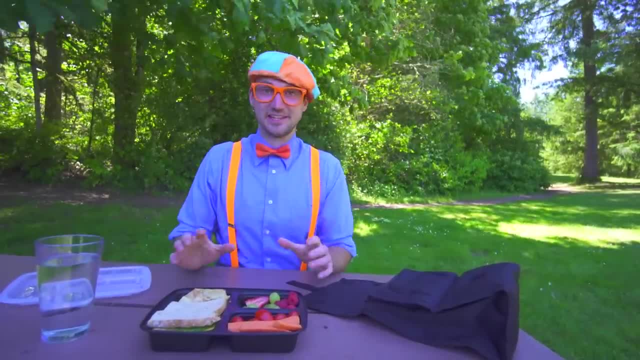 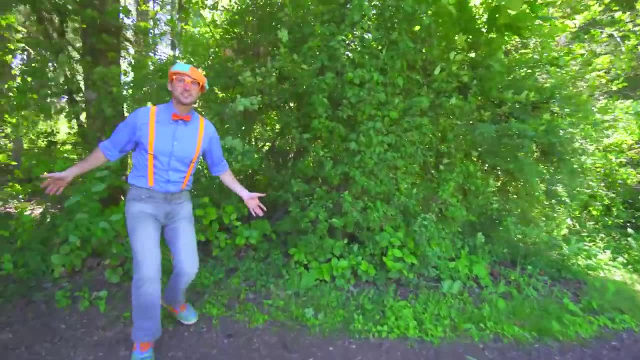 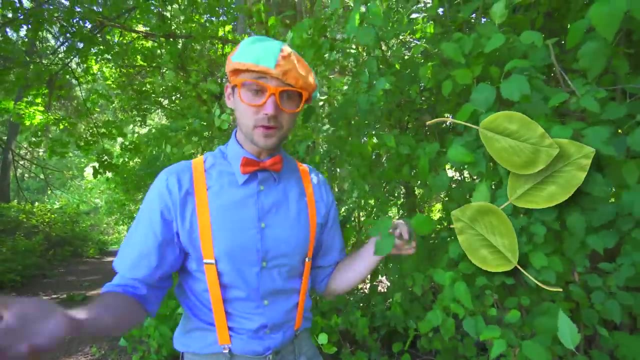 a sandwich crackers. but we'll get to this in a little bit. Let's go play first. come on. Wow, this park is so beautiful, Like these plants. they just look like plants, but they're so beautiful to me. 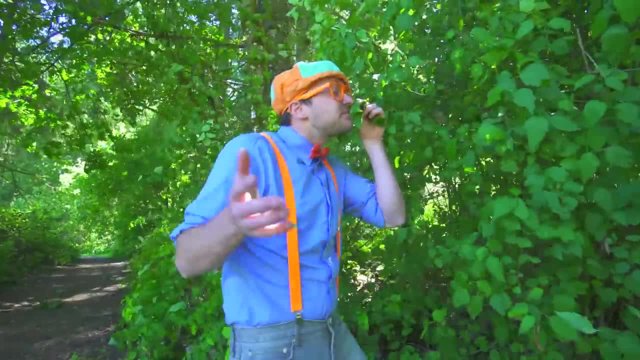 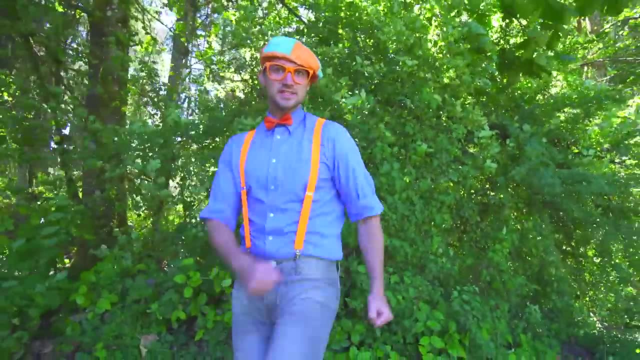 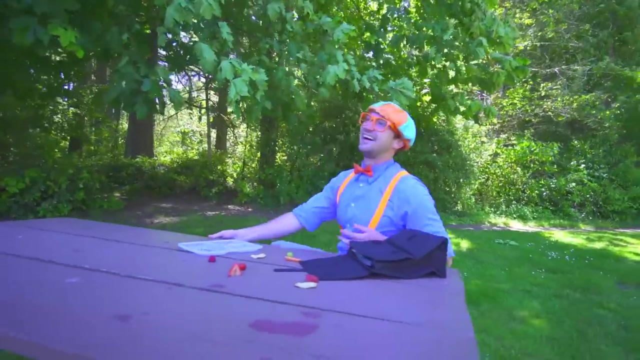 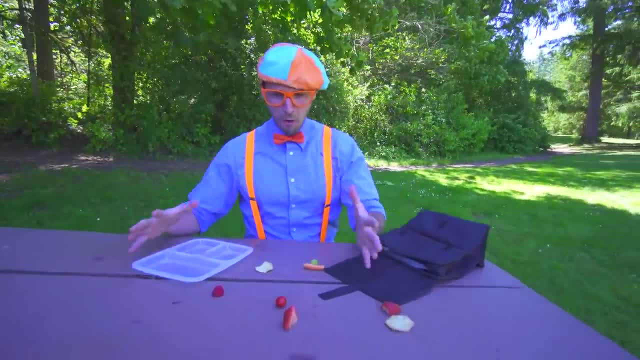 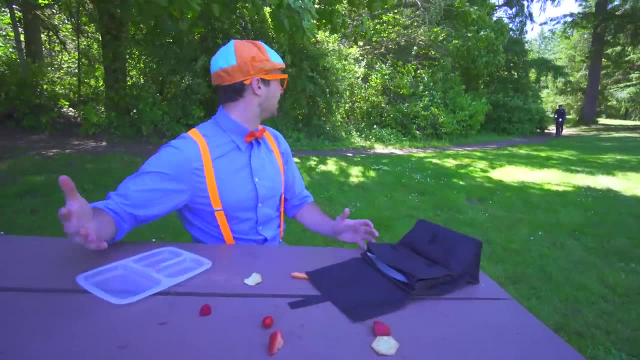 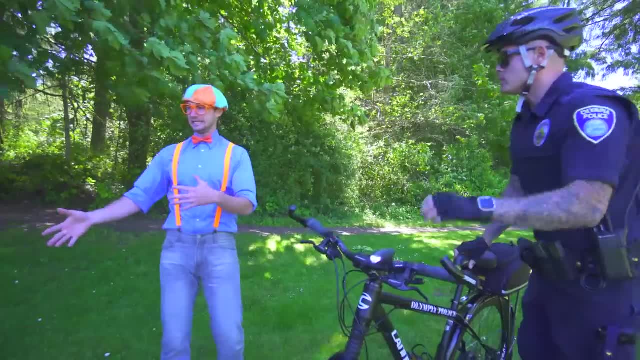 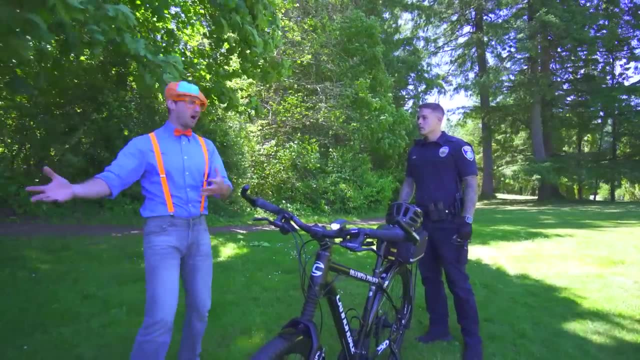 What's going on? My lunch was just right here. I was eating it and it was so good. And then I went over here and I looked at some plants and then I came back here and it was all gone. Well, it looks like we're gonna have to investigate this. 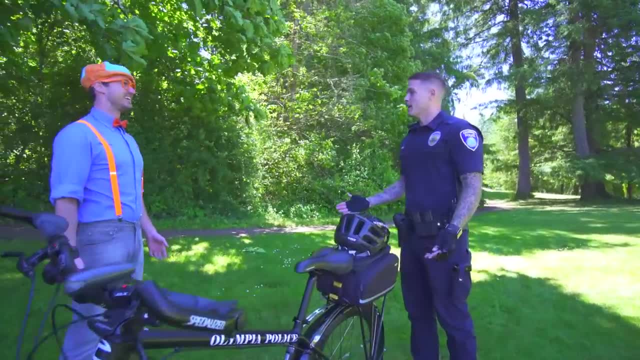 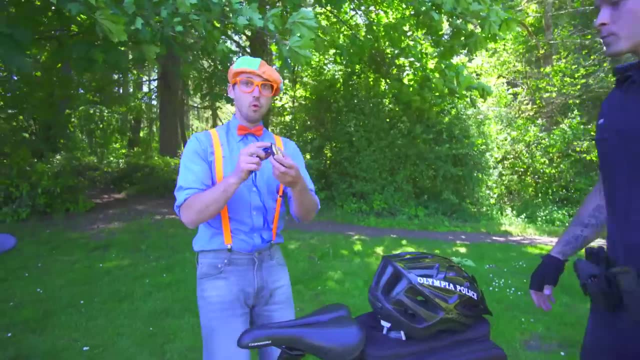 Lucky for you. crime scene bag with me. I've got a really good idea. Do you want to help me? Blippi, I would love to. yeah, Oh, I've got this special badge just for you. Whoa, Wow, look at that. It even has my name on it. 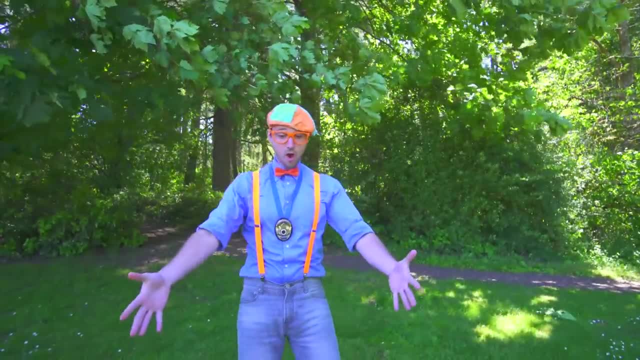 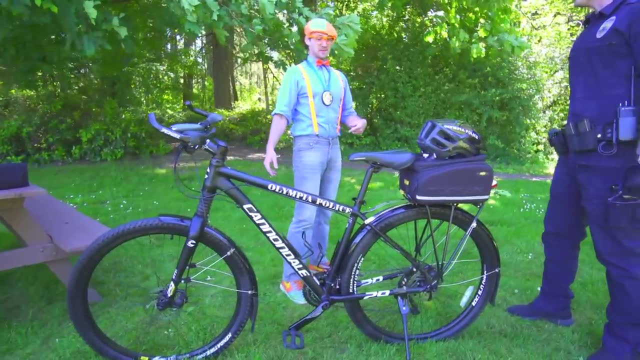 Whoa, I am honored, Whoa, and look at what you rode up on A police bicycle. Can I look at it? Of course you can. Blippi, Oh, cool, Okay, Look at this: a helmet, Wow. 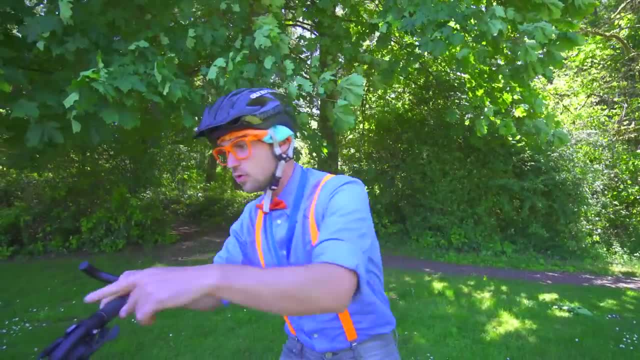 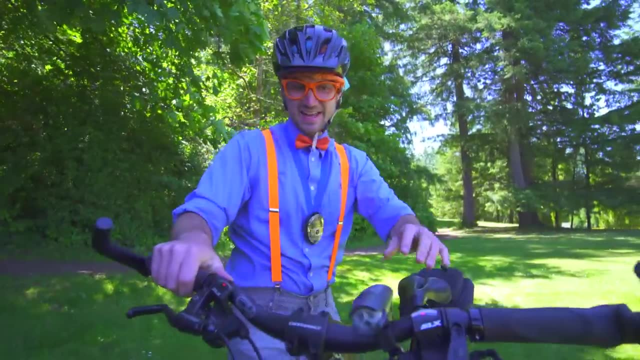 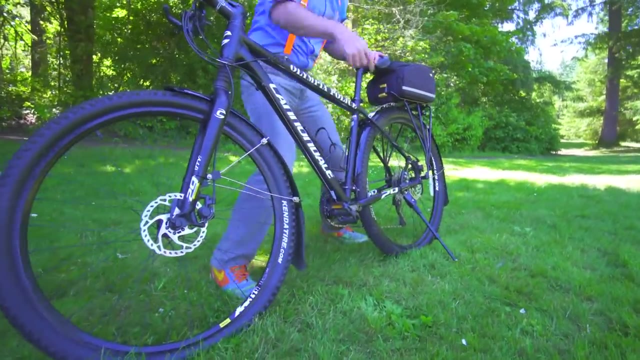 this keeps you nice and safe. Okay, And oh, look up here. Do you see that? It's a light And the handlebars And one big giant wheel and tire, And then a second big giant wheel and tire. 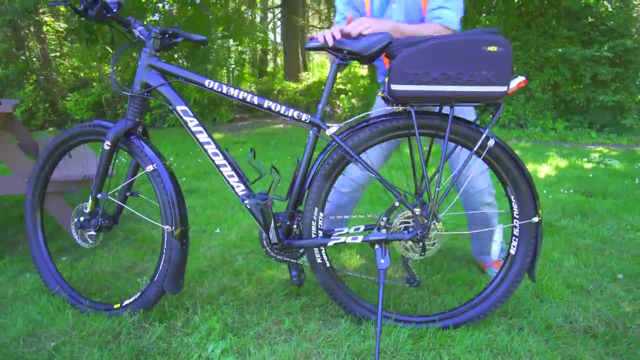 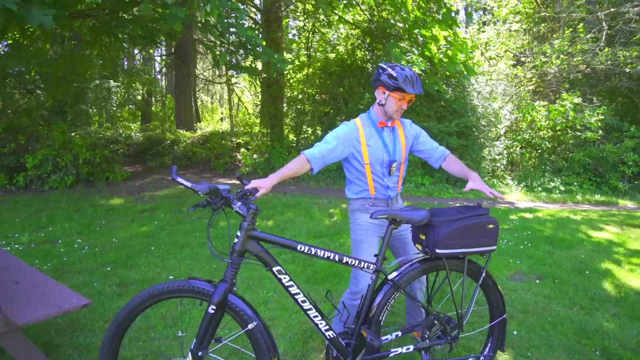 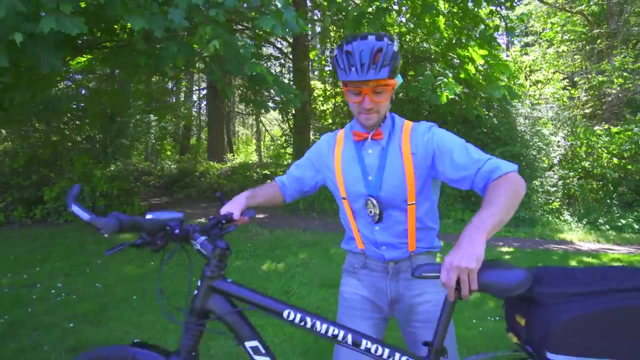 And then we have the pedals and the A kickstand. Let's put that up right now. Yeah, and look at this. This is the crime scene investigation bag. he said This is going to help us find my lunch, But first let's take it for a ride. 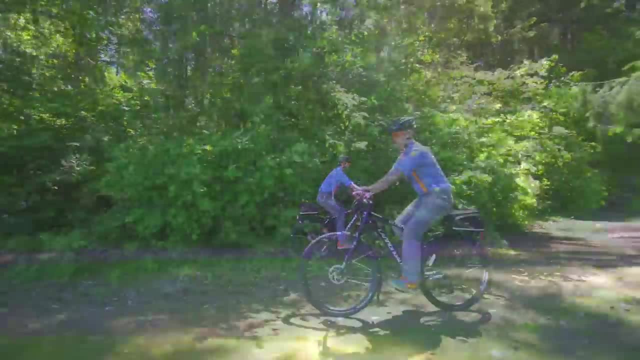 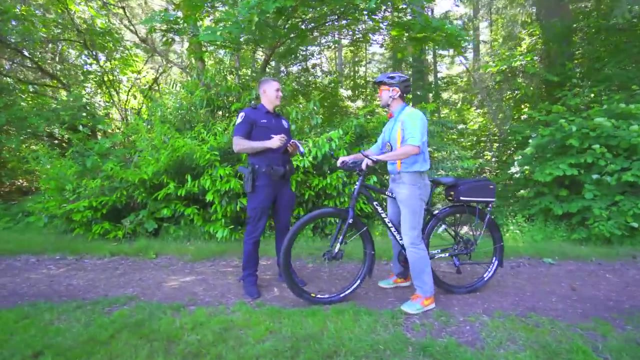 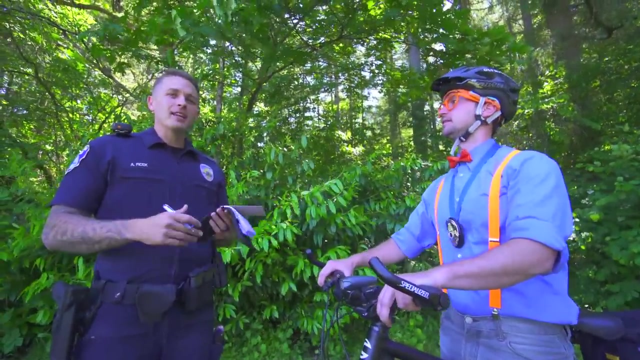 Whoa, that was so much fun It is, isn't it? Blippi? Yeah, Well, I think we should get started on the investigation. What do you think? Yeah, I think so too. All right, I think the next best thing, send in the canine. 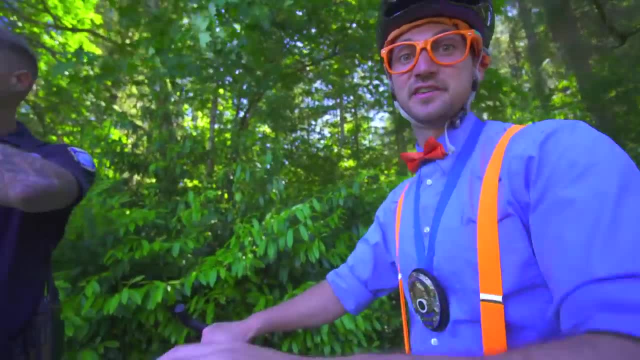 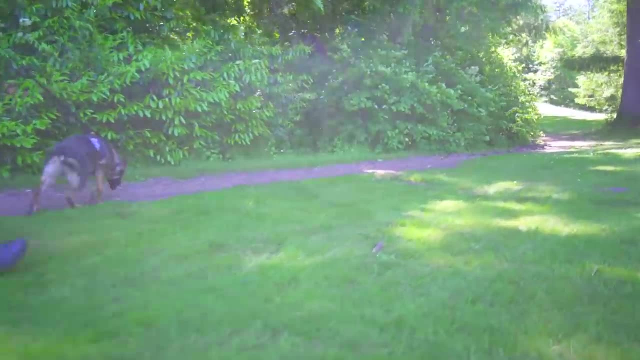 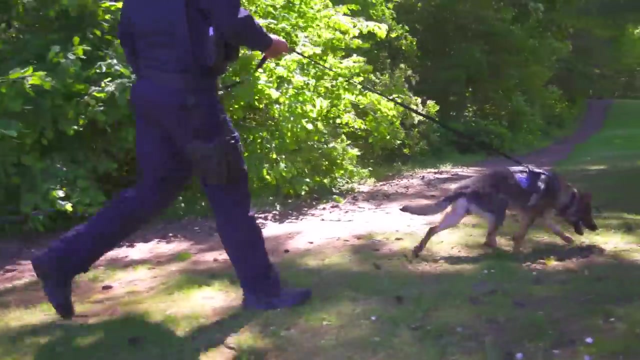 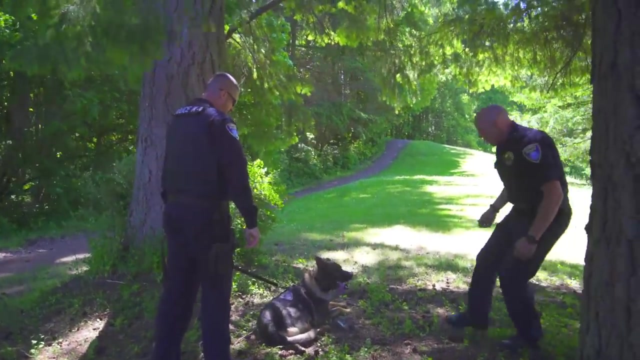 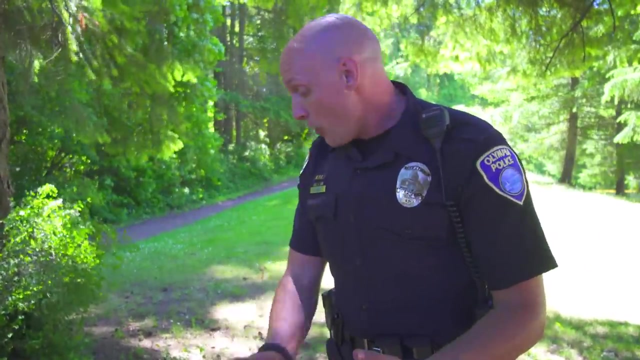 Ooh, canine, That's another word for a dog. Officer Fechek, send in the canine. Whoa, he did it. Police dogs have really sensitive noses and police use those to help us track to people and evidence to help us with our investigations. 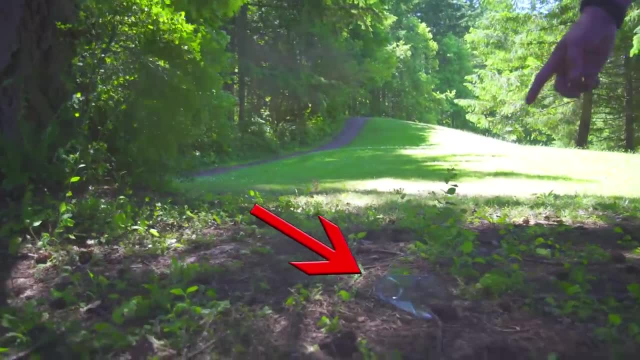 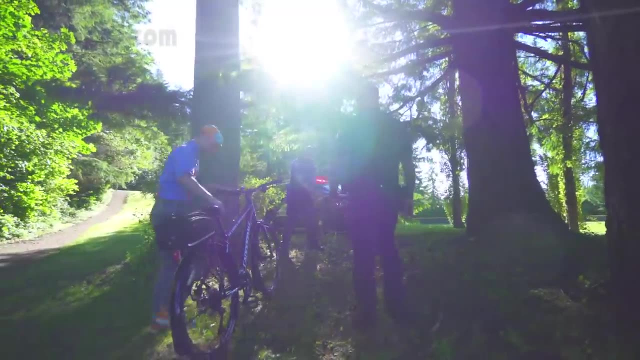 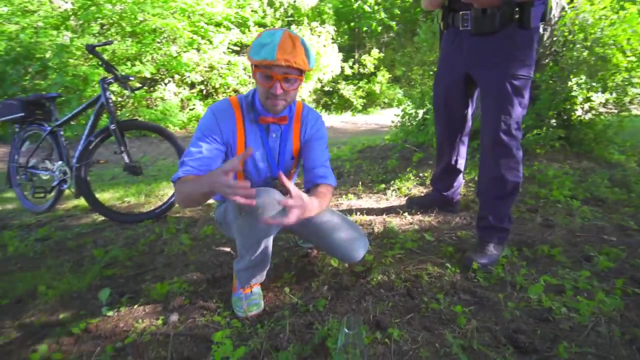 He did it. He found some evidence, Investigator Blippi, this is the evidence that the canine tracks to: Oh look, This is my glass. This is my glass that had all the water in it. What's it doing all the way over here? 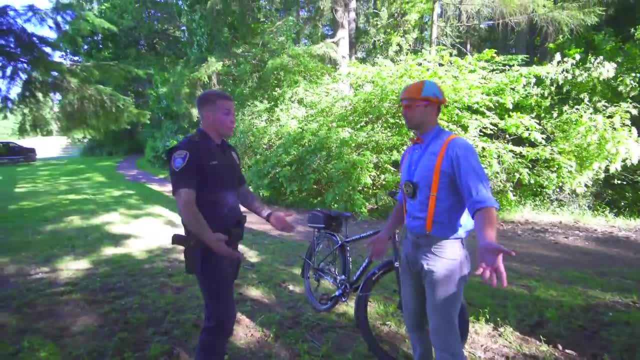 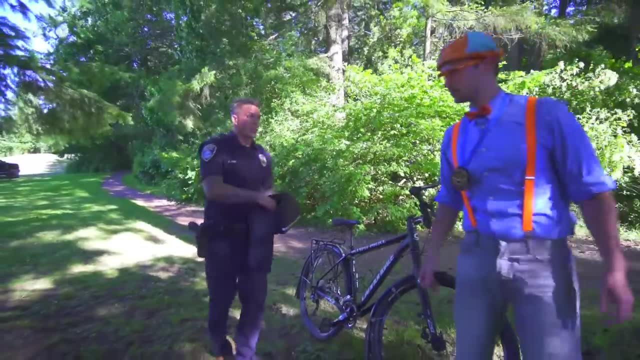 Huh, Well, there's the glass. What do we do? Well, we're going to have to collect the evidence using the bag that we talked about earlier. So the first thing that we're going to have to do is put evidence tape up to secure the scene. 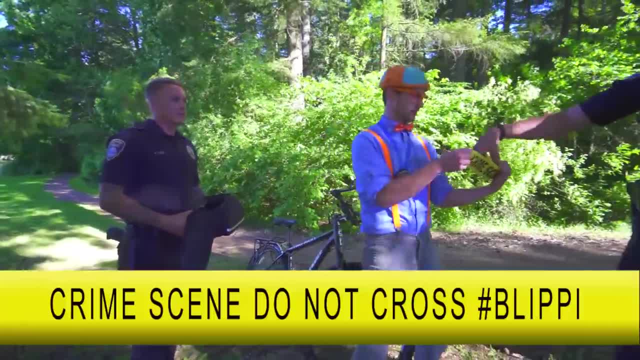 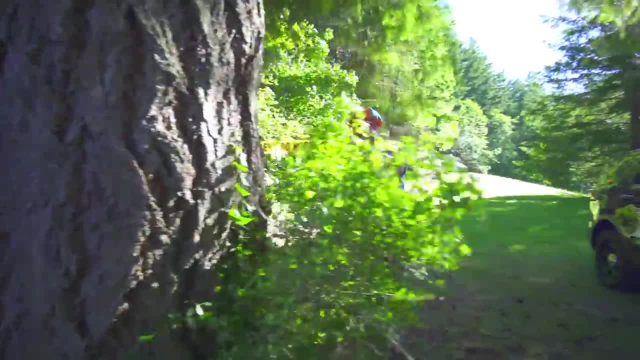 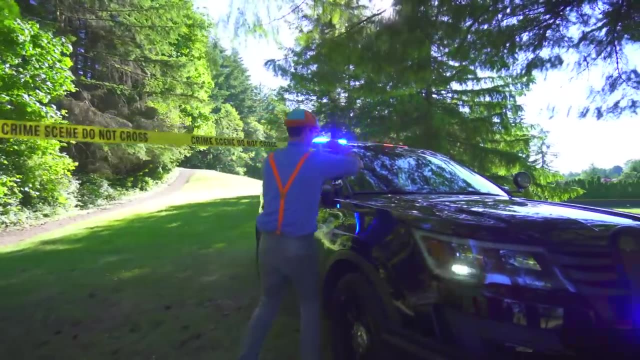 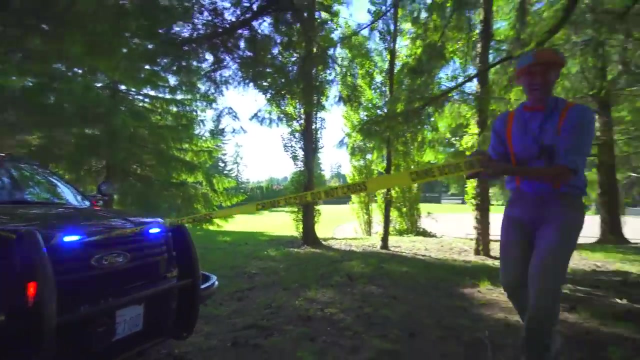 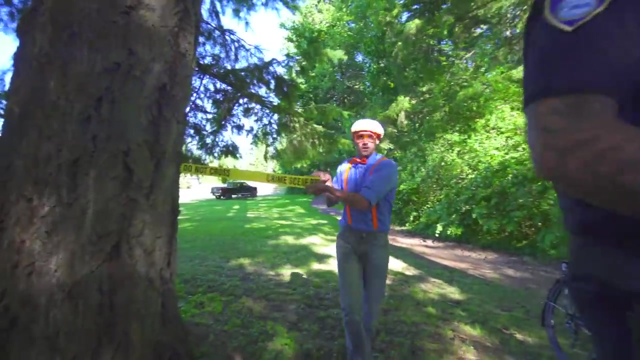 Okay, Ooh, thank you. Ooh Whoa, look, It says Crime scene. Do not cross. Whoa, Whoa, Let's go around the bumper. Whee, Whoa, Here you go And we can tie it off. 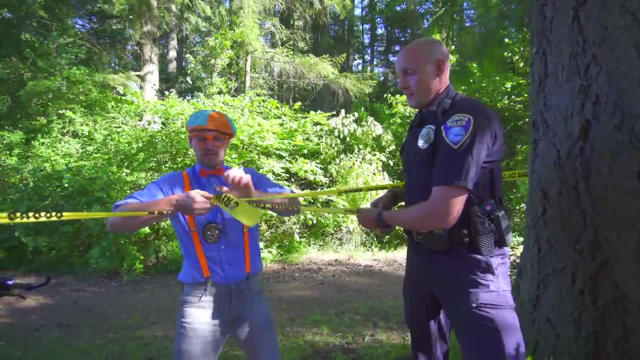 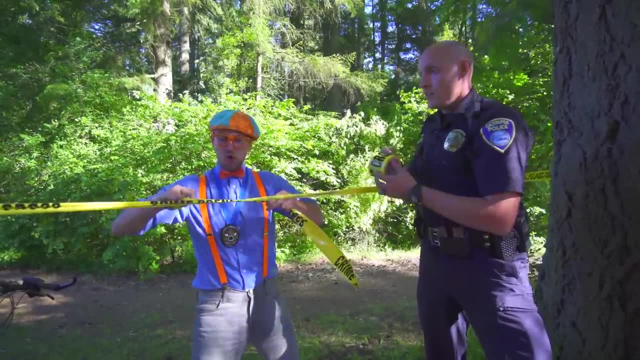 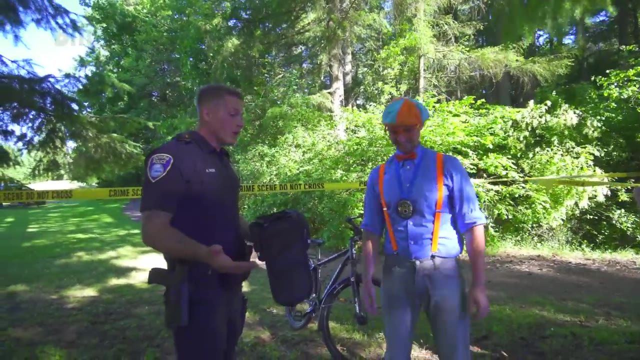 Okay, Let's tie it. Here we go. Oh, almost there. Oh, good job, Blippi, Thanks. Okay, It's nice and tied off. Now what? That was? a great job, Blippi, Thanks. Now we have to take pictures using a ruler. 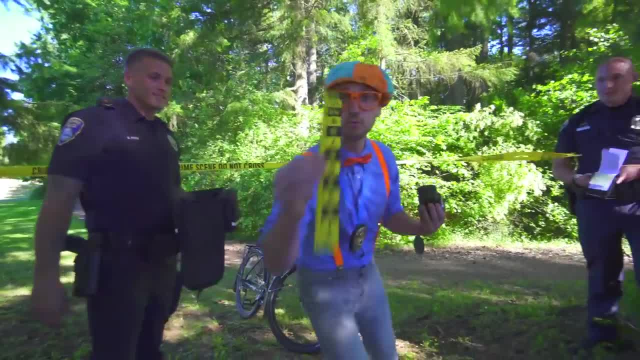 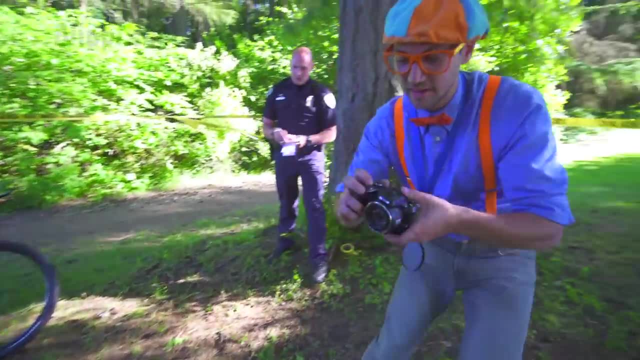 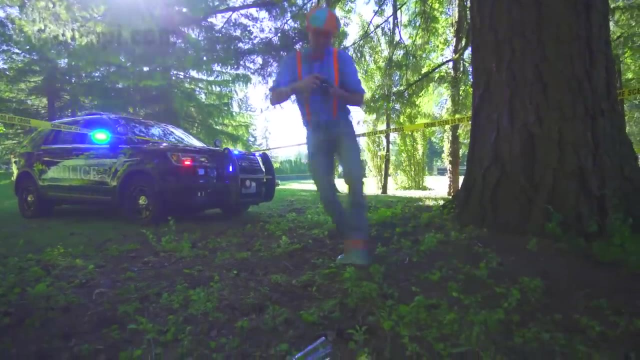 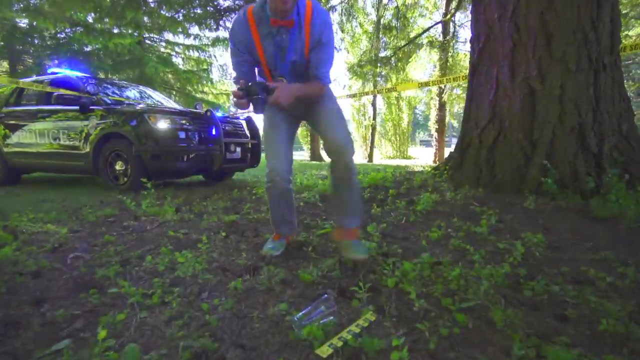 Okay, Hey, here we go. We have the ruler. Let's put this down right next to it. Then we have a camera. Let me turn it on. Ooh, Smile, Oh, you are so beautiful. Glass. Okay, close up. 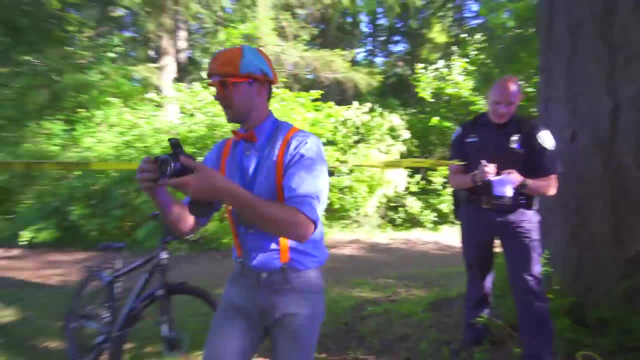 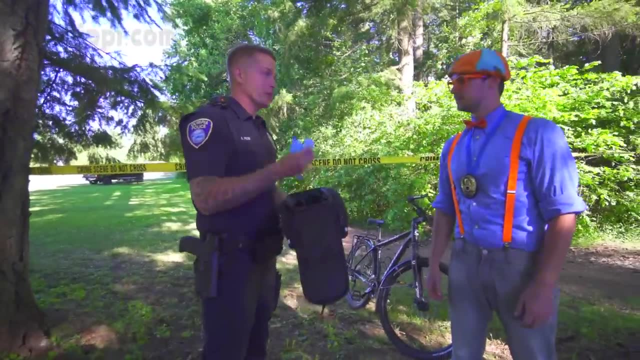 Okay, Turn that off And here you go. All right, So now that we have the markers, we actually have to collect the evidence. Okay, But before we do so, we've got to put gloves on, because we don't want your fingerprints. 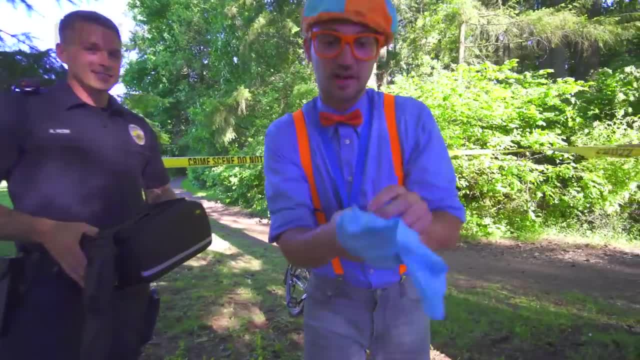 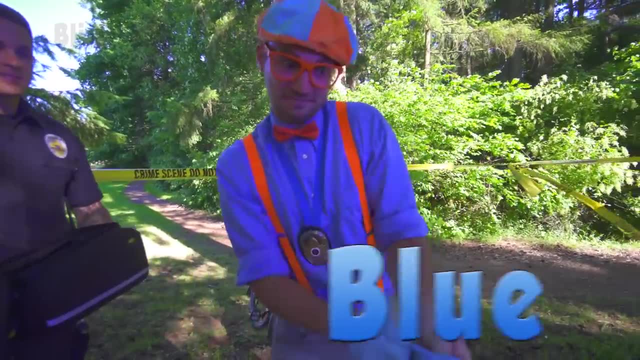 being on it, Right? Okay, So we have to put these gloves on, And this first glove is the color blue, And the second glove is also the color blue. All right, I've got the gloves on. Now what? Okay? 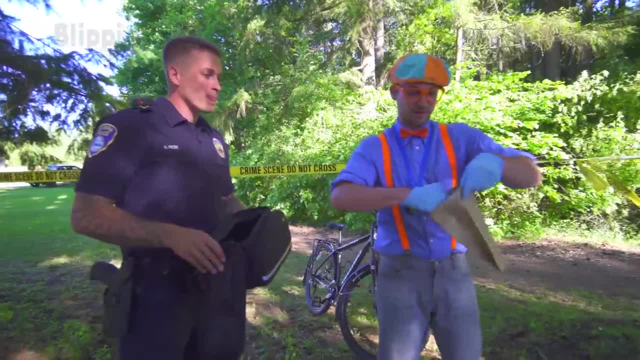 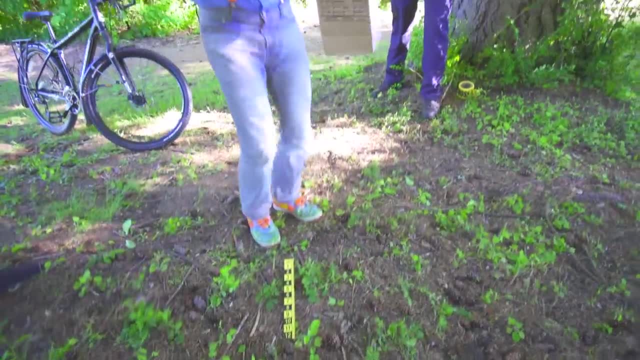 Now that the gloves are on, we can actually pick it up and put it into a bag. Okay, Ooh, Look An evidence bag. Okay, Here we go Pick it up. Wow, Ooh, Okay, Let's put it in the bag. 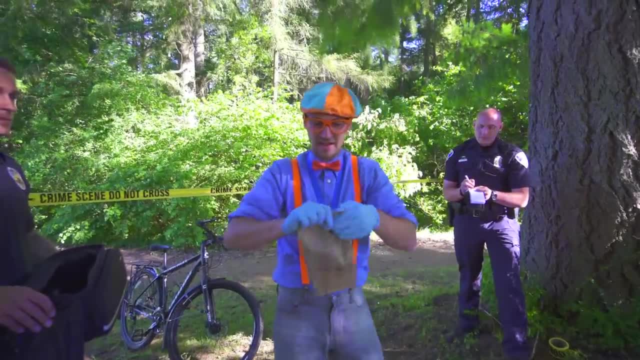 All right, So I got it in the bag. Now what? That was a great job. Now we have to get it down to the police department to process it, Okay, So how do we get it there? Well, we're going to have to call in the motorcycle. 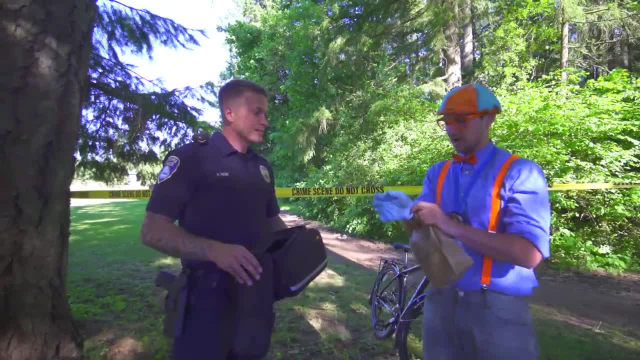 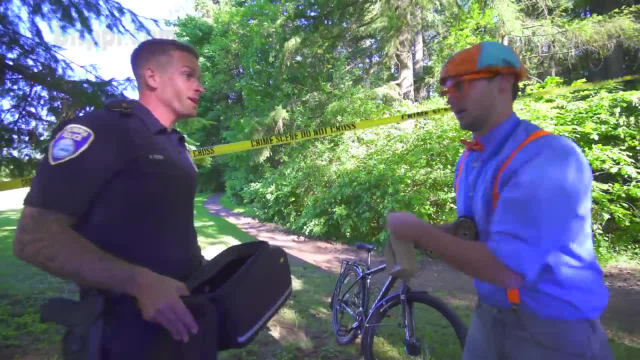 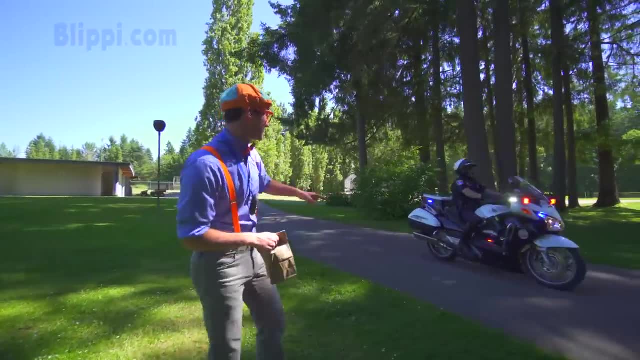 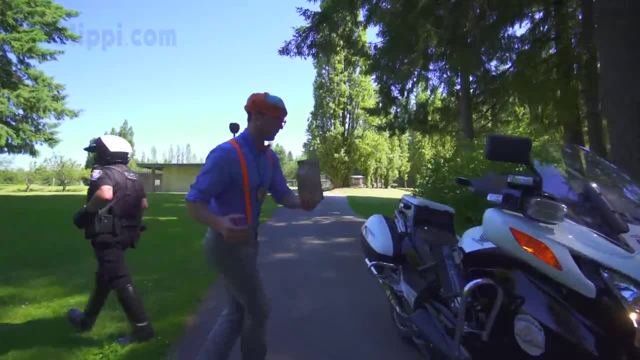 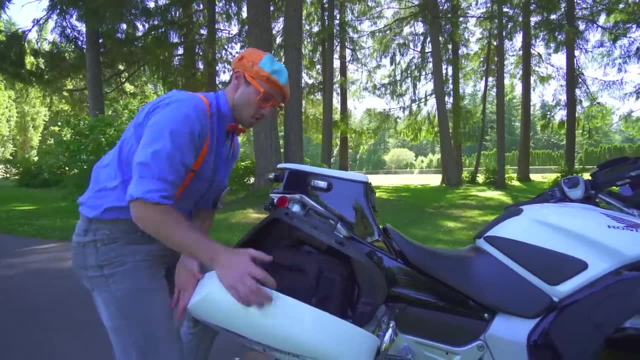 All right, Whoa, Look at what it is. Wow, It's a police motorcycle and this is what's going to be used to transport the evidence Here. Come here, Wow, Look at it. Okay, First things first, Let's put the evidence in the back of this motorcycle. 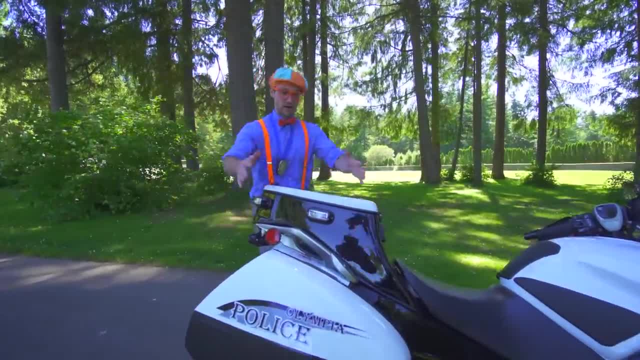 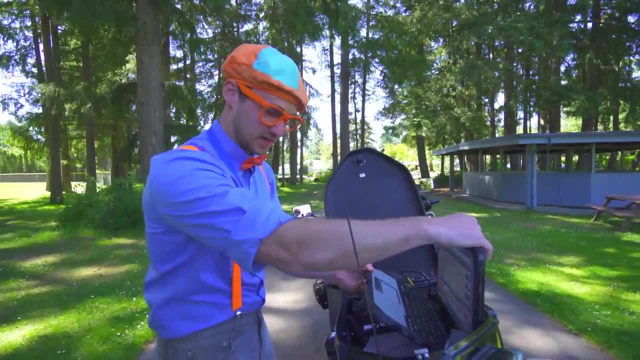 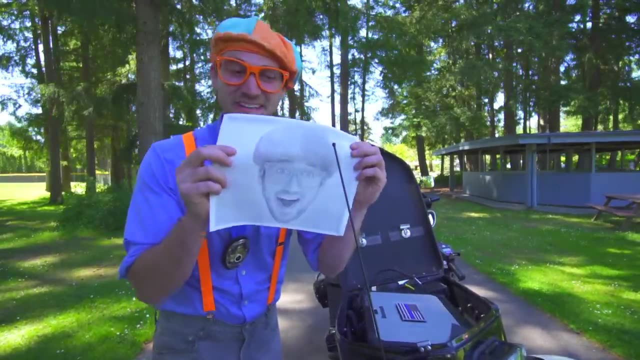 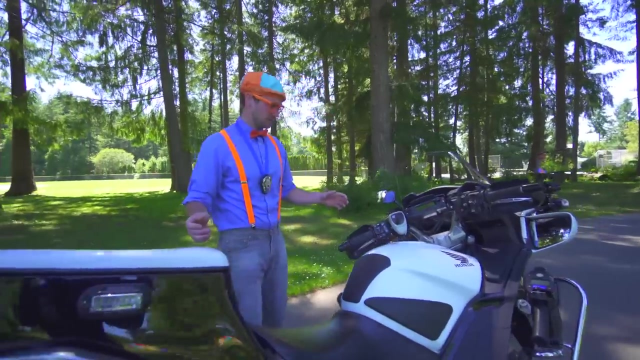 Okay, Now it's safe back here, Ooh, And back here. Here's a compartment, Okay, with a laptop. see, there's a laptop and a printer too. what is this? oh, it's a picture for me. oh, nice picture. okay, put that down right there. okay, so many cool. 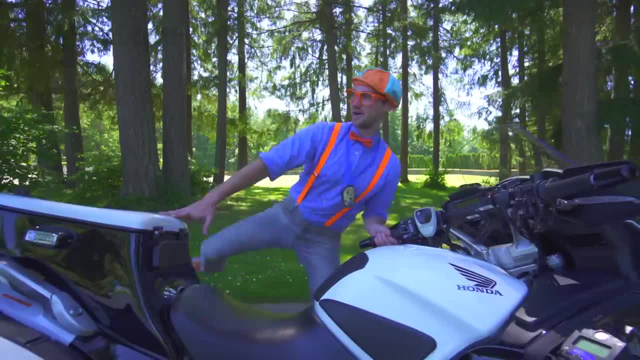 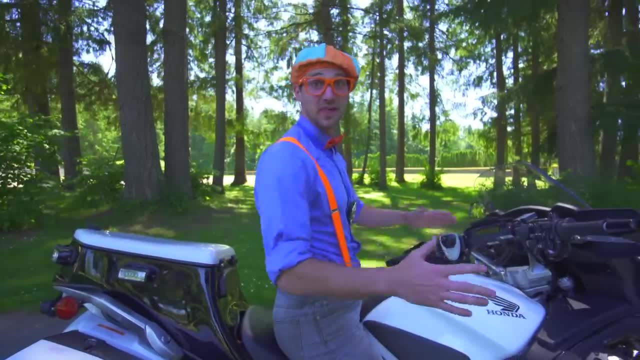 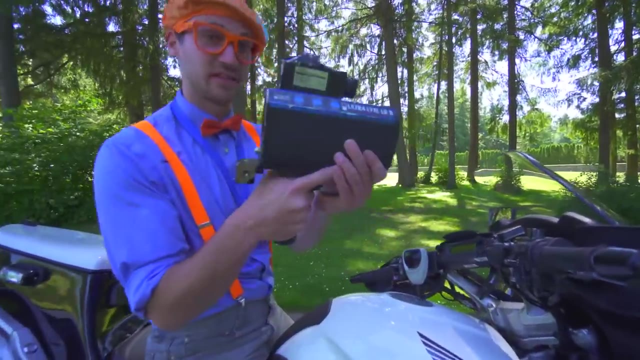 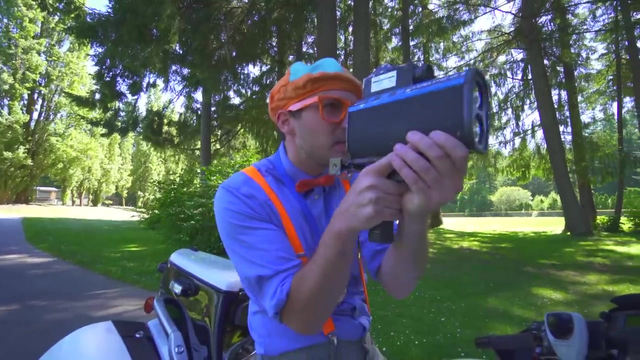 things to show you. but first maybe I should hop on. whoa, whoa, this motorcycle is really big, way bigger than the average motorcycle. okay, um, let me show you this. yeah, kind of want to show you this first. this is a radar gun. see, this is what's used to check the speed of everyone driving on the road. so you, 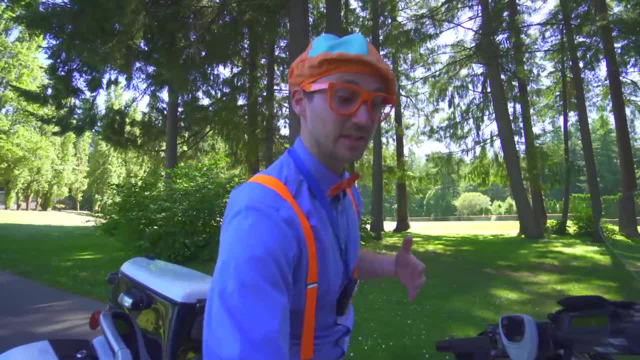 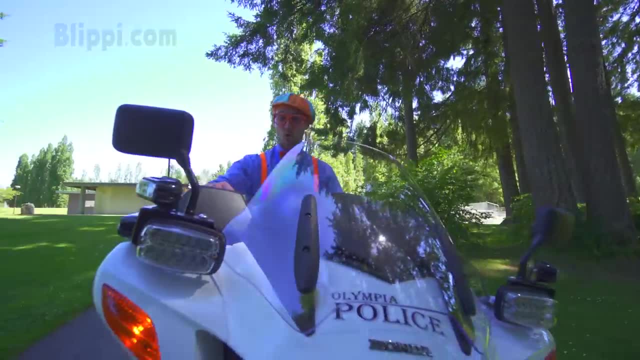 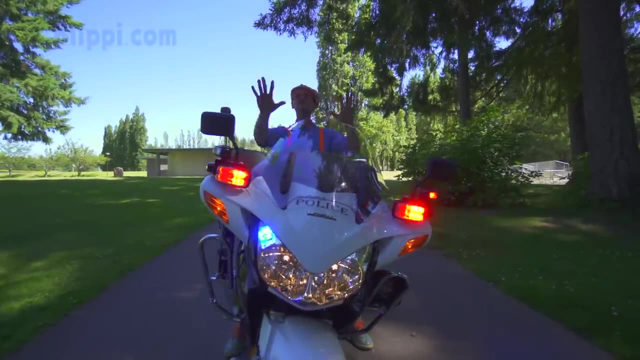 should drive the speed limit or lower, because that's the limit of safety. and let's see what else can I show you. oh yeah, the lights. watch this ready. oh yeah, red and blue lights. that's to let everyone know that there's an emergency. and what else is also used to let everyone know that. 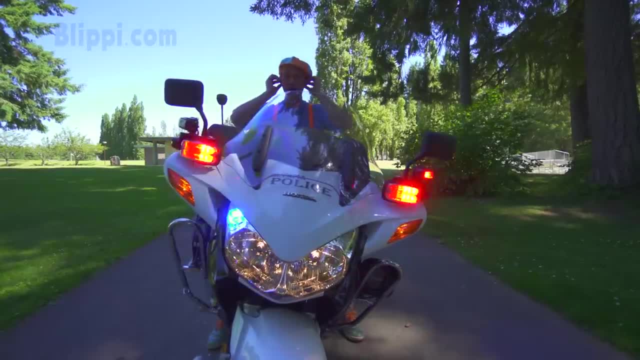 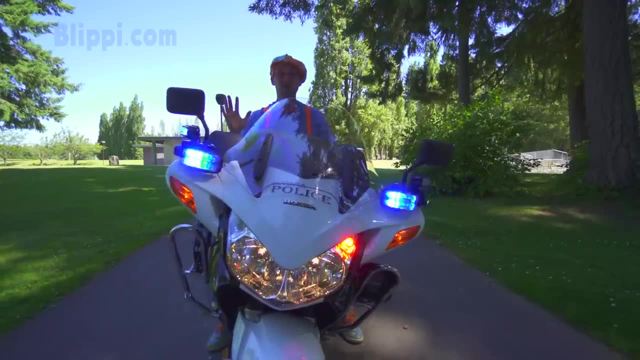 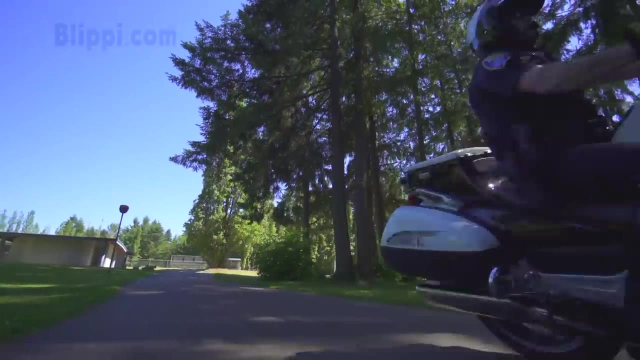 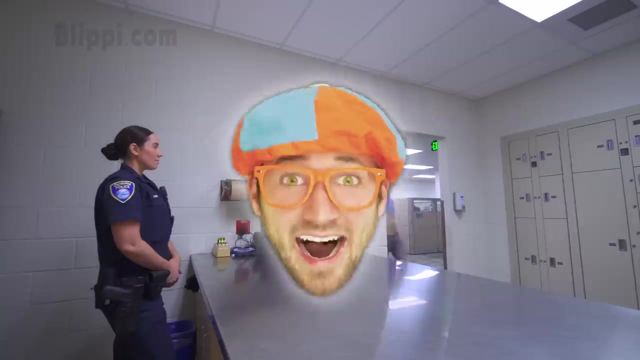 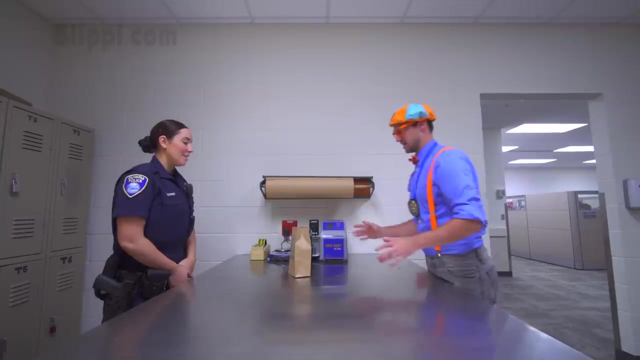 there's an emergency is the siren, and then also the horn, yeah, and then the police officer on the motorcycle took the evidence to the police station. whoa, look, we're inside the evidence room with our evidence. hey, how are you good? hey, that's the evidence. what do we do? so we're gonna process it for prints, okay? 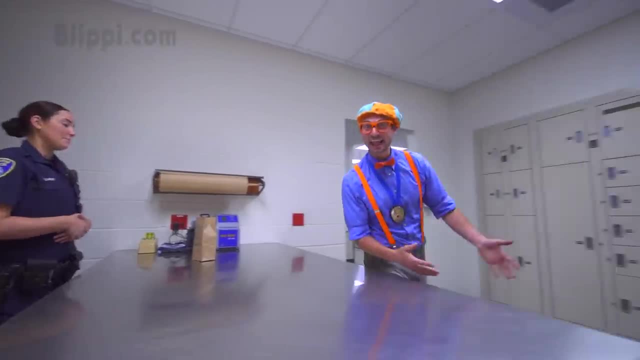 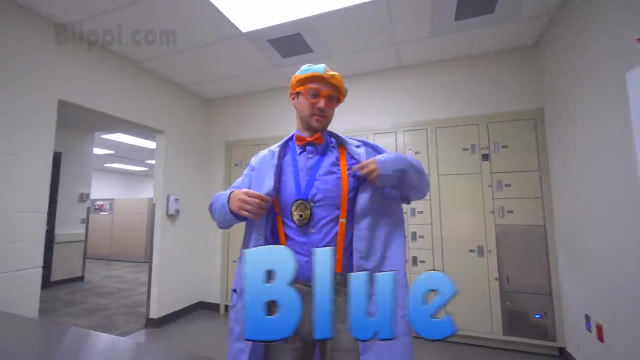 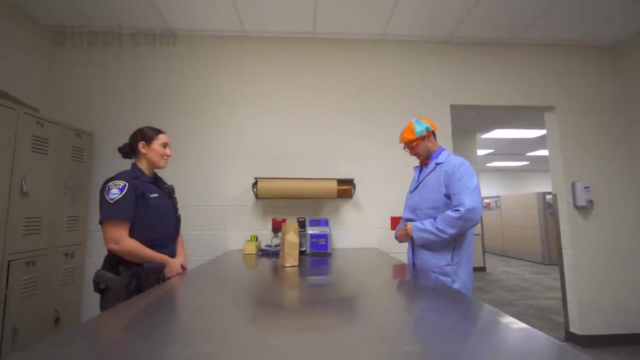 how do we do that? first, you're gonna need your lab coat. lab coat, look, yeah, it's the color blue. I like the color blue. it's one of my two favorite colors. blue is one of them and orange is the other. all, right, now, I have my lab coat on now. what? now you need your gloves. gloves, are they? 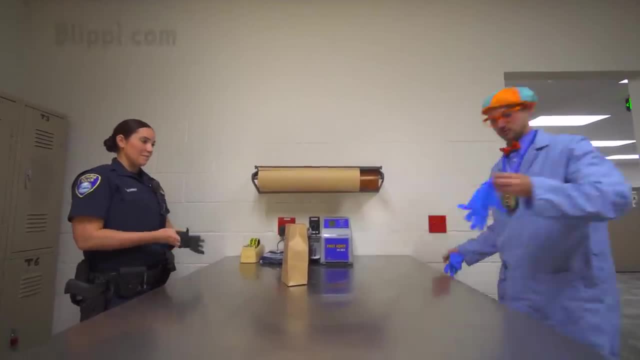 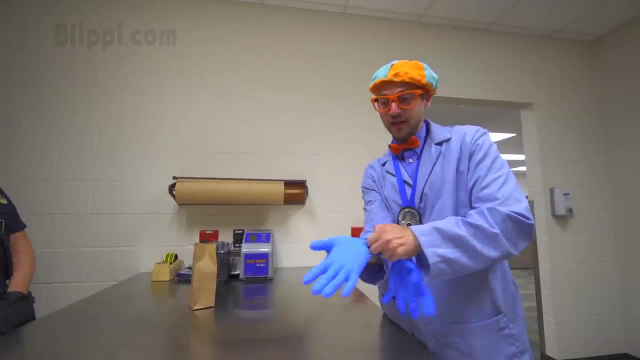 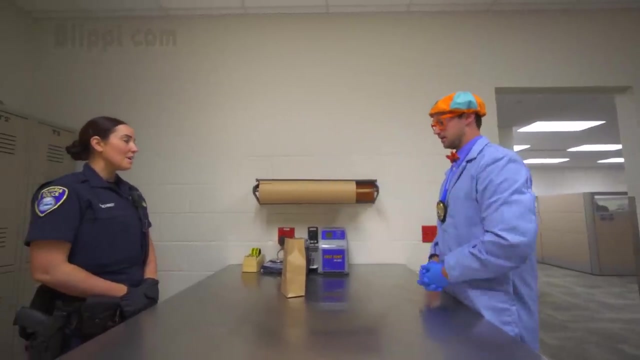 okay, they're right. here looks like: oh, look at these blue rubber gloves, so we wear these. so then we don't make our own fingerprints on the evidence. all right, so now I have the gloves on. now what? now you're gonna need to pull this brown paper down, okay, oh, here we go. thank you. 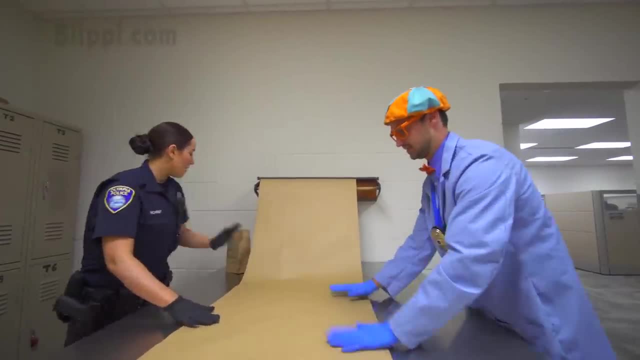 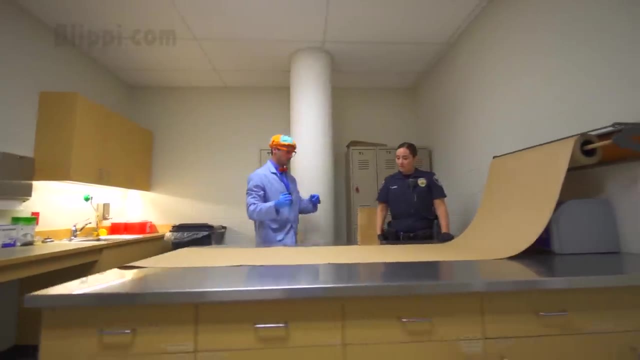 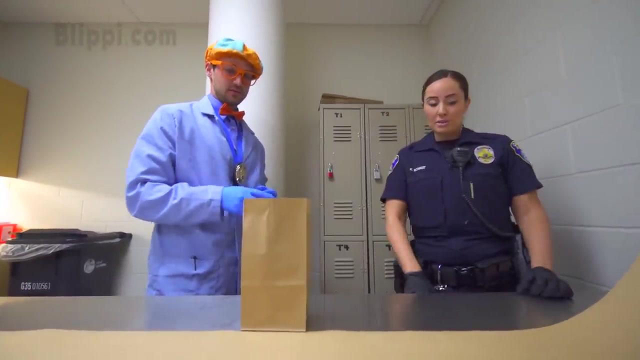 brown paper. okay, all right, now you can come on over to this side, all right, and now? so we have this. we have the paper right here and gloves on. so now, what do you need? now, you're gonna need some tools. okay, let's see. first of all, you're gonna need your paint dust. 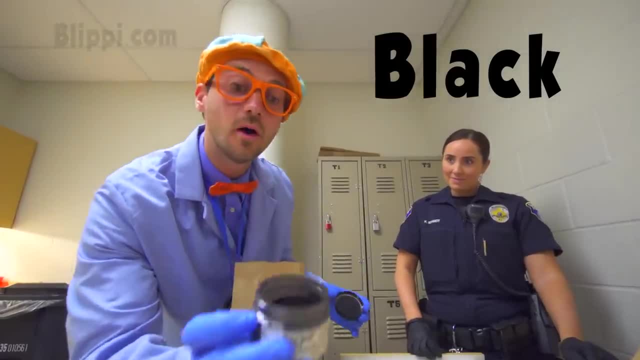 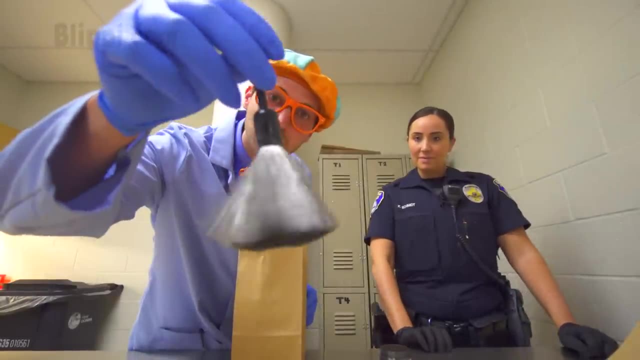 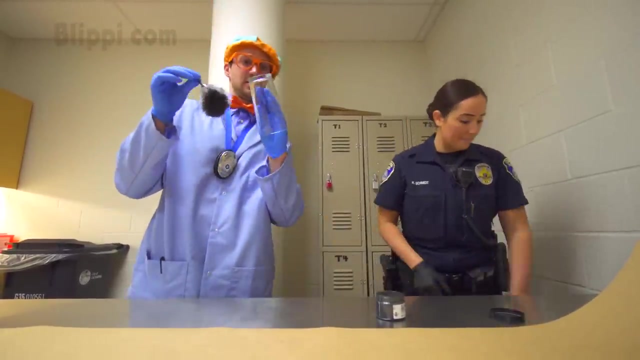 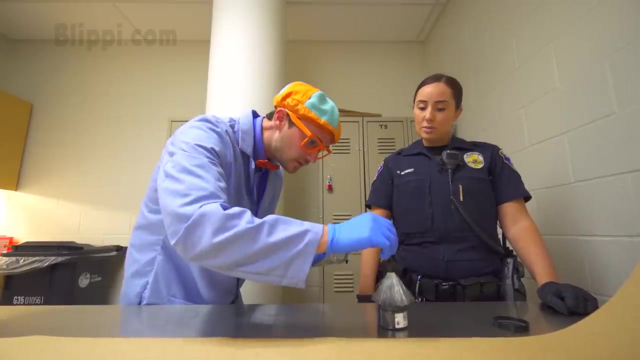 look at that print: dust, it's the color black, whoa. okay. next you're gonna need your brush brush. look at that brush- whoa. so now, what do I do? so take your glass out of the bag, okay, hey, okay. now dip your brush into the dust. okay, just a little bit. okay, I've got some dust. do you see that? now what? 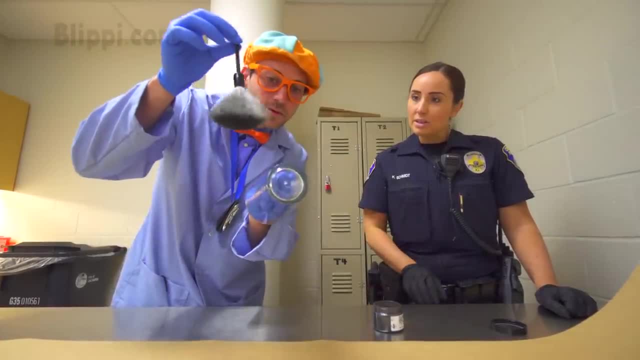 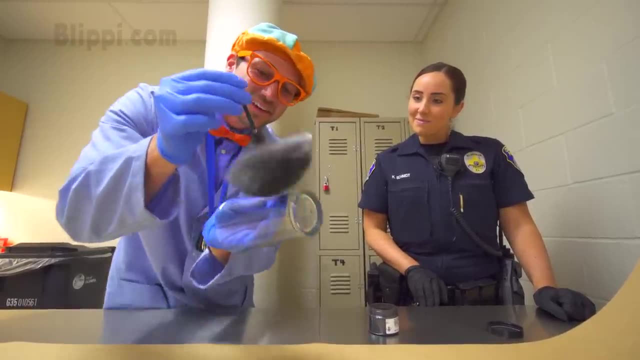 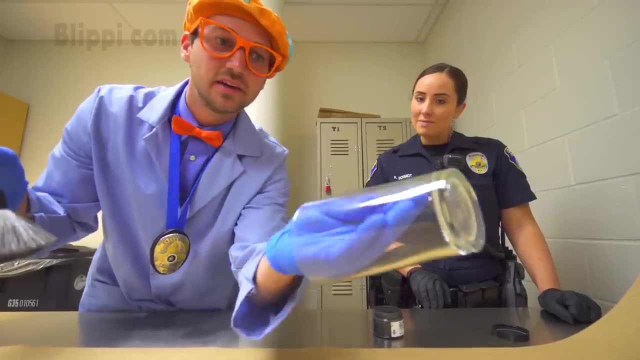 now paint your brush on your fingerprint like a fairy dancing on the leg. ooh, fairy dancing on the lake. I like that. you're funny. okay, here we go. all right, whoa, it's showing something. wow, all right. okay, I'll take that. okay, next you're gonna need your print winter print lifter. so a print. 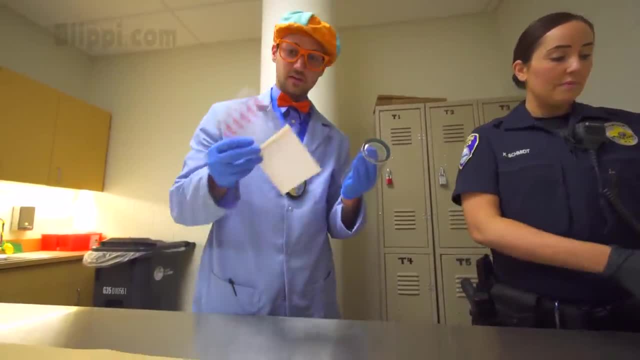 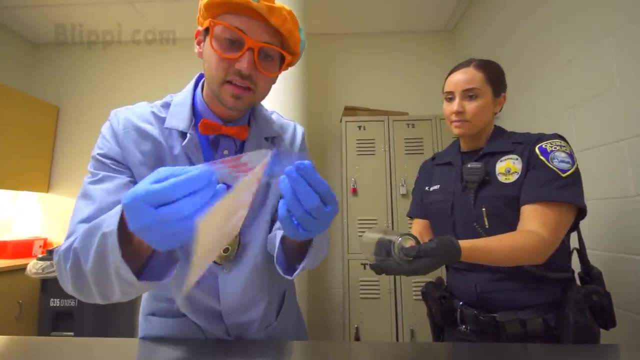 lifter. so a print lifter looks like a sticker. so I did have this. I just couple things like aすご Türk, a sticker. so can you hold this for me, sure, okay, so now i'm gonna unstick this, and this is really sticky, and then i'm gonna put it right here. 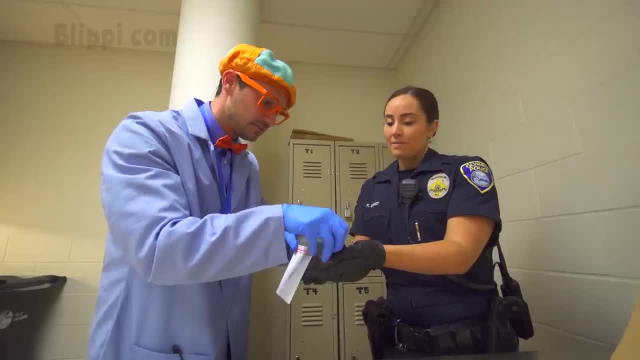 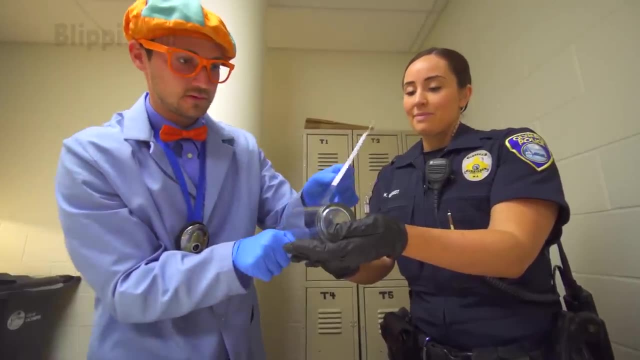 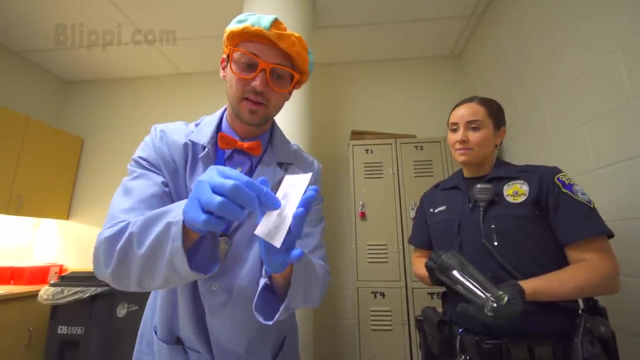 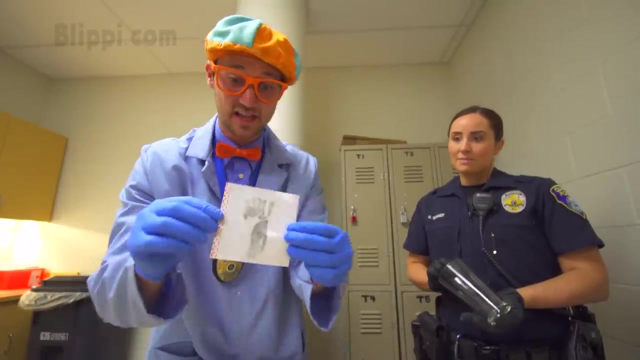 oh, there we go, oh, okay, and then should i peel it off? gently peel it off, okay, okay, just like that. oh, oh, we did it, wow, okay, let's close it up like a book and look at that. wow, we just pulled a print off of the glass. yeah, the evidence glass, okay. 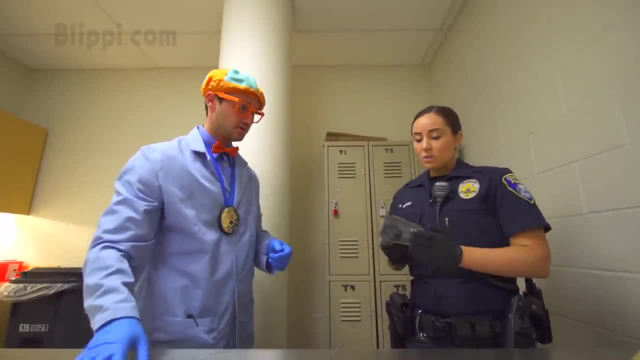 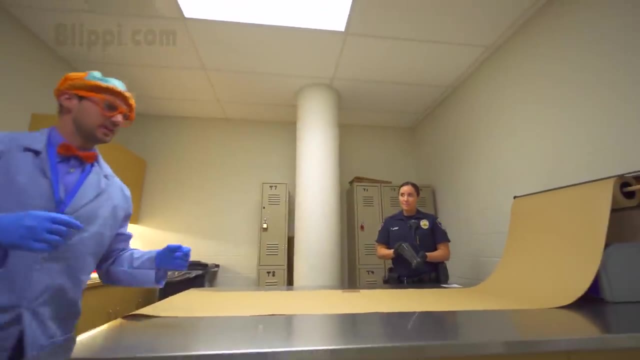 so i'll give you that. and then what do we do with the glass now? so the glass needs to go back into a paper bag, okay, so i'll go get a paper bag, okay, and yeah, here we go. oh, let's see, perfect, there's the paper bag. 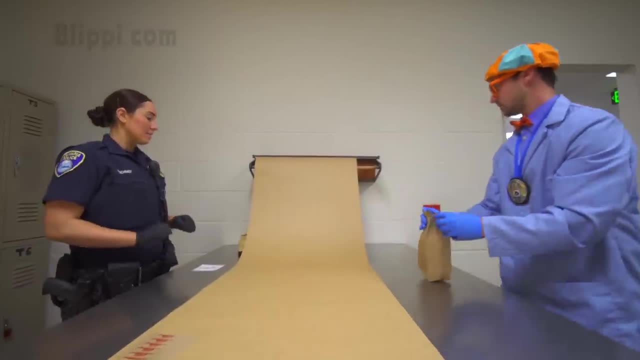 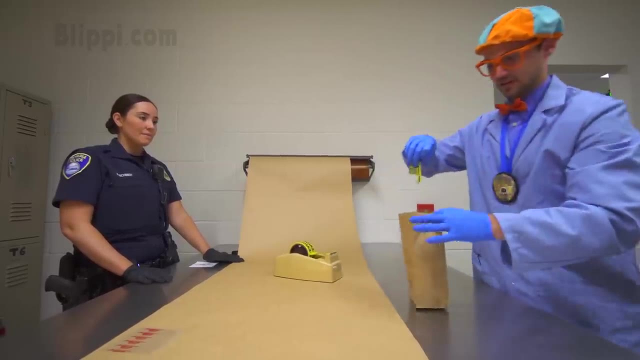 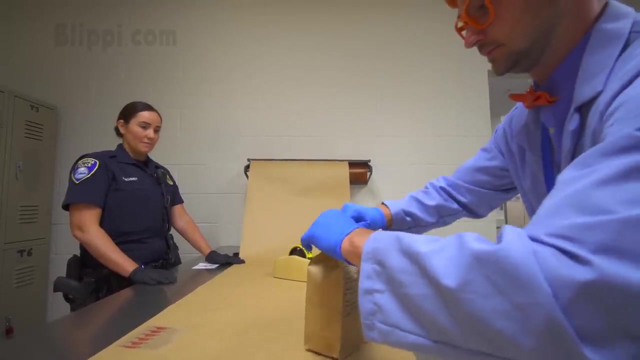 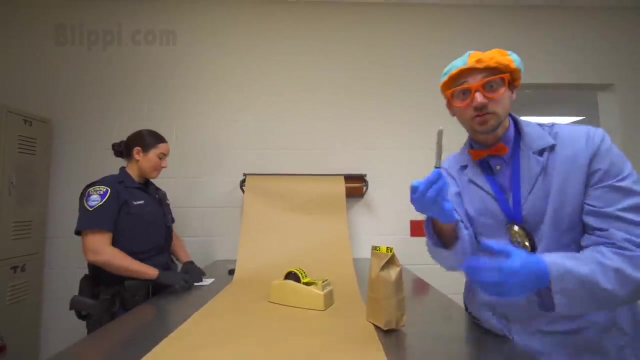 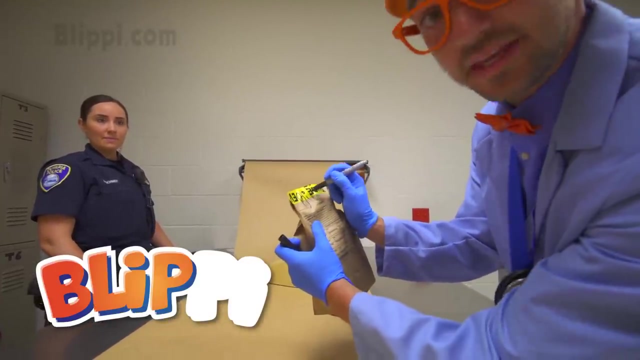 there we go. okay, now what? now you need to seal the bag with evidence tape. okay, evidence tape. oh, okay, check this out. evidence tape, seal it up. all right, it's nice and sealed. now what? don't forget to sign it. oh, to sign it. will you spell my name with me ready, b l i p p i blimpy. good job, all right.